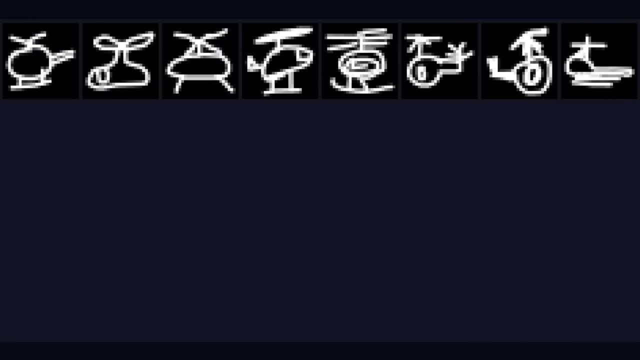 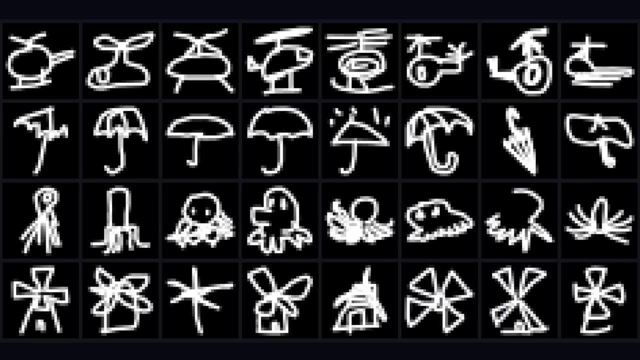 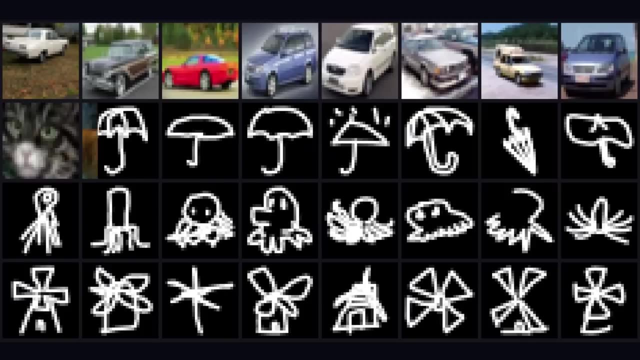 to recognise doodles of ten different objects such as helicopters, umbrellas, octopuses and windmills. Actually, we could even try one last thing after that, which is attempting to identify these little colour images, again of ten different things, this time from cars to cats and birds to boats. 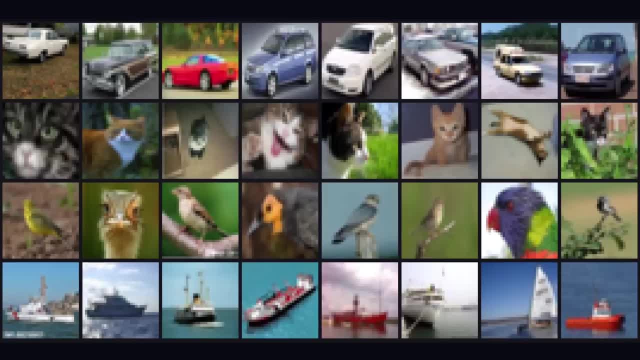 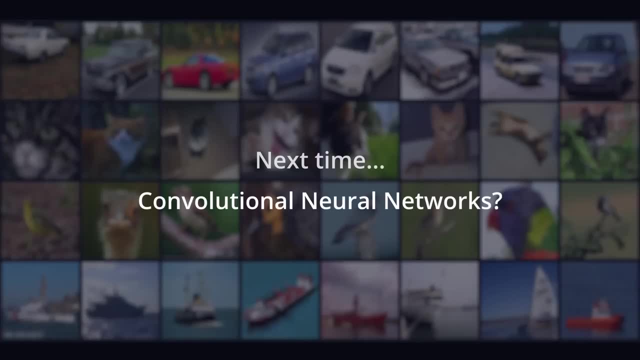 This is obviously quite a leap up in complexity, though, so if it proves too baffling for our simple network, then we'll have to return in the future to upgrade it to something like an original neural network, which is supposed to be much better at these kinds of problems. 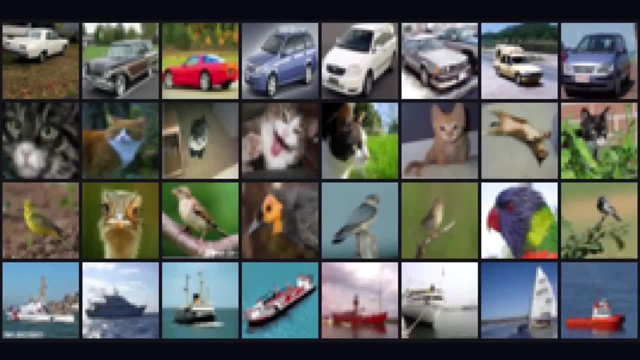 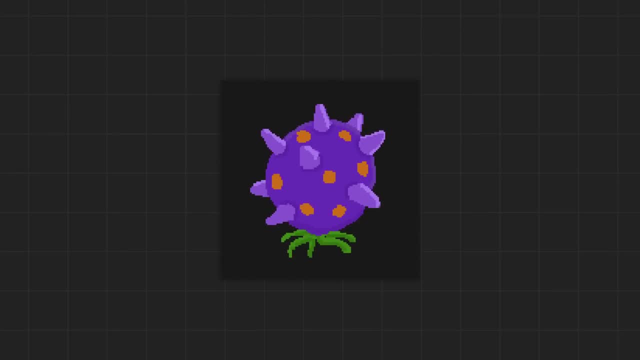 Anyway, to help figure out how we're going to build our neural network, let's imagine a simple example. We've discovered a peculiar new fruit which is purple and spiky with orange spots and extremely delicious. Strangely though, some of them seem to be poisonous, and will give you a 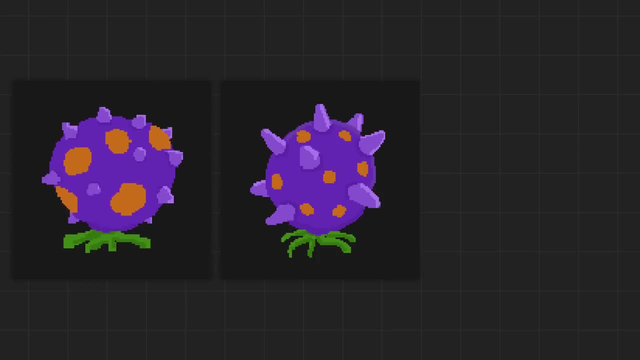 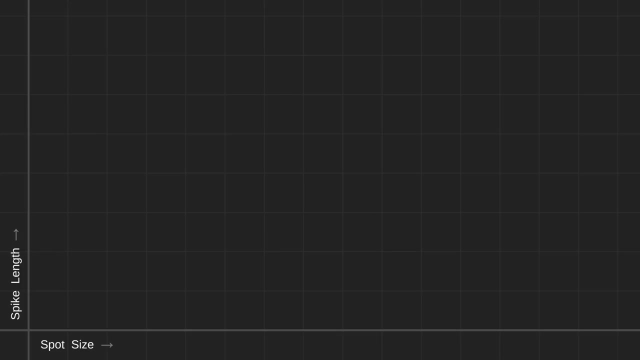 terrible stomach ache. So let's examine a few of these fictitious fruit and we can see that their size of their spots and the length of their spikes. We could try drawing a graph with the size of the spots on one axis and the length of the spikes on the other. Then we could collect a 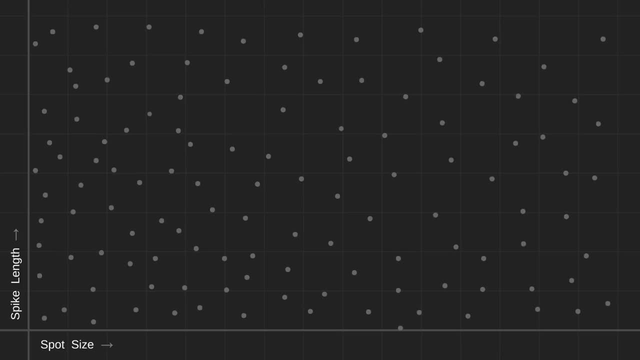 bunch of fruit and plot them all on this graph based on those attributes. With some brave volunteer fruit eaters, we'd label which were safe and which turned out to be poisonous. Now, if the result ended up looking kind of random like this, then the spots and spikes: 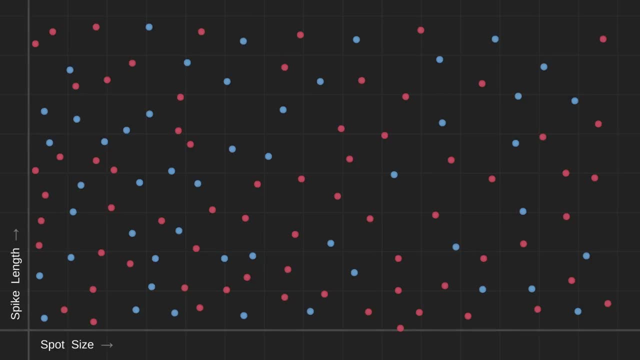 probably don't have much relationship with whether the fruit is poisonous or not, and we'd have to go back to the actual map and we'd have to think of something else. But if the data turned out looking more like this, then we're in business. We could draw a little line here called a decision boundary. 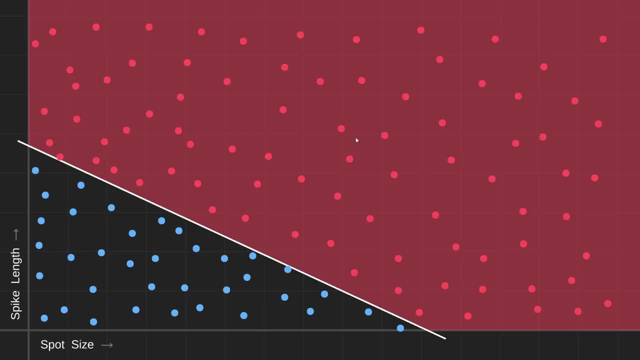 and say that any fruit we find that falls on this side of the boundary is probably poisonous and on the other side it's more likely that it's safe. So our very first step is to create a simple network capable of determining exactly that We have two inputs in our problem: the size of 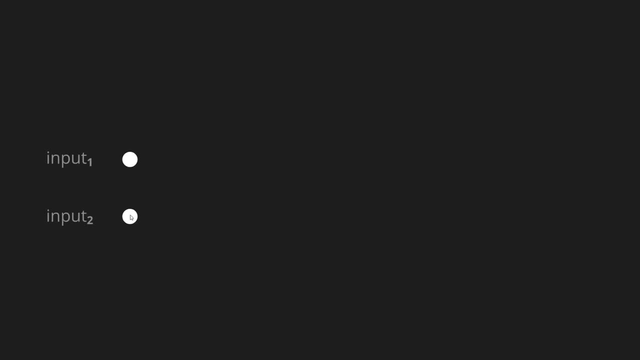 the spots and the length of the spikes, and there are also two possible outcomes: safe or poisonous. The way we'll interpret these is: if the first output has the highest value, then we're predicting that it's safe, but if the second output has the highest value, our prediction 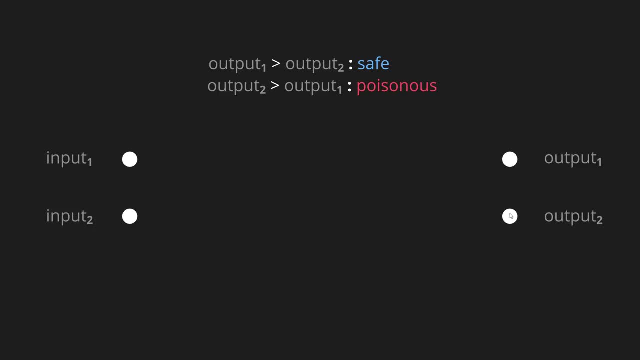 is that it's poisonous. Now you might be thinking: two outputs is quite extravagant. why not just have one and say: a positive value means safe and a negative value means poisonous? And we could definitely do that, but in future problems there'll be more than just two. 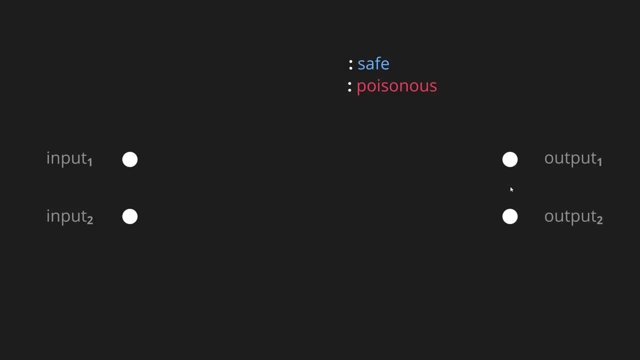 possibilities. We'll have to figure out which one is safe and which one isn't, and we'll have to think about the possible outcomes, so it's helpful to have a separate output for each of them. Alright, so these outputs obviously depend in some way on the inputs. 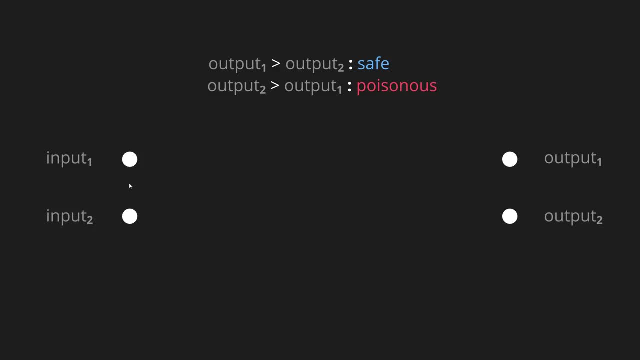 but we don't know how much of an effect each input should have. So let's connect both inputs up to the first output, and these connections each represent a weight for essentially how important the inputs are to that particular output. So the actual value of this first output will be equal to the first input multiplied by the weight. 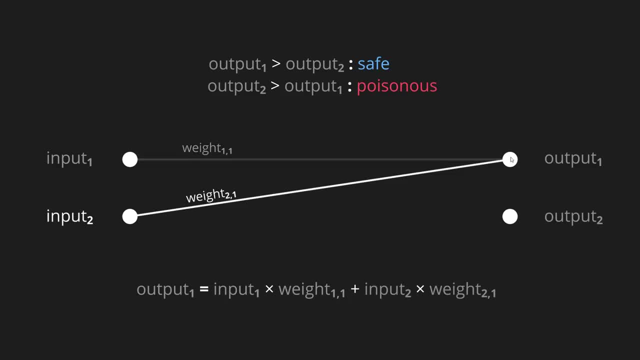 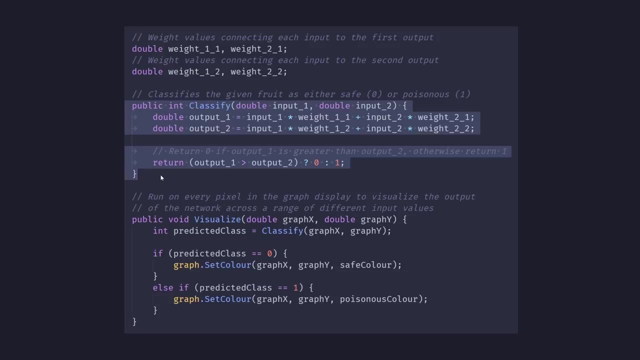 of its connection, plus the second input multiplied by the weight of its connection. I've quickly written up some code to perform this calculation, which you can see in the classify function over here. Then, to visualise what's going on, there's this visualise function which gets run for every pixel. 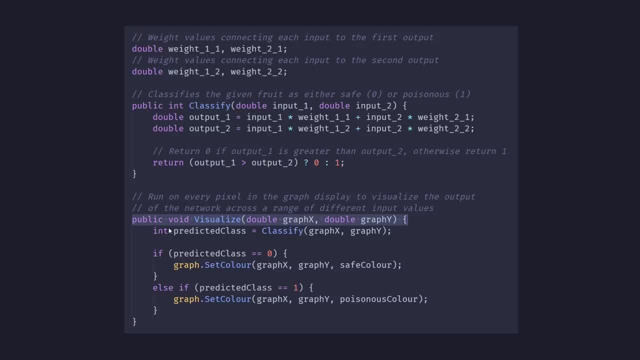 in the graph display and it asks the network to predict whether a fruit at that point would be considered safe or poisonous and then colours the data to predict the fruit at that point the graph accordingly. So let's see what this does. At the moment it's very paranoid and seems. 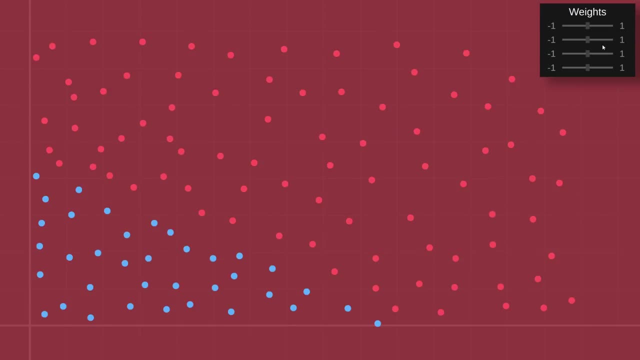 to think everything is poisonous. but up in the corner here we have our network weights, so I'll play around with these a bit to see if I can get that decision boundary how we want it. Unfortunately, no matter what I do, I can only get the boundary to essentially rotate around. 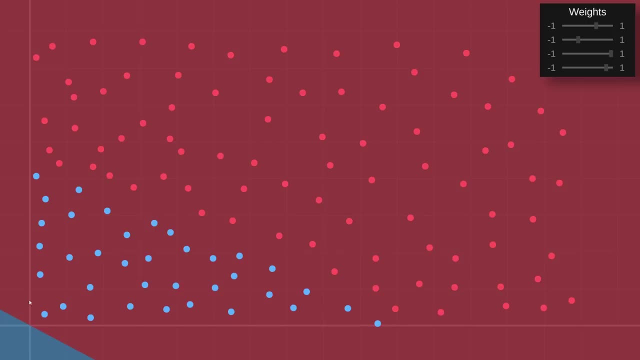 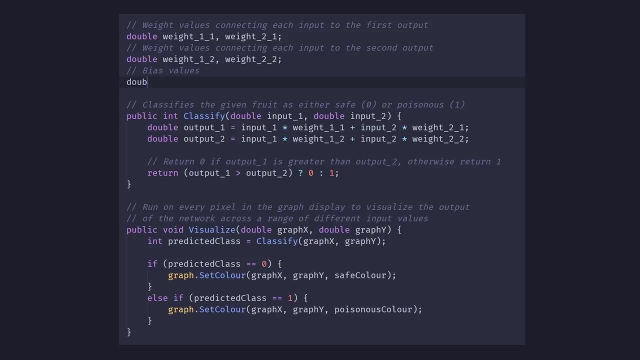 the origin of the graph here, when what we need now is to be able to shift it vertically. So let's go back to the code and make a tiny upgrade to our network by adding in two new values called bias1 and bias2, and these will simply be added onto our weighted inputs over. 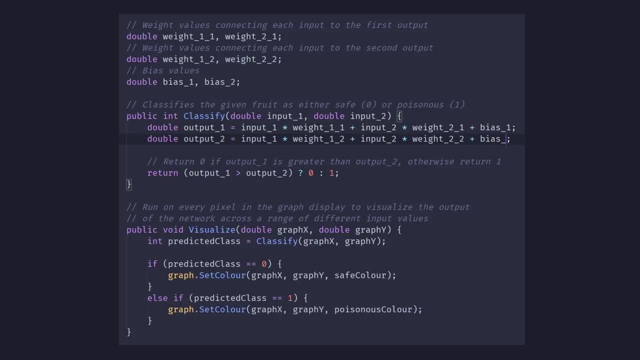 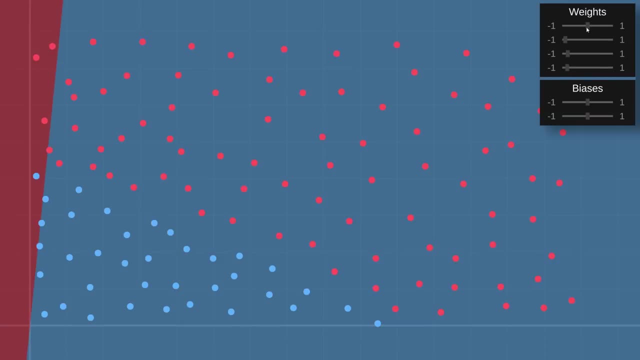 here, allowing us to move those values up or down. Okay, let's give it another shot. so I'll fiddle with the weights again to try to get the angle of the boundary correct and then I'll move on to the biases. It's a bit finicky to control, but with some patient. 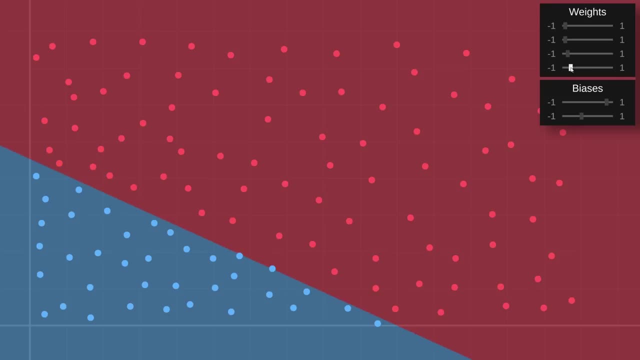 tweaking, we should eventually be able to hand train our code. This was a pretty straightforward task, though, so let's imagine that when we collected this fruit data, it actually ended up looking something like this: This is trickier, of course, because we can no longer separate safe from poisonous with a straight line, so we'll need to make 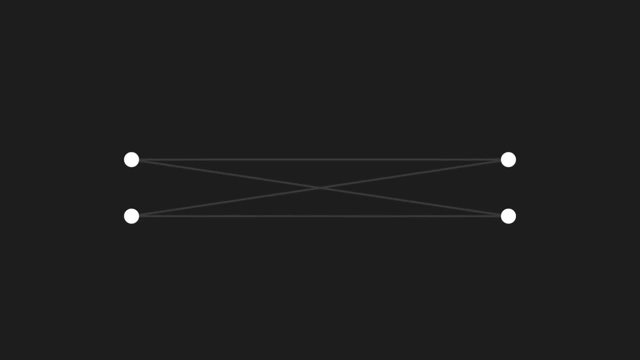 some more upgrades to our network. One way we could try to improve the network is simply by making it bigger. It doesn't make sense to change the number of inputs and outputs in our network, but we can do it and in this case that's correct. So if we add a number, 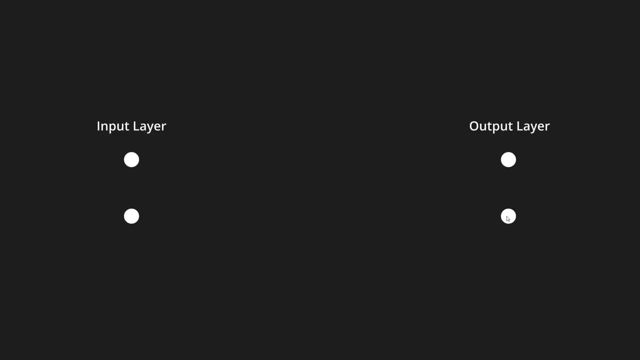 inputs, because those are determined by the problem we're trying to solve, but instead we can create a new layer that sits in between. These in-between layers are known as hidden layers, for whatever reason, and they can have as many nodes as we like, and we could even have multiple hidden layers, but let's keep. 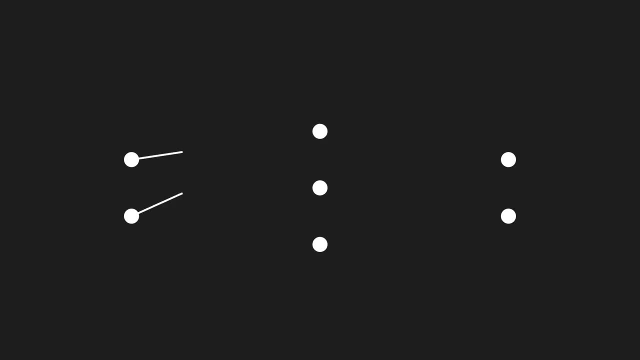 things simple for now. So as our input values get fed forward to the next layer, they'll be multiplied by their weights, as we've seen before, and added up with a bias value, together creating a weighted input for that node. And once that's been computed for all the nodes in the middle layer, those values can 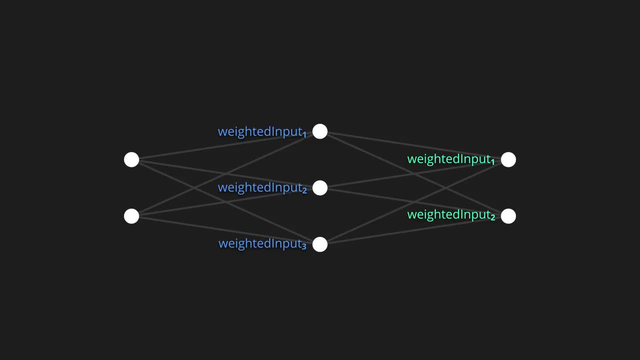 then be fed forward in the same way to form the weighted inputs of the next layer. Even for this extremely tiny network with only 12 weights and 5 biases, it would be quite tedious to write out all the calculations by hand, like I did over here, so I'm going. 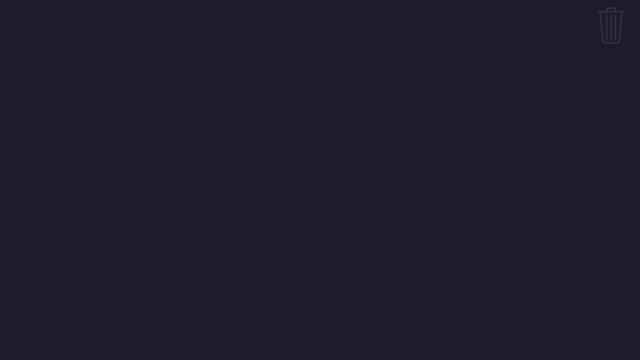 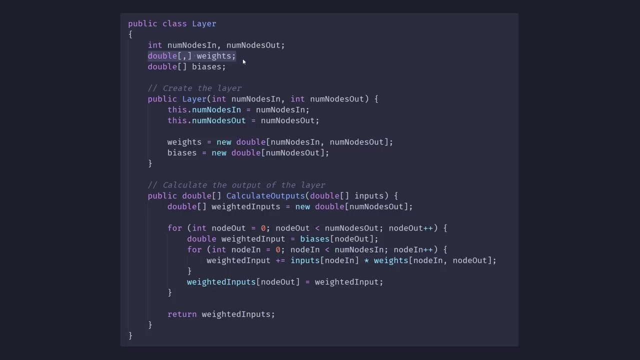 to throw all of this code out and start working on a more sensible solution. So I've begun by making a layer script which stores the weight values for all the incoming connections, Along with bias values for each node in the layer, and these get set up over here based. 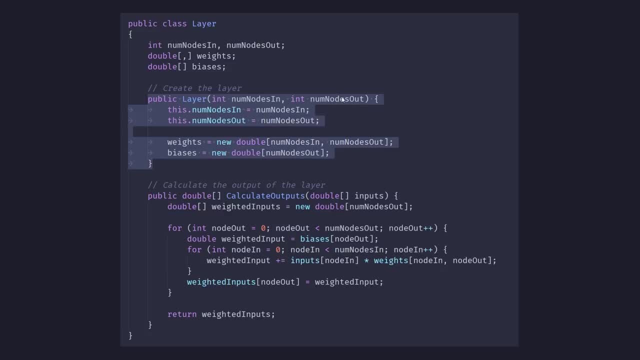 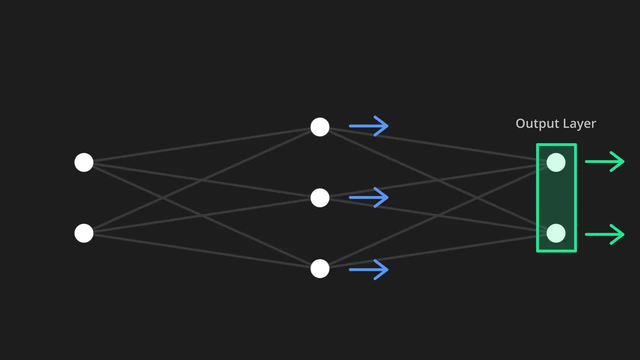 on the number of incoming and outgoing nodes. Just to clarify in the code I'm thinking of this layer, for example, as having 3 incoming nodes and 2 outgoing nodes. Then this layer would have 2 incoming nodes and 3 outgoing nodes. 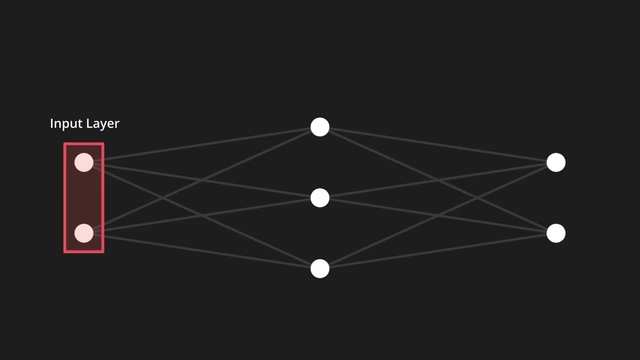 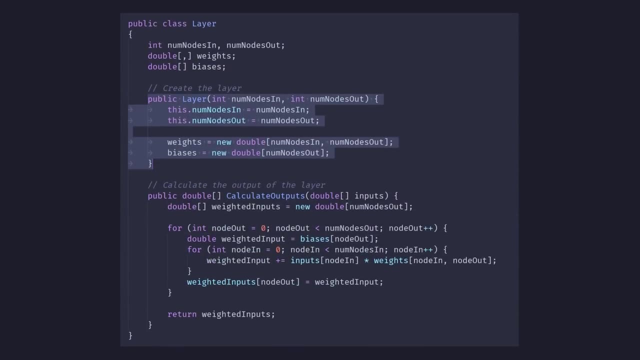 And finally, this layer really just represents the values given to our network. it doesn't do anything, so it's not going to be an actual layer in the code. Alright, back to the layer script. all that's left to look at in here is this: calculate: 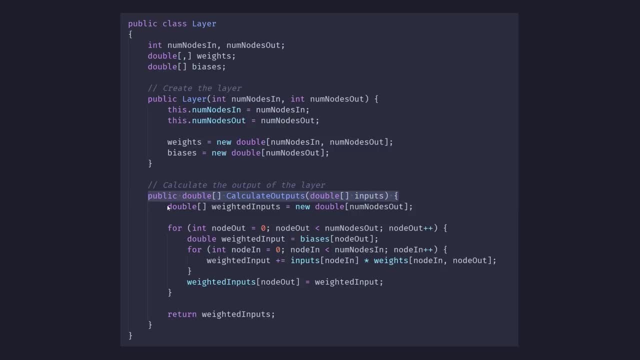 output function which takes in some input values and computes the weighted inputs simply by looping over each outgoing node, setting the corresponding weighted input to that node's bias value and then looping over all the incoming values, multiplying each of those by the weight of their connection and adding the result onto the current weighted. 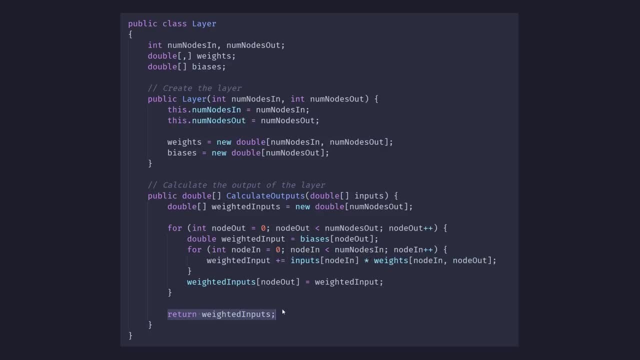 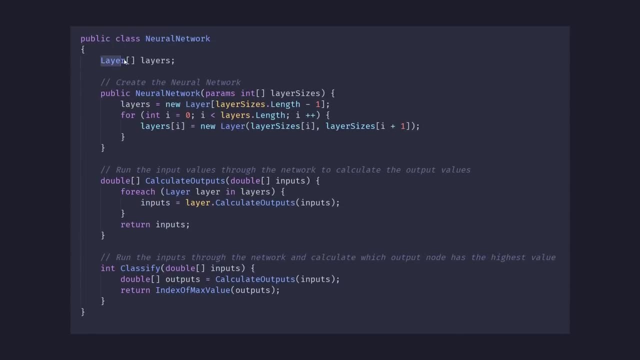 input- For now at least, these weighted inputs are then returned as the output. Next we have the actual neural network class, which contains an array of these layers. So when a network is created, it needs to be told how many nodes there should be in. 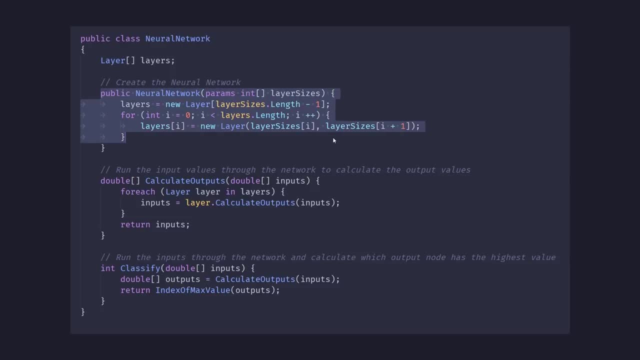 each layer and it uses that information to set them all up like so. Now, over here is the function for calculating the output of the entire network, and all this does is loop through all the layers, calculating the output of each layer, and 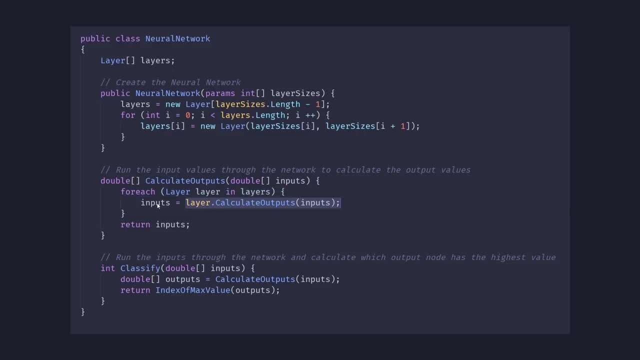 using that as the input to the next layer. Finally, the classify function works essentially the same as before. it just calculates the output values and returns the index of whichever value is largest. So I'll create a network with three layers now, which will give us a lot more parameters. 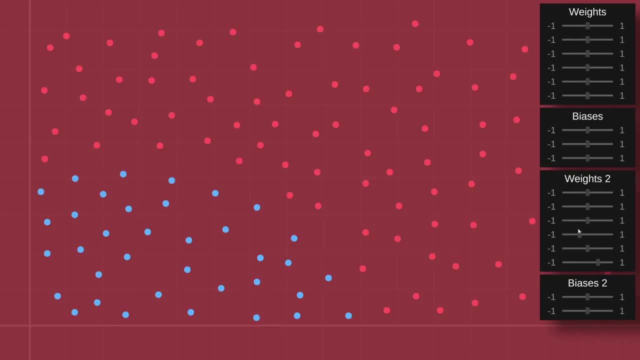 to play with and let's see what new and exciting things we can do. Well, it turns out adding an extra layer doesn't help at all, At least not on its own- To make this boundary bend. we're going to need to allow the layers to have a non-linear 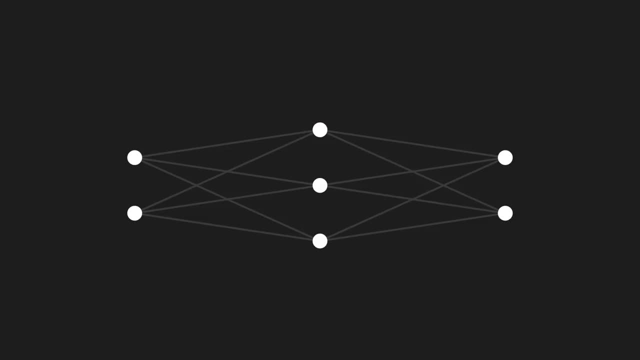 effect on the output. So let's go back to our design and zoom in on a single node. In a loose analogy to biological neural networks, we can think of this node as a neuron and the weighted input over here as some sort of stimulus. 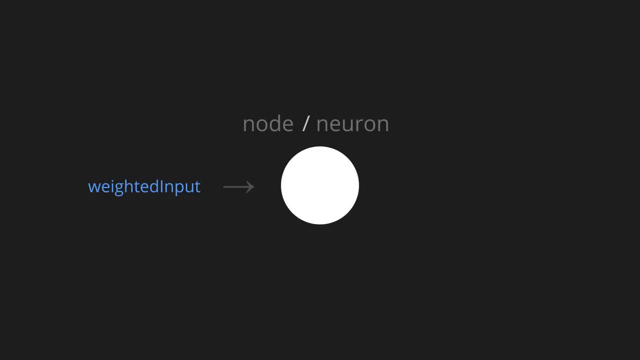 If the stimulus is sufficiently stimulating, that should cause the neuron to fire, which in our model could mean outputting a value of one, whereas if the stimulus is small, the neuron wouldn't fire, so we'd just be outputting zero. I'll refer to this output as the activation value, so we just need to write a little function. 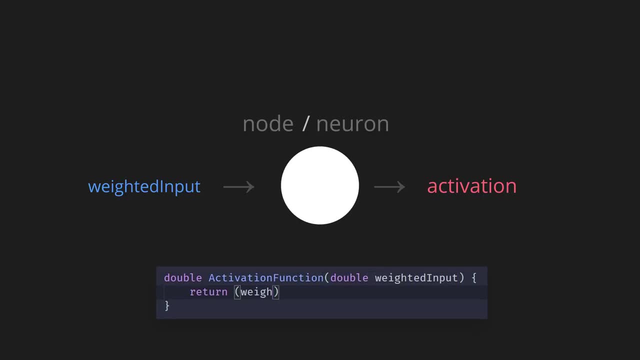 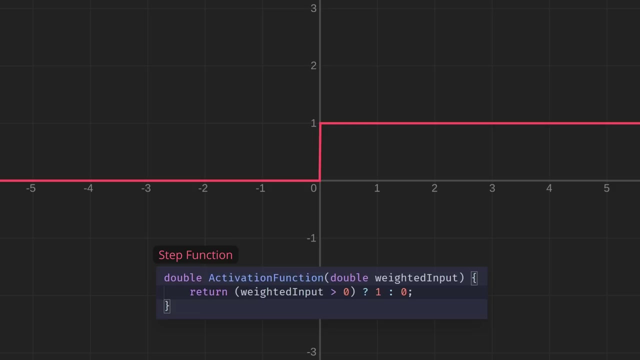 that takes in the weighted input and computes that activation value, Something like this. And let's quickly visualize that with a graph. So the x-axis here shows the weighted input and the y-axis shows the corresponding activation value. Using an activation function like this should allow us to have more complex decision bombs. 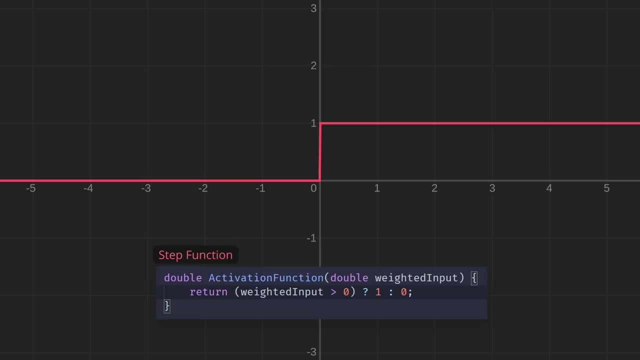 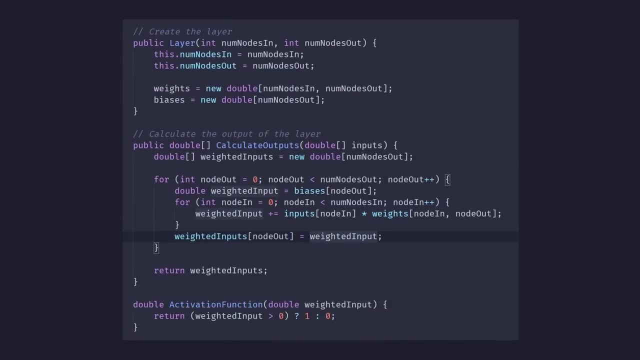 So let's go ahead and do that. Let's do that. Before we can try it out, though, we'll need to quickly jump into the layer script and, instead of outputting the weighted inputs over here, let's pass them through the activation. 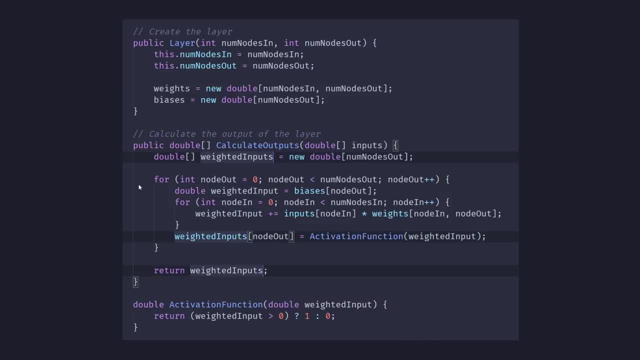 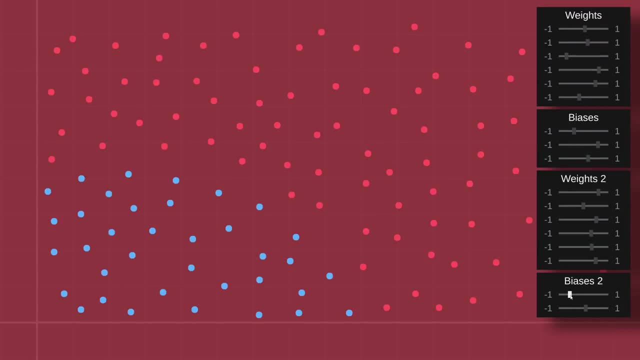 function and then output those activation values instead. So returning to the joyful process of randomly tweaking sliders until something happens, we can at last see that we're able to actually make simple shapes with the decision boundary. And, of course, increasing the size of the network now would allow us to make increasingly. 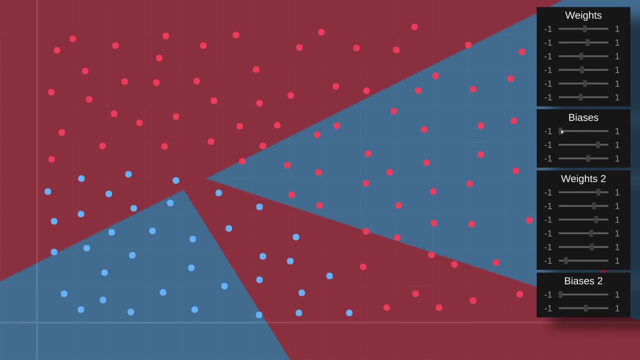 fancy shapes, But this tiny network is already sufficient to correctly classify the made-up data we have at the moment. By the way, you might have noticed that the biases no longer simply shift the whole boundary up or down, like they did before. instead, they're just a way of easily shifting the 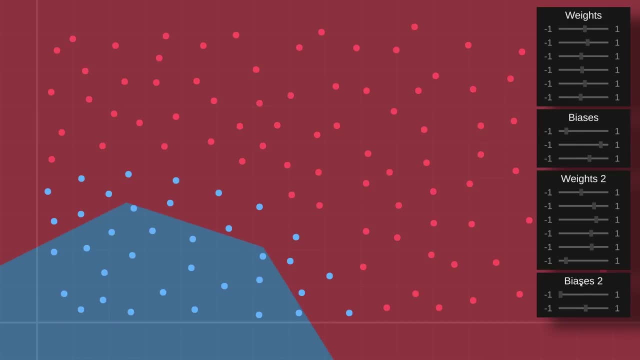 value that goes into the activation function. So, thinking of our biological analogy, it would be like a threshold that the stimulus needs to exceed in order for a particular neuron to exist. So let's go ahead and do that Now. one thing I don't like about our current setup is how abruptly and dramatically the 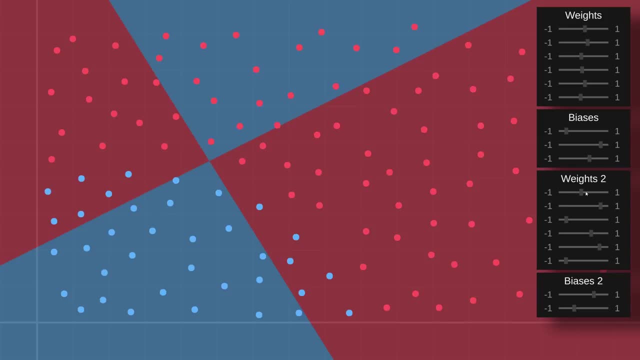 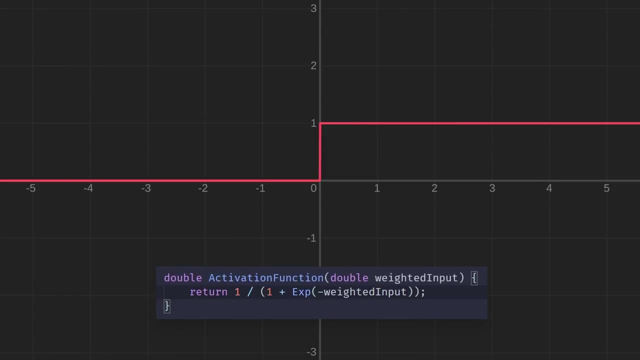 output can change in response to just a tiny tweak to some of these sliders. So let's go back to our choice of activation function and maybe replace it with something like this instead, which simply smooths things out. This is called a sigmoid function, by the way, and it's just one of many different functions. 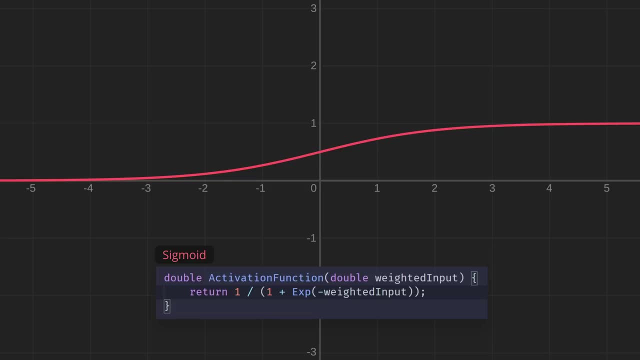 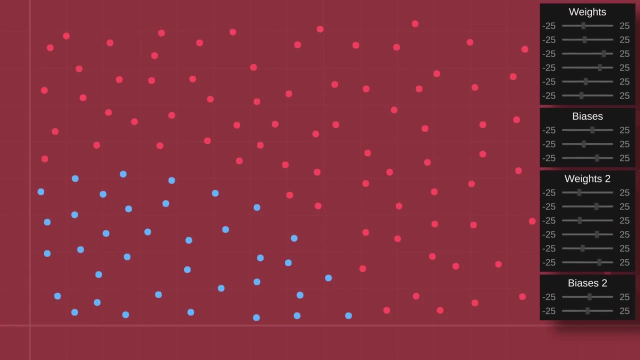 that people have experimented with for neural networks. Here's a few others just as a matter of interest. Anyway, let's go with this one for now and see how that affects things. So I'll mess around with these sliders once again and we're now able to make nice smooth. 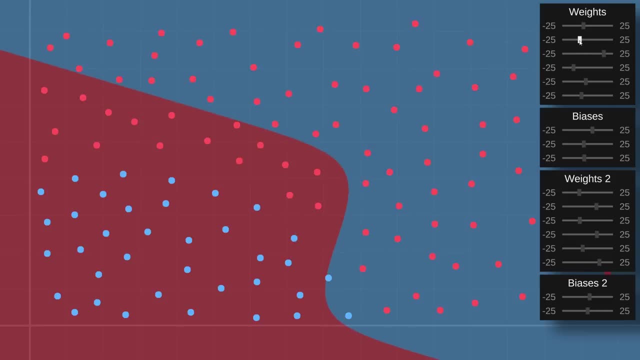 boundaries and, more importantly, making small changes to any of the sliders will no longer result in a drastic change to the output. Anyway, as fun as it is trying endlessly to train this network by hand, the goal, of course, is for the computer to do it all by itself. 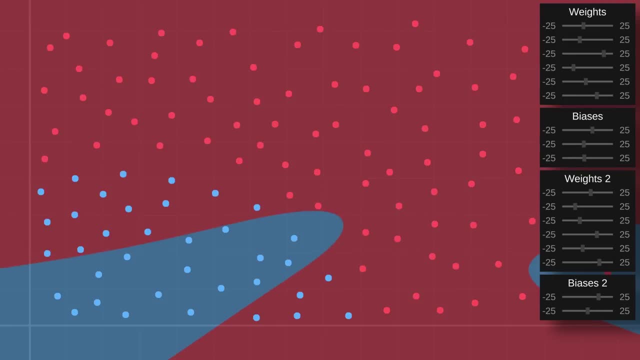 And for that to work, it's going to need a way to measure how well it's doing. One approach would be to simply count the number of known data points that are being classified correctly, But the trouble with that approach is that often making a small adjustment to one of 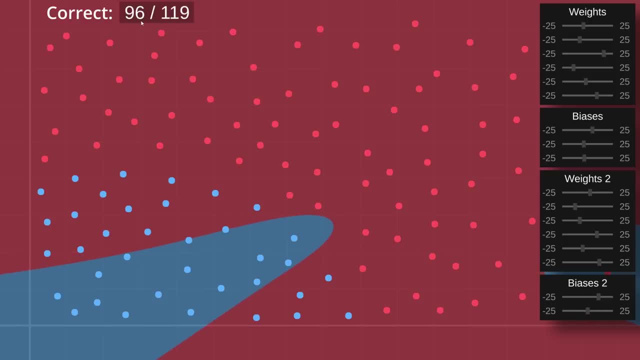 the sliders won't actually change that number, meaning it's impossible for the computer to know if that adjustment was beneficial or not. So we should try to find a more precise way of measuring progress. Let's look at the outputs of our network again, which are now being squished to somewhere. 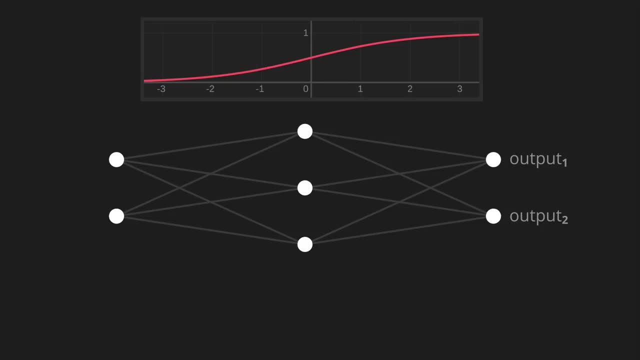 between 0 and 1 by our sigmoid activation function. So if we give the network the inputs of a fruit that's safe to eat, we'd hope to see a 1 at the first output and a 0 at the second output, representing total confidence. 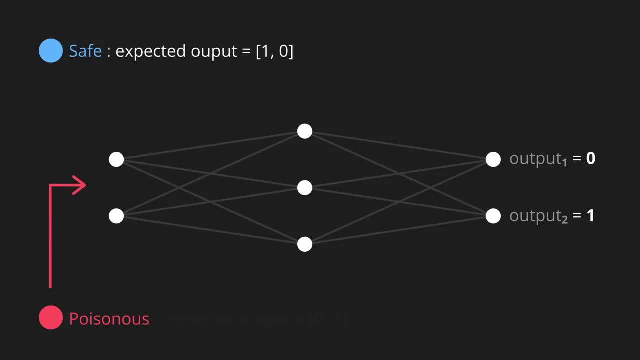 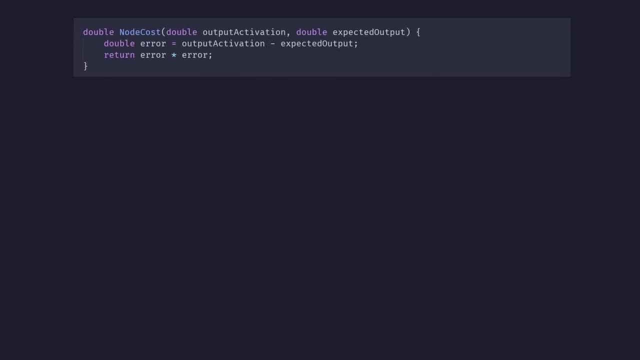 that it's safe, And for a poisonous fruit that should be the other way around. So since we know what the outputs should be for our training data, I've added a little function to the layer script, called the nodecast, Which takes in the output activation value of a single node along with the value we 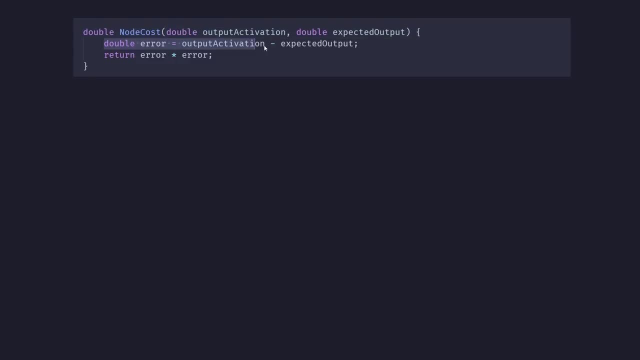 want it to be. All it does is calculate the difference between the two and square the result. Just to make it positive and, I guess, to emphasise large differences as being much more urgent to correct than small differences, Then in the neural network script I've added a function simply called cost, which takes 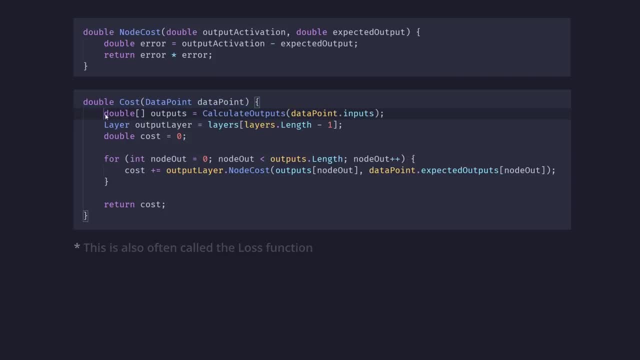 in a single data point, such as one of our fruit, and runs its inputs through the network to get the output values Using those. it then adds up the individual costs of all of the nodes in the output layer to get an overall cost, telling us how badly the network is doing for the given data point. 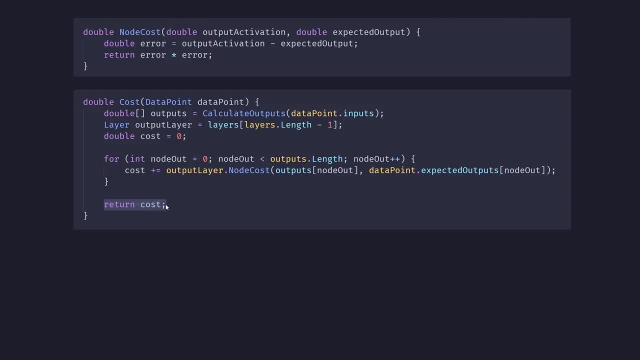 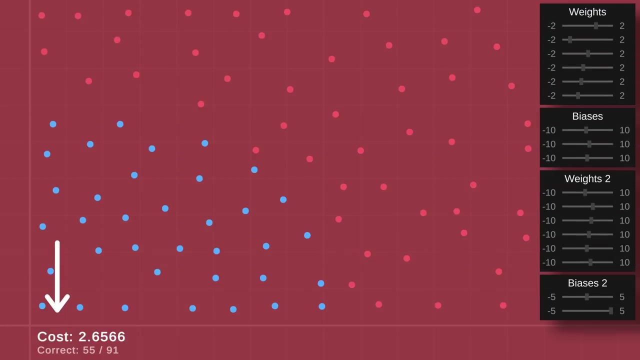 We're most interested, though, in how the network is doing across all our data points, so here's another version of the cost function, which takes in multiple data points this time and just adds up each of their costs and returns the average. So you can see that value at the bottom of the screen, and the goal of the network is. 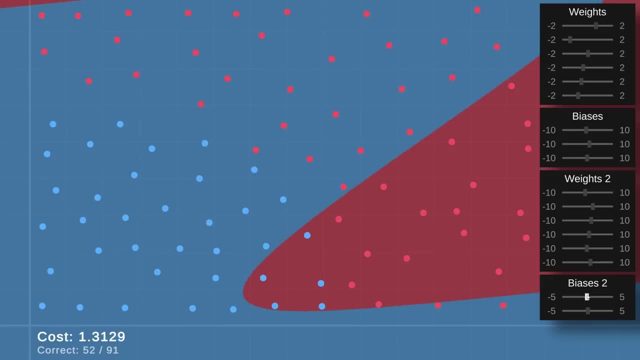 for its 17 weights and biases here, which result in the smallest average cost For the tiny network we have here. we could probably even get away with a brute force trial and error approach, but our networks are going to get a lot bigger as we tackle. 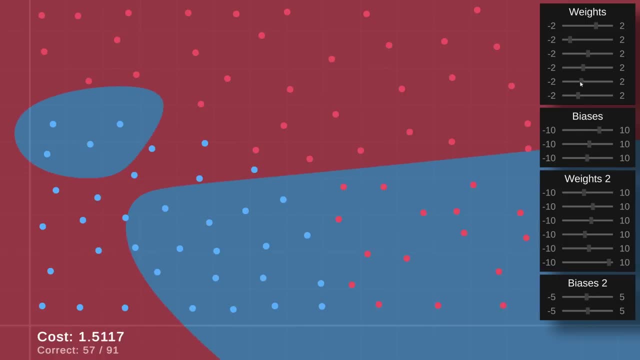 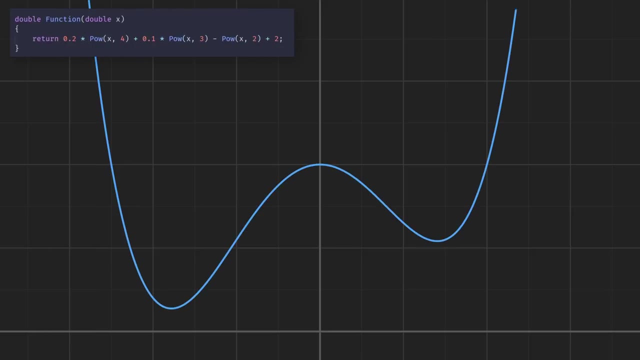 trickier problems, so we should definitely try to find a better solution. Let's simplify things by thinking first about this little example function where, similar to the task of finding the weights and biases that minimise the cost function, we want the computer to find the input values. 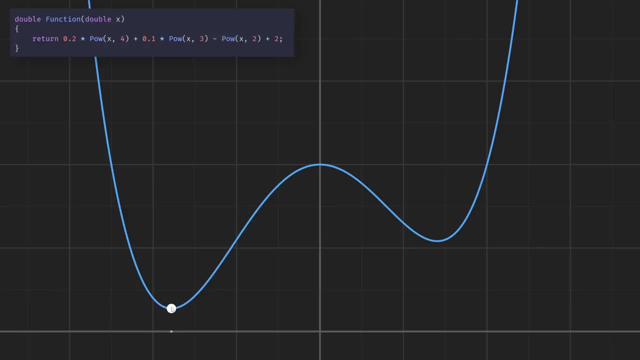 And, of course, we'd like it to do this in as few steps as possible, not just calling the function millions of times until it finds a good answer. Now our solution is going to rely on calculating the slope of the function, so let's try writing. 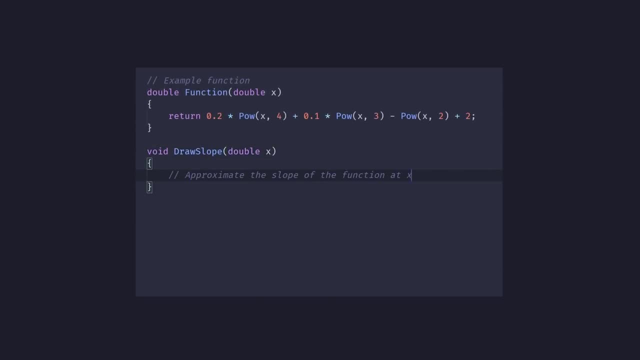 some code to visualise it. We can approximate the slope very easily by first defining some tiny value, which I'll just call h, and then calculating how the output of the function changes. The steepness of the slope will just be this change to the output divided by the change. 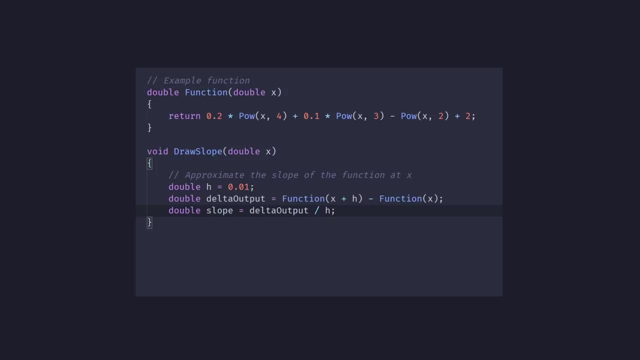 to the input that caused it. So, as I said, this is just an approximation, because we're technically calculating the slope between two points on the graph, but the smaller we make h, the closer our approximation will be to what the true slope would be, precisely at the given input value. 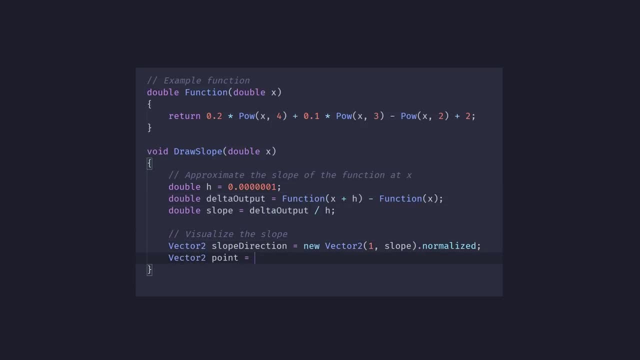 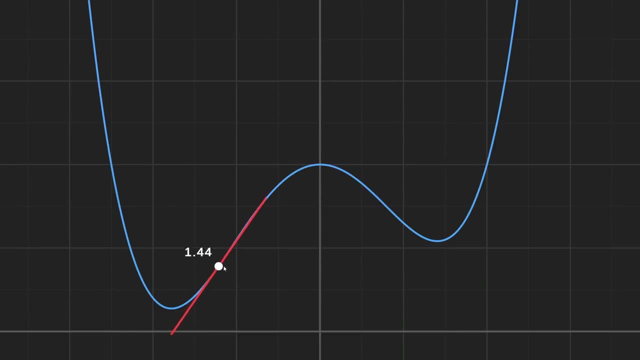 Anyway, we can then visualise the slope with a bit of code like this: Let's see how that looks. So the slope value is pretty intuitive. we can see, for example, that it's negative over here because the function is decreasing as the input increases, but it's getting closer. 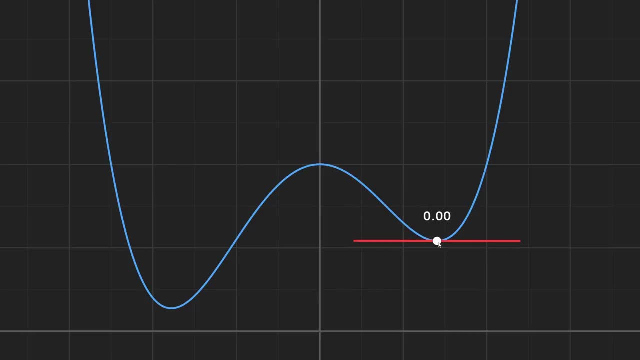 to zero as things level out, and once the function starts increasing faster and faster, we can see the slope value increases as well to reflect that. Now, for a function like this one, we could actually do some maths to directly calculate the points where the slope is zero. Which would be super easy. So let's see how that looks. So the slope value is pretty intuitive. we can see, for example, that it's negative over here, because the function starts decreasing as the input increases faster and faster, which would be super easy. 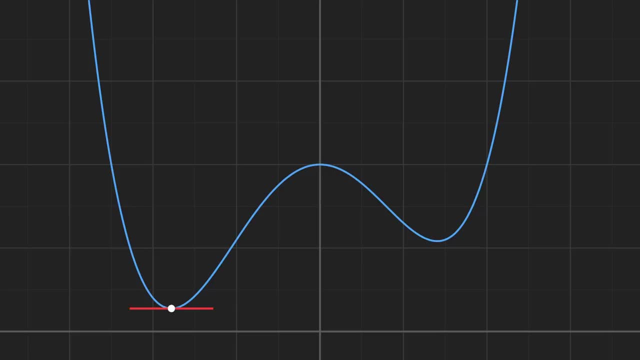 But unfortunately that math just isn't viable when it comes to our actual neural network. Instead, we're going to be relying on a technique called gradient descent, and the idea here is that we'll pick a random starting value and then just slide down the slope into the 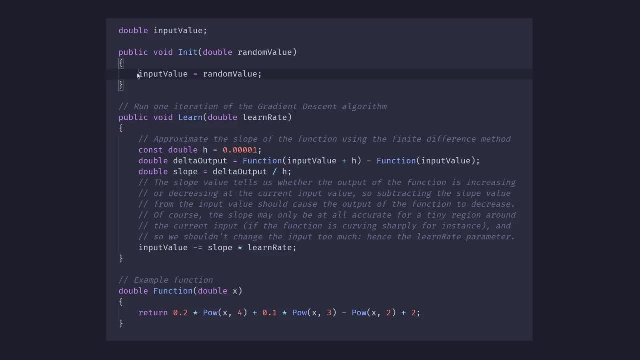 value. Here's some code for doing exactly that: It initialises the input to a random value and then, in this learn function, it approximates the slope, like we did a moment ago, and then simply subtracts the slope value from the input value. 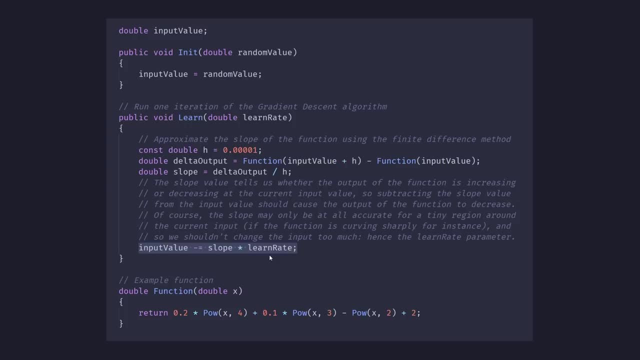 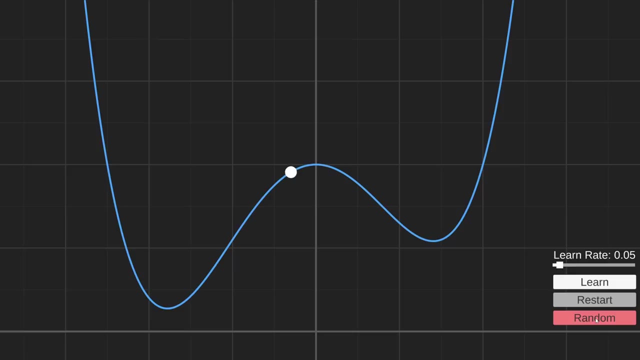 And this learn rate parameter here just allows us some control over how much the input changes with each iteration. Let's try it out So I'll give us a random starting value and then I'll just go press this learn button a bunch of times to repeatedly run the gradient descent algorithm and we can see it's very. 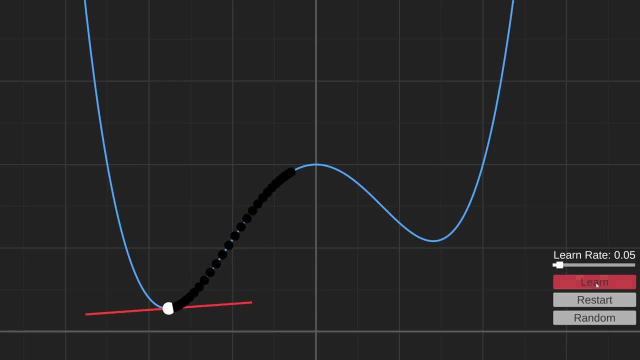 slowly making its way down the slope. Let me restart this and try again with a much higher learn rate. But now it's clearly trying to learn too quickly because it's just bouncing around all over the place and not making any kind of consistent progress. 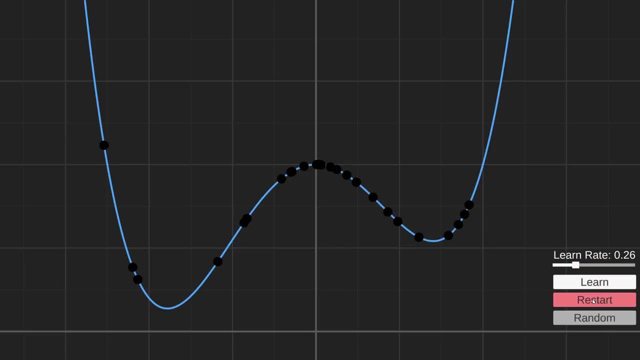 So we need to try strike some sort of balance with the learn rate, and if we manage to find a good value for our specific problem, we can see it's able to learn pretty efficiently. Of course, there's no guarantee that we'll fall into this optimal solution known as the. 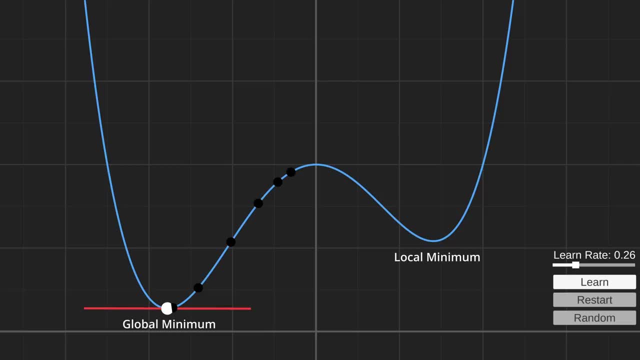 global minimum. we could very easily fall into a local minimum instead, but this process tends to give good results in practice. There are all sorts of things we could experiment with in the future to try and improve it. So to get a better picture of how this will apply to our actual network, let's pretend. 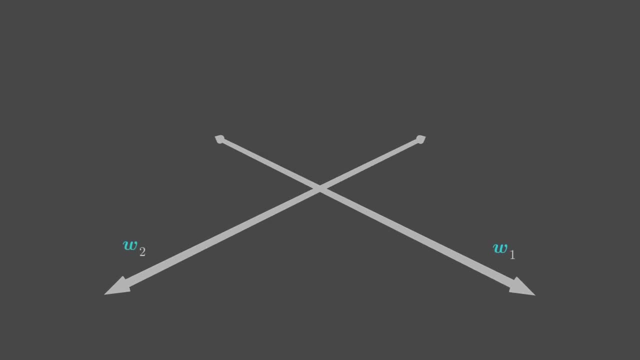 that the network has just two weights and these will start out with random values, so let's imagine them over here, for example. Now, if we want to know how good these weights are, we could run all our data through the network to calculate the average cost, and let's represent that as a height in the third. 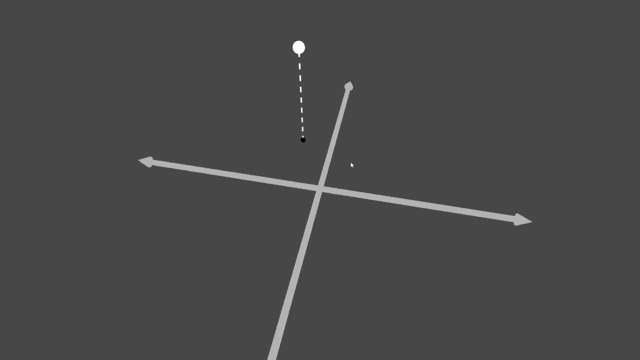 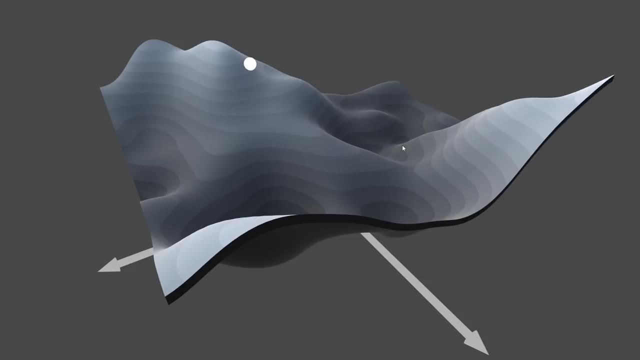 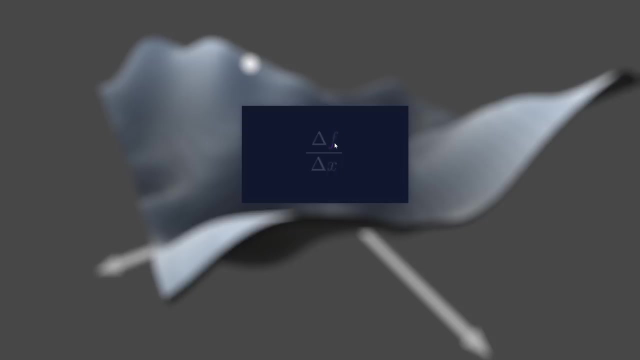 dimension. We can then imagine the average cost that would result from any configuration of weight weights as a kind of landscape like this. Now, in the previous example, we approximated the slope by looking at how a tiny change to the input variable affected the output of the function, and we could do the same. 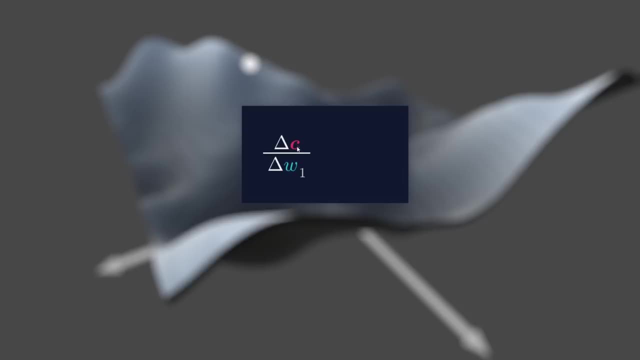 thing. here we'd look at how a tiny change to the first weight affects the cost, as well as how a tiny change to the second weight affects the cost, And these two together tell us the slope, or gradient rather, of the cost function with. 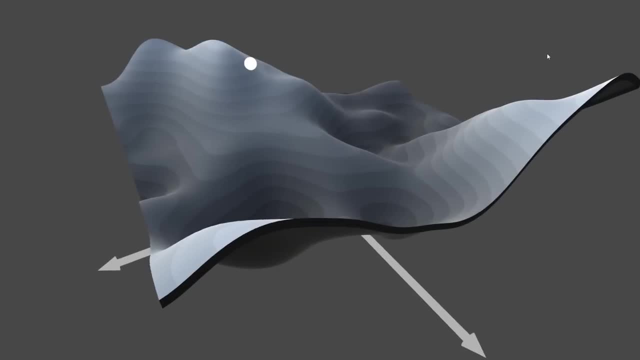 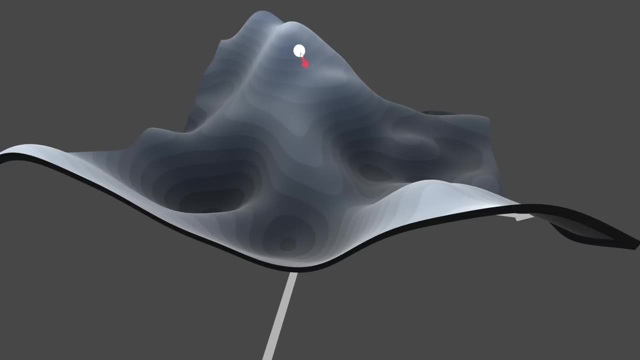 respect to the weights. So if we subtract the current gradient from the weights again using the learn rate, we'll see that the weights move downhill. And so with each iteration of gradient descent, we can imagine our weights rolling further down the slopes of the cost function before finally settling into one of the values. 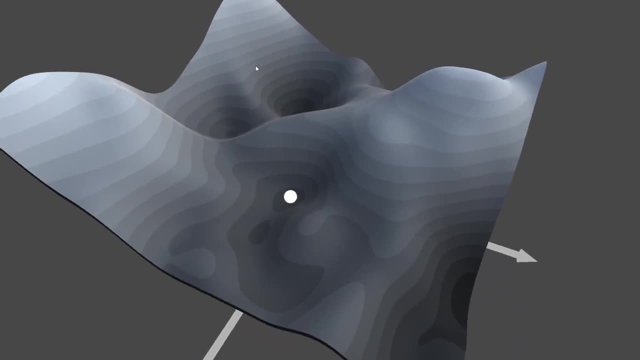 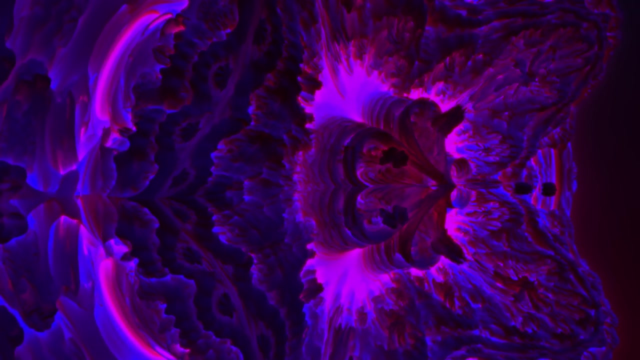 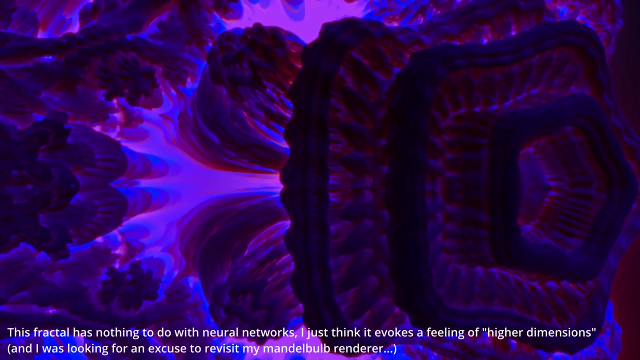 Now, obviously, in our actual network we'll have loads of weights and biases affecting the cost, so this is all happening in more dimensions than we can hope to imagine, but the idea remains exactly the same. Alright, I'm going to go ahead and implement all the stuff we've been talking about and 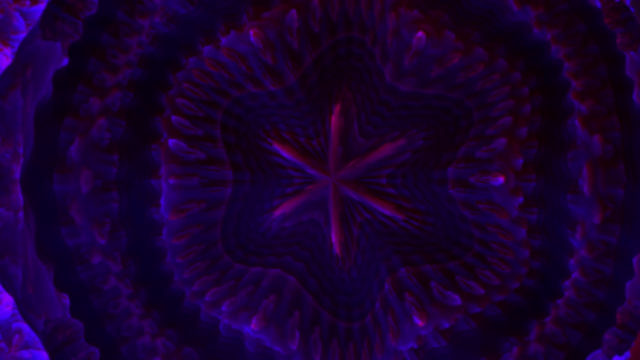 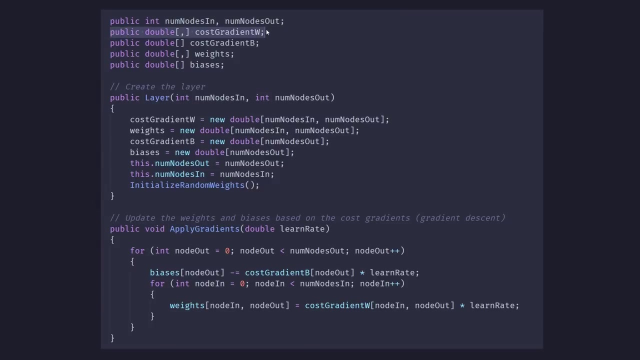 I'll see you then. So over in the layer script I've added these two arrays for holding the cost gradients with respect to the weights and biases. Then we have this new applyGradients function which takes in the learn rate and it loops. 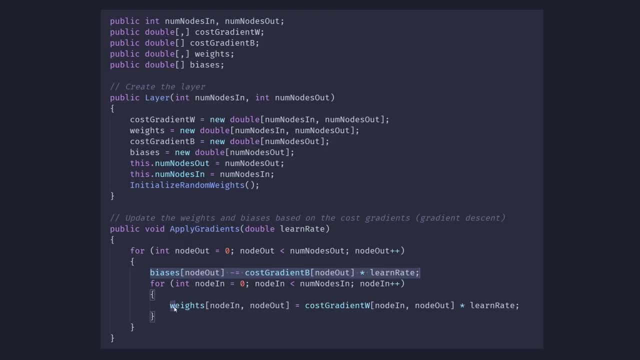 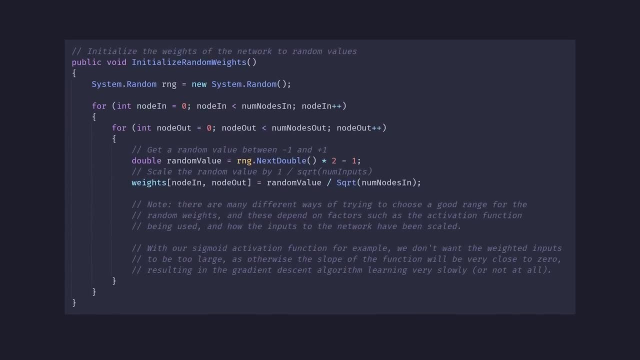 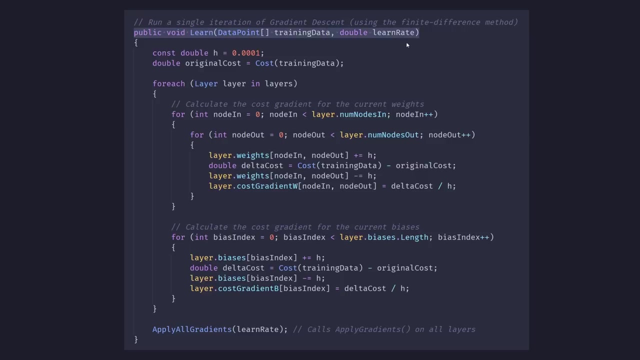 over all the weights and biases and just subtracts the corresponding value from the gradient from each of them. I've also added a function for giving random starting values to all of the weights, which looks like this: Now in the neural network script we have this new learn function which takes in all 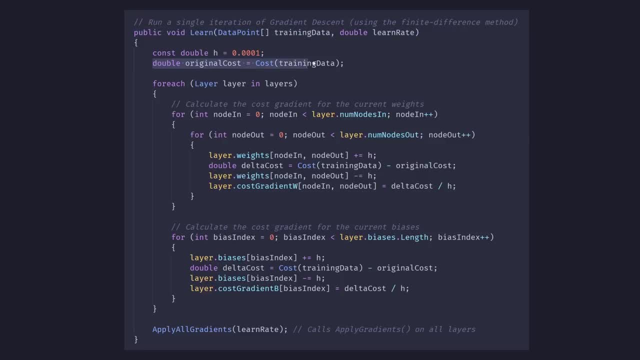 our training data and it starts off by using that to calculate the current cost value. Then, for each weight in the network, it makes a tiny nudge to that weight to measure how much that causes the cost to change, and it resets the weight after doing that, just to. 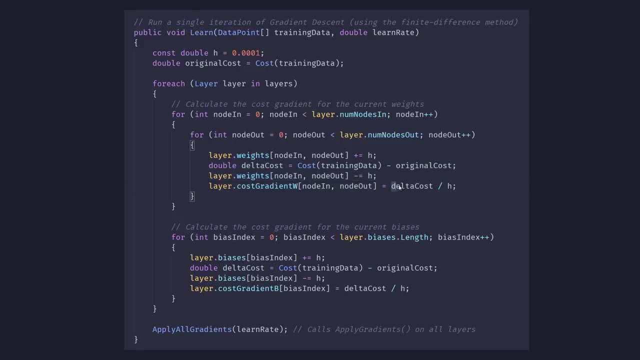 not throw off the calculations for the rest of the weights. Okay, So we have this value here, telling us essentially how sensitive the cost is to the current weight, and stores that in the gradient array. This here is just the same process for the biases and, at the end of all this, the gradients. 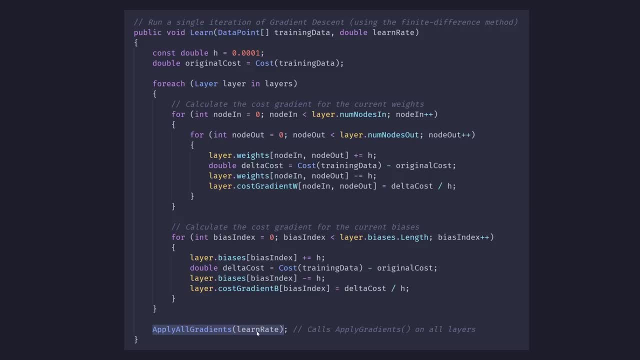 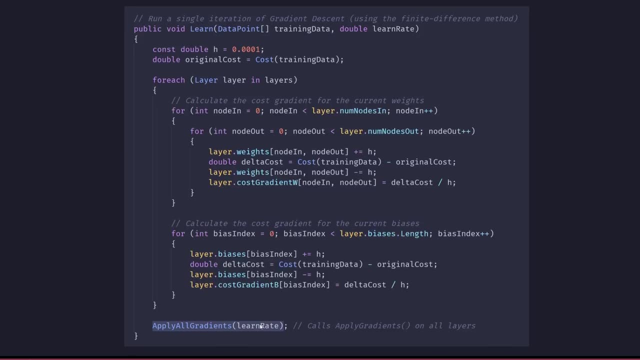 are applied on all the layers. So as long as the learn rate isn't set too high, this process should cause the overall cost of the network to decrease each time we run it. So let's return to our potentially poisonous fruit to see if it actually works. 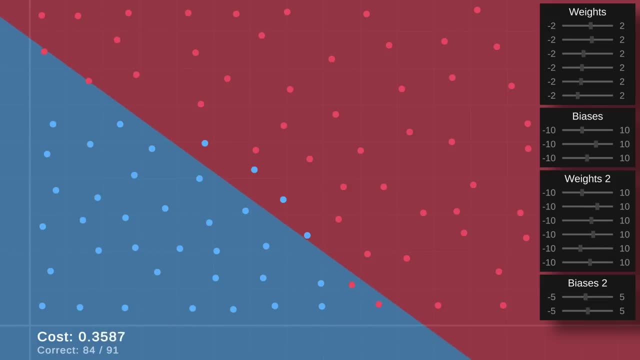 It has quickly found this linear boundary which does an okay job of separating safe from poisonous, and the cost is still going down, even though not much seems to be happening. so let's give it a little bit longer to contemplate matters. And at last it's managed to perfectly classify the training data. 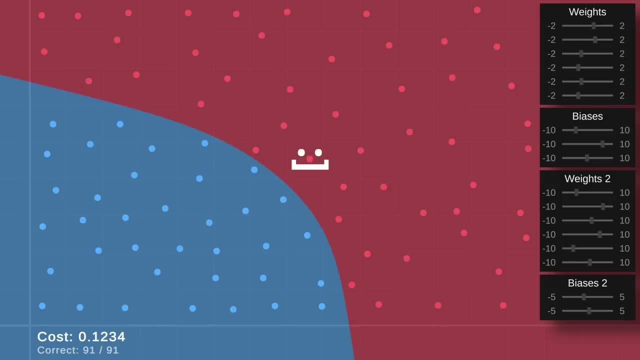 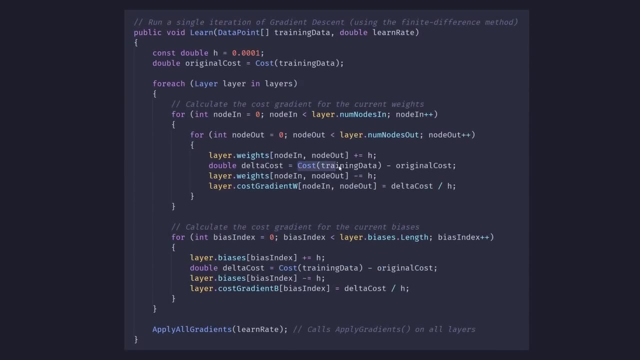 So our neural network is learning, which is exciting. The problem we have now, though, is that it's excruciatingly slow. This is mainly because we're having to run the cost function for every single weight and bias parameter and remember the cost function needs to feed all of the data it's 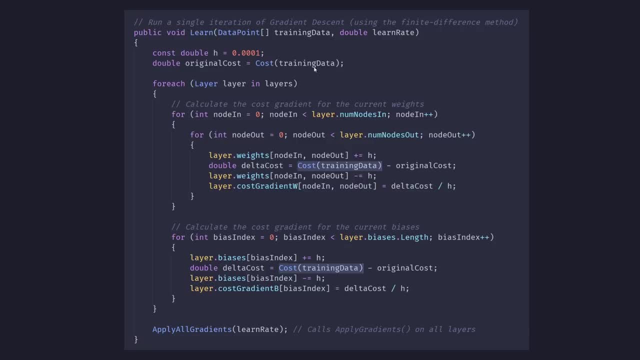 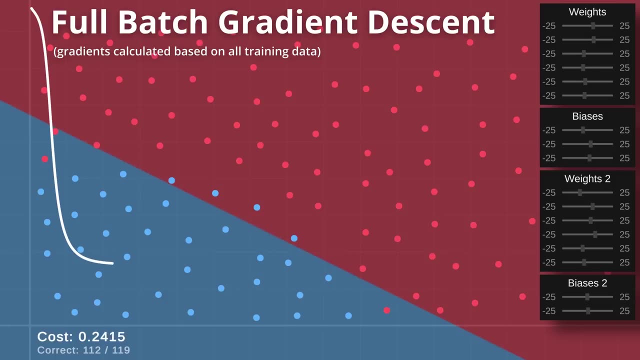 given through the entire network. So one thing we could try is simply to give it less data. When we give it all the data we have, we can see the cost goes down nice and steadily as it learns. but if we had hundreds of thousands of training samples it would take a really 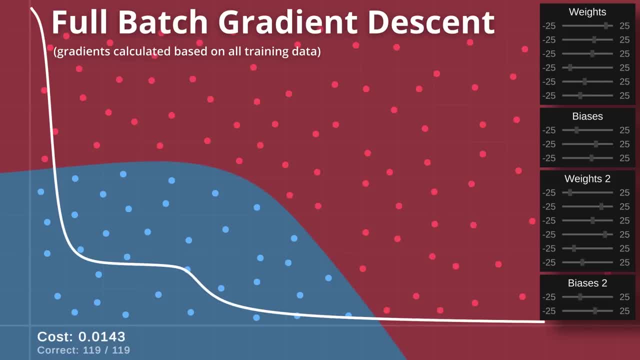 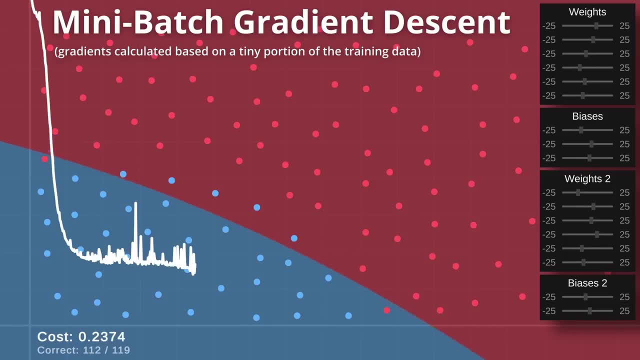 long time just to complete a single learning iteration. Instead, If we just give it a tiny portion of the data each time, we can complete learning iterations much faster. This does make the learning process noisy because we can imagine our cost landscape will look a bit different for each minibatch, so they won't all agree exactly on which. 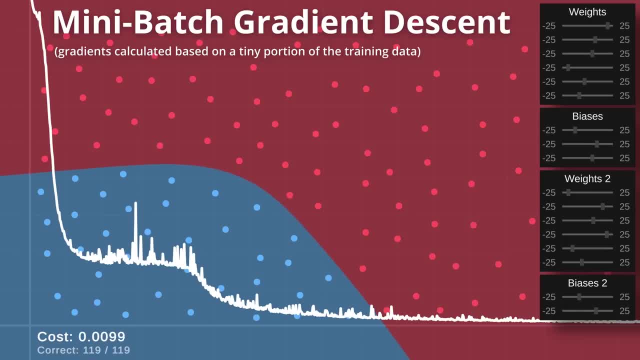 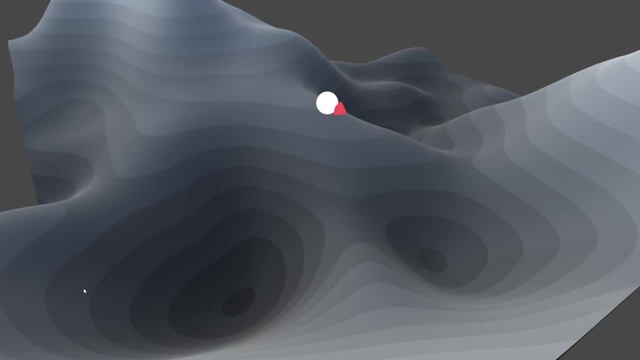 way downhill is, But it does speed things up immensely and the noisiness can apparently even be beneficial in a number of ways, for example in helping to escape the dreaded saddle point which are regions like this, Which can slow the learning process down dramatically. 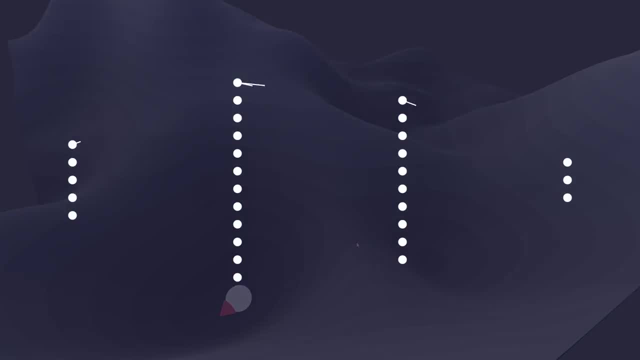 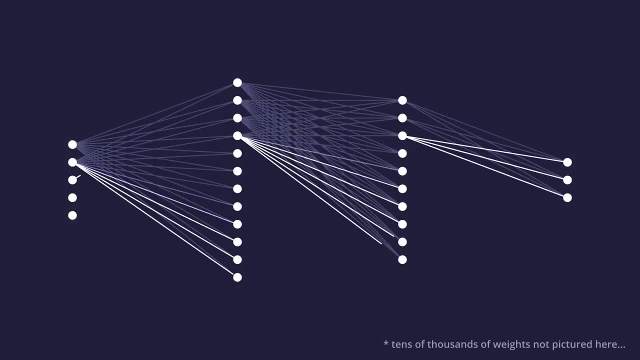 So this minibatch technique is a big improvement, but by itself it's not enough. If we want to scale our network up to, say, tens of thousands of weights- which is actually still very tiny- then that would mean running each data point through the network tens of. 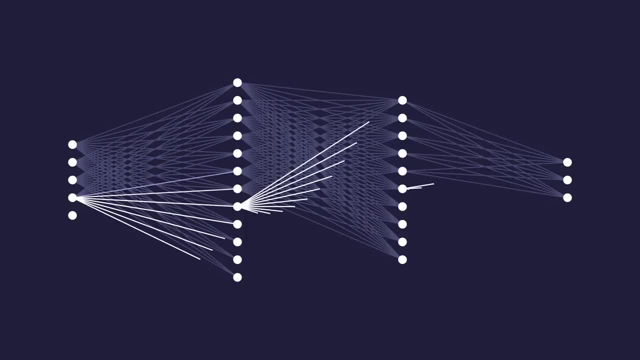 thousands of times as well, and so our network's going to take pretty much forever to learn anything interesting. Happily for us, Here's another way to calculate these gradients, where, for each iteration, we'll only have to run our data points through the network once. 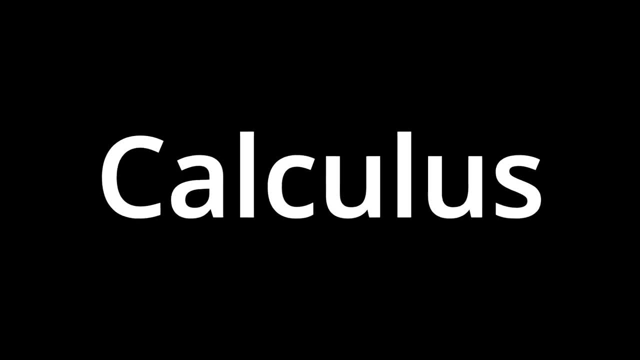 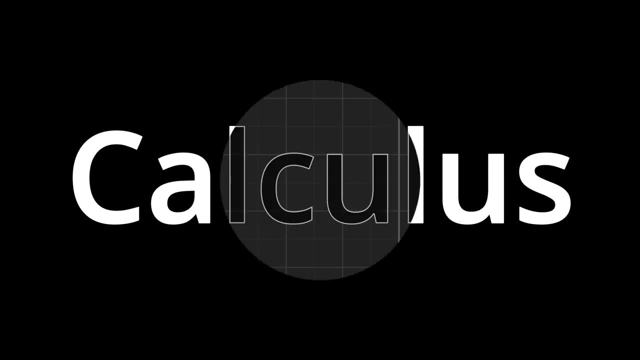 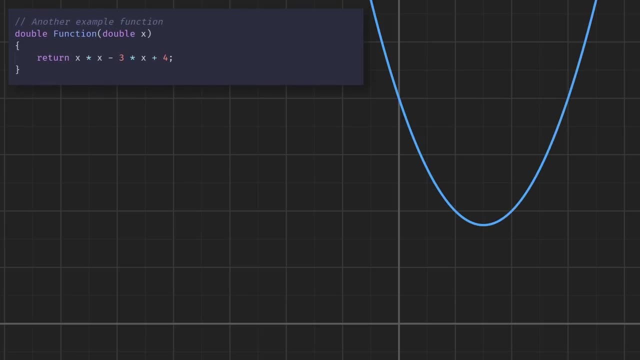 And all it's going to cost us is a bit of calculus. In case you haven't studied calculus or just need a refresher, I'd like to quickly go over the essential ideas we'll be using today. So, as an example, let's consider this function: f of x equals x squared minus 3x plus 4.. 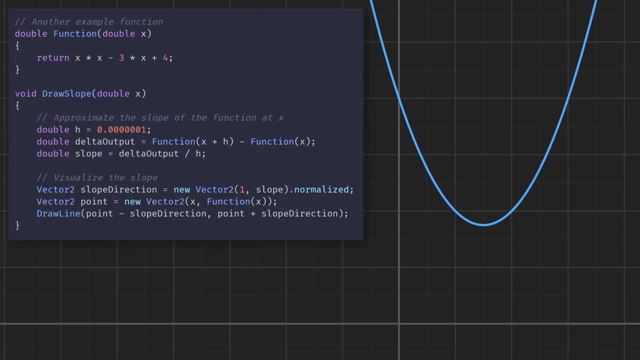 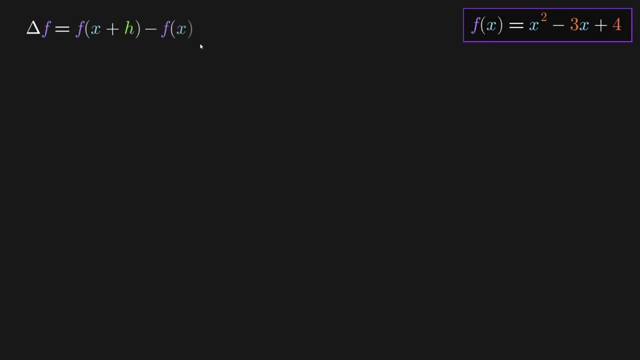 Then here's our code from earlier: We're approximating and drawing the slope of a function, and we just want to figure out a more efficient way to calculate the slope where we don't need to call the function multiple times. So let's consider this line first, which I'll write out in more mathsy notation over here. 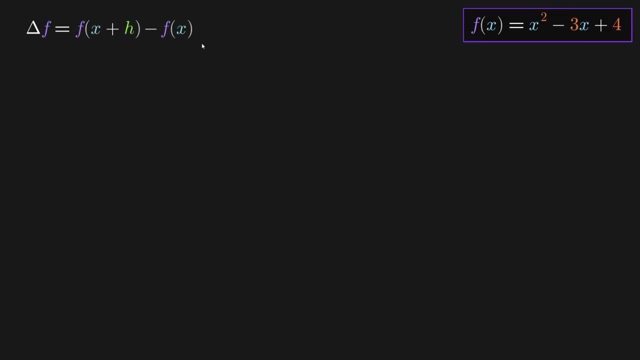 And let's just see where this takes us if we try patiently working our way through the calculation. First of all, we can write out this f of x plus h in full by just looking at our equation up here and wherever there's an x replacing that with x plus h, like so, 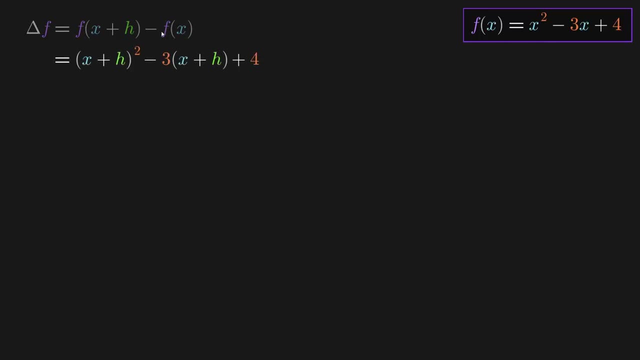 And then from that we want to subtract f of x. so let's write it out in full as well. Now, if we want to simplify this, we'll first need to expand it all. so x plus h squared comes out as x squared plus 2, xh plus h squared. then we subtract 3x and 3h, we add 4, and 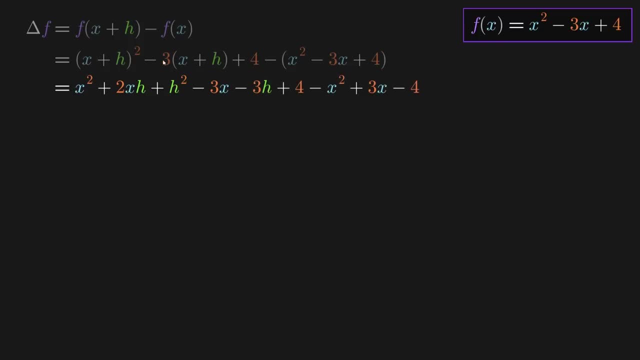 finally subtract this stuff, And now we can see that this x squared and the negative x squared will gobble each other up, As will these two terms and these two terms terms. So, once the dust settles, we've managed to simplify things quite a lot, and we can 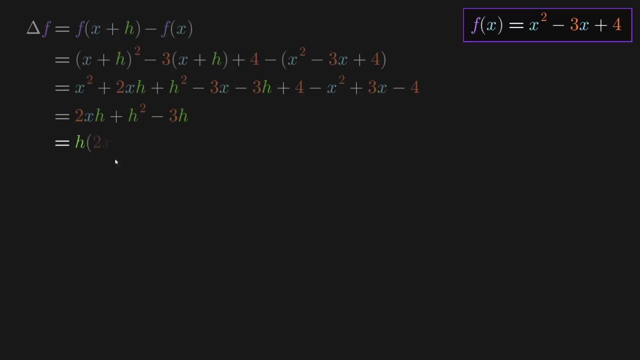 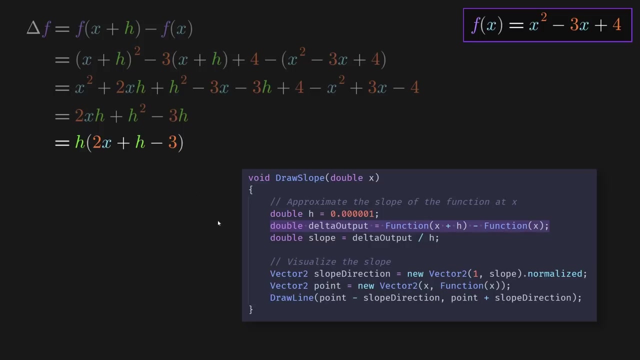 also see that h is a common factor in all these terms, so we could even neaten things up a little. That's as far as we can really take it, though. so, referring back to our code, we then calculate the slope by dividing this change in the output by the tiny change to the input that caused. 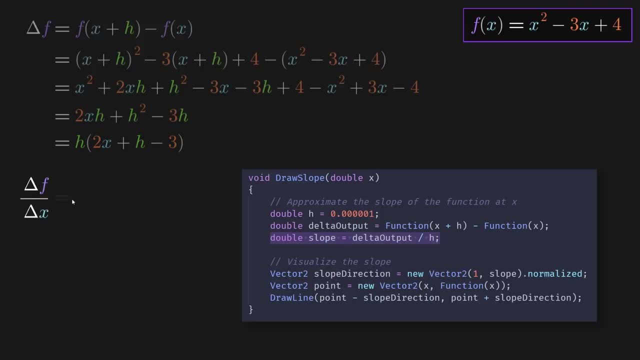 it. So let's write that out over here Right away. we can see that these two h's will cancel each other out, and we're left with just 2x plus h minus 3.. Here's where things get a little weird, though. We know that the closer h is to 0,, the more 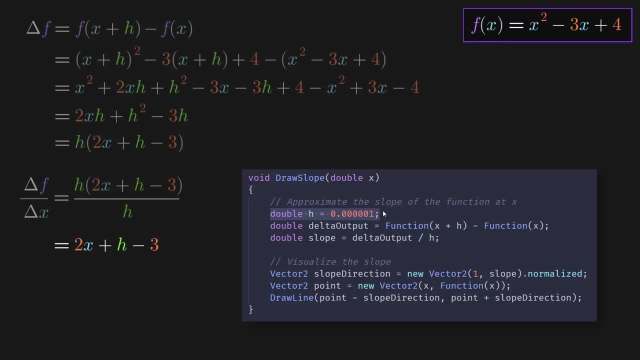 accurate our approximation of the slope will be. We also know it can't actually be 0, because then not only would the change in the output just be 0, but we'd also be trying to divide everything by 0.. Nevertheless, if our answer over here gets more accurate, the closer that h is to 0, it. 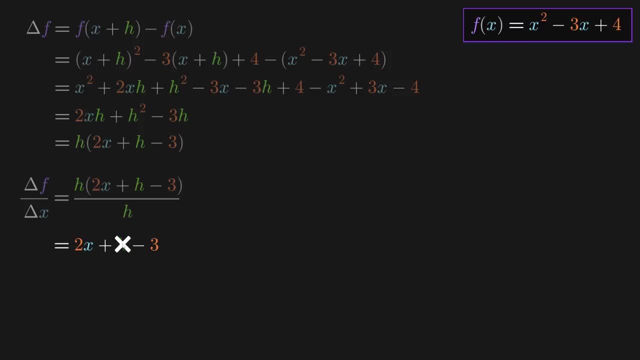 makes sense. It makes sense, intuitively at least, that we should just remove h entirely, But we don't want to be put in math jail, of course, so let's be a bit careful about this. First of all, we should switch to a proper calculus notation which looks like this: 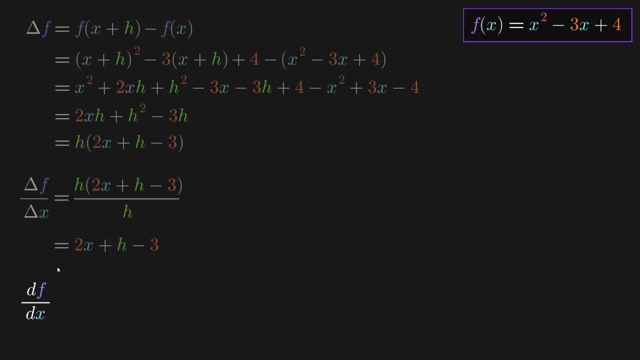 So this notation up here represents an approximation, whereas this is going to be our exact answer. We can then add this bit of mathematical legalese which just says: as h gets closer and closer to 0, this thing we calculated 2x plus h minus 3, is going to be 0. 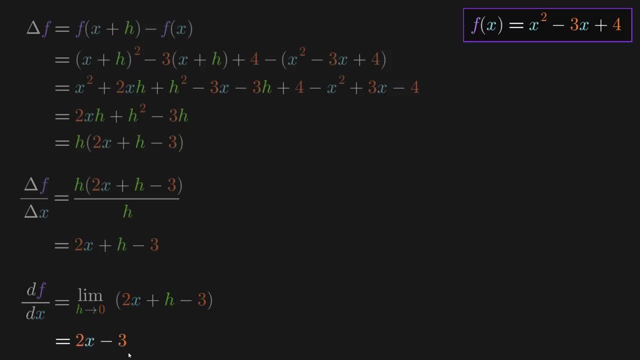 And this is going to get closer and closer to being just 2x minus 3.. So what we've calculated here is called the derivative of f with respect to x, And to see what it means, let's go back to the graph of our function and draw in its derivative. 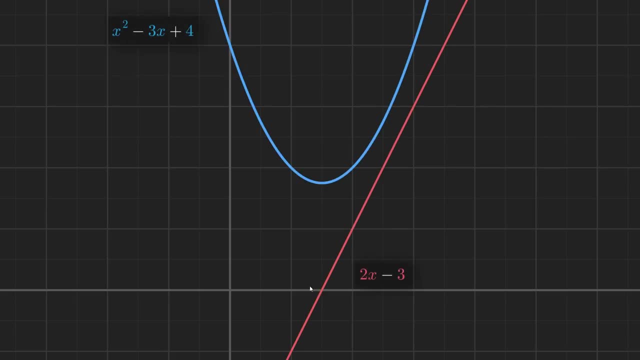 as well. Now we can see here that where the derivative is 0 corresponds to where our function has 0 slope, And where the derivative is negative, that's where the function is sloping downwards, and so on. So the derivative is this super helpful thing. 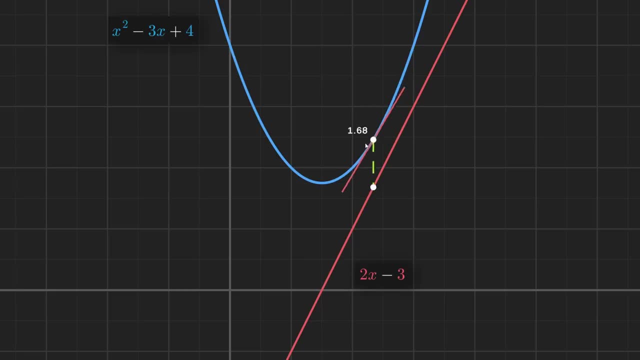 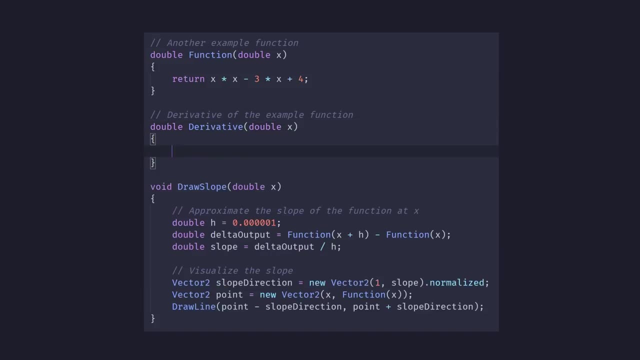 that tells us the exact slope of our function at any input value. Let's quickly go into our code and create a little function which returns the derivative we just figured out, and then we can replace all the stuff here with just a single call to that derivative function, like so: 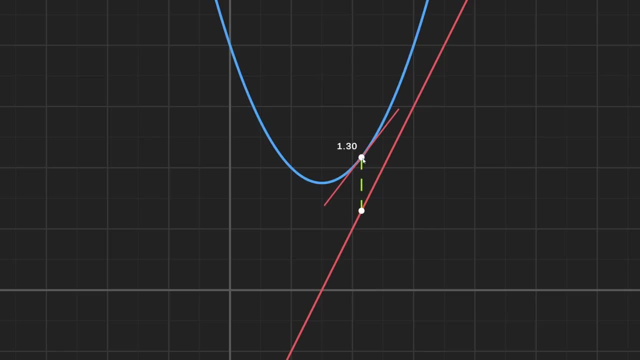 Then to test it, let's try drawing the slope again, and it works perfectly. So we've managed to make the slope calculation more accurate and more efficient, with the only downside being that we do have to actually figure out the derivative of whatever function we're. 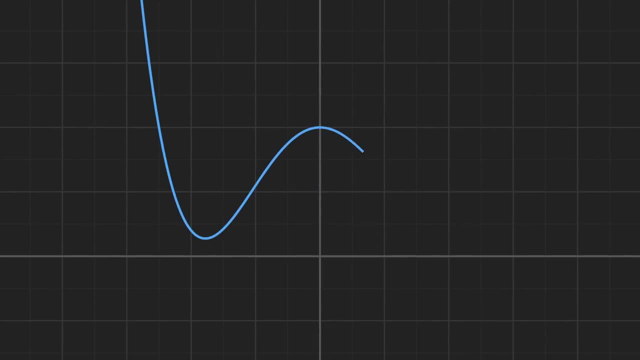 using. Just as another quick example, here's that function we used earlier when we were thinking about gradient descent, and here's its derivative. And we can see again how the derivative tells us exactly what the slope will be at any input value Or, put another way, how sensitive the 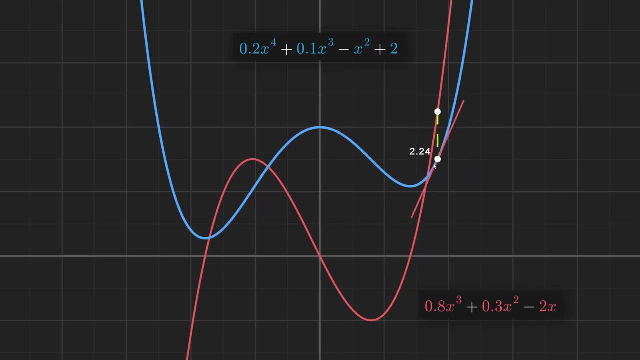 output of the function is to a change in the input. Okay, so to figure out how to do that, let's go back to our code and let's see what we can do. So, while all of this is going to actually help us, let's consider a ridiculously simplified 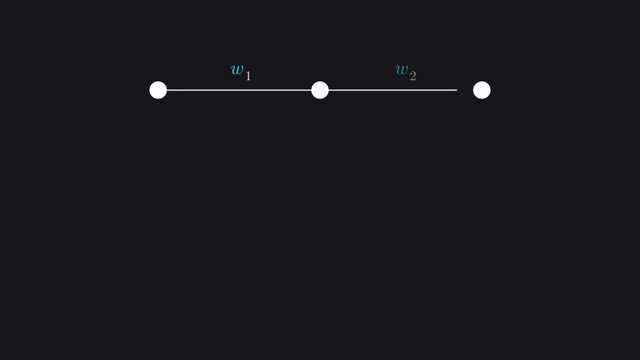 network that has just three nodes connected by two weights, like this, And let's write out quickly how this works: So the input node receives some input value, let's call that activation 0, and we then calculate the weighted input, z1 for short, which is just the input multiplied by the 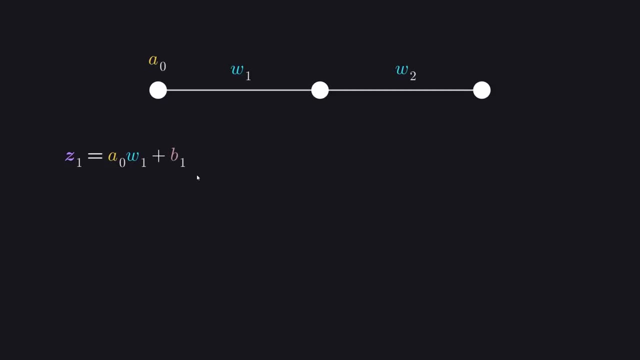 weight plus some bias value. Next we calculate activation 1, simply by passing the weighted input into our activation function. We then do the same thing to calculate z2, and finally a2.. We can now evaluate the network by calculating the cost, so we just use the cost function. 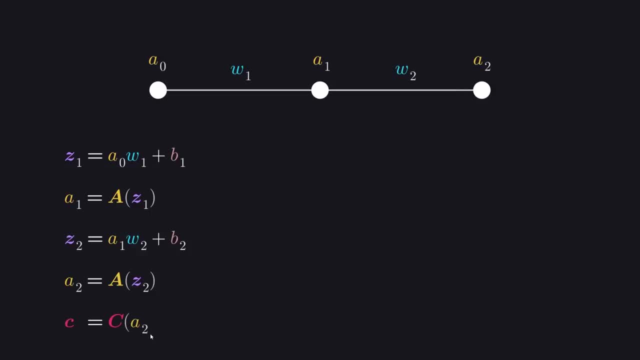 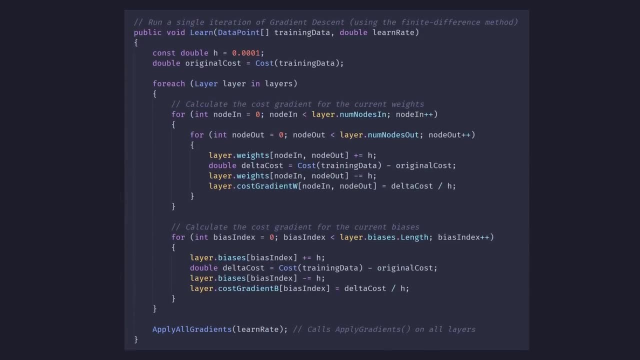 and pass in the output activation value along with the expected output for the current training sample, or y for short. Now, if we think back to this horrifyingly inefficient gradient descent code that I wrote, remember what we're trying to speed up is this calculation here of how sensitive the 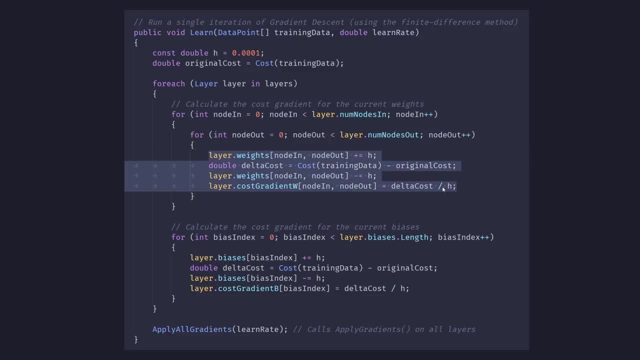 cost is To a change in the input value. So we can calculate z2, and finally a2.. We can calculate z1, and finally a2.. To a change in any particular weight or bias parameter. So let's say we want to calculate that value for weight number 2 over here Instead of 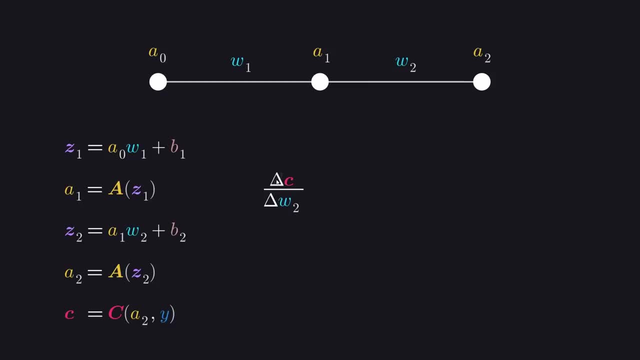 approximating it. we've seen recently that we can actually get a more efficient answer by calculating the derivative, And I'll write this with these fancy curly d's, since we're dealing with functions with multiple variables. now, Anyway, this might look a bit confusing to calculate, because we're trying to figure. 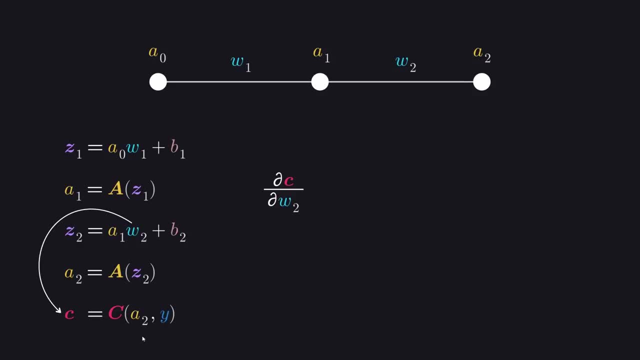 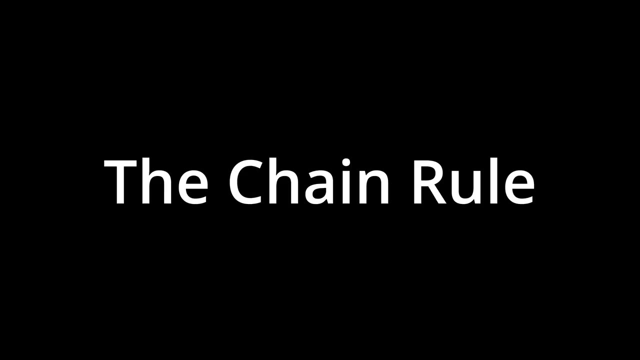 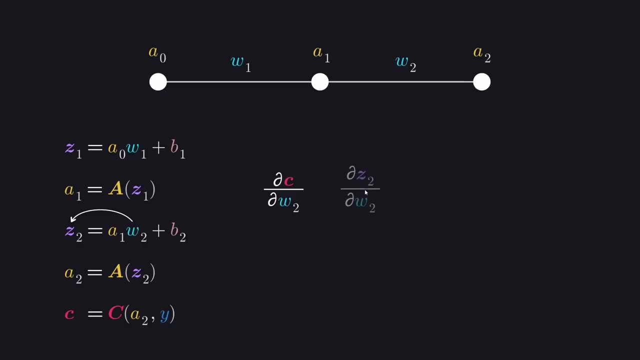 out how w2 affects the cost, but it isn't one of the cost functions' inputs. So let's get started To unravel this mystery. there's one final calculus concept for us to contemplate today: The chain rule. The chain rule tells us to simply look at how w2 affects z2, which you can write out: 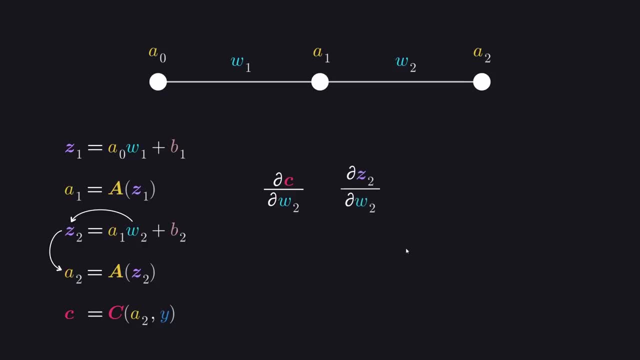 like this: And then look at how z2 affects a2, which I'll write out over here as well- And finally look at how a2 affects the cost, which, once again, I'll write out over here. All we need to do now, according to the rule, is multiply these partial derivatives together. 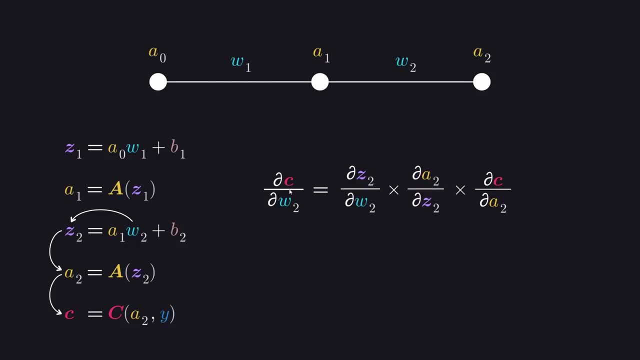 and it will give us the result we want. So let's do that. We can even kind of see that this is true, because if we think about how fractions cancel out when you multiply them, this gives us the correct result. So our task now is figuring out what each of these partial derivatives actually is. 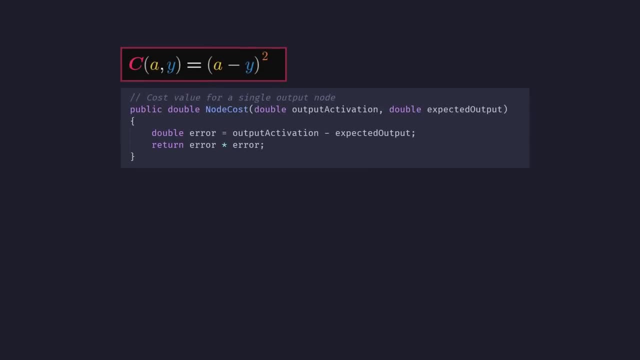 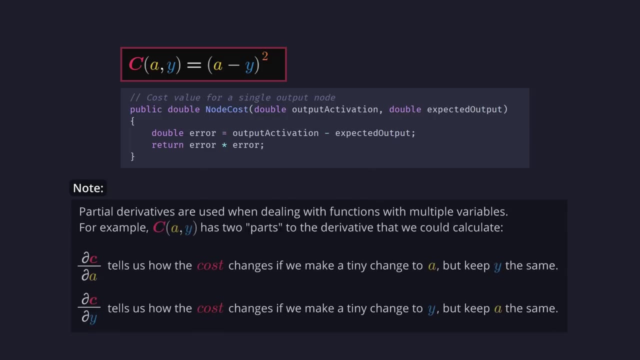 and let's start with this one on the end. Here's our code again for calculating the cost of a single node, and we need to figure out the partial derivative of this with respect to the output activation value. There are shortcuts for doing this sort of thing, So let's do that. 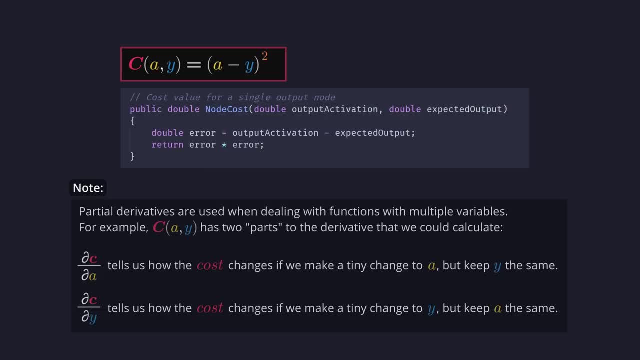 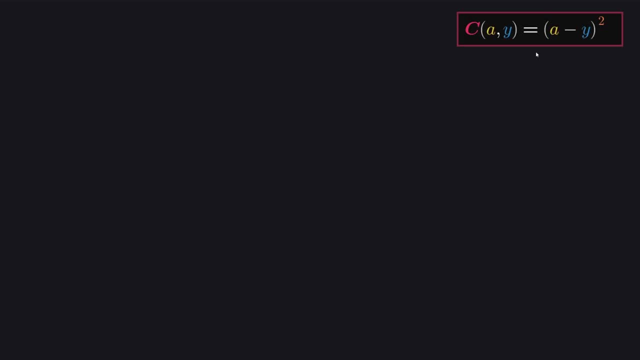 But I'd just like to quickly show how the approach we used earlier still works exactly the same way for a multivariable function like this one. So over here we're looking at how the cost changes in response to a tiny change to this output activation value, and we're then dividing by the size of that change, Like before, let's. 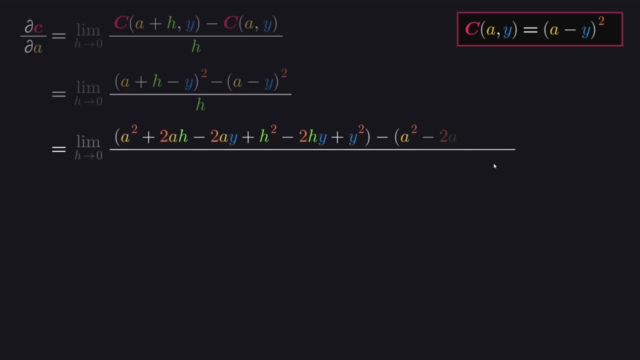 write this out in full and expand everything, which is pretty tedious, but we then get to cancel a bunch of stuff out, which is always satisfying. I'll tidy that up and we can see once again. we end up being able to cancel out this division. 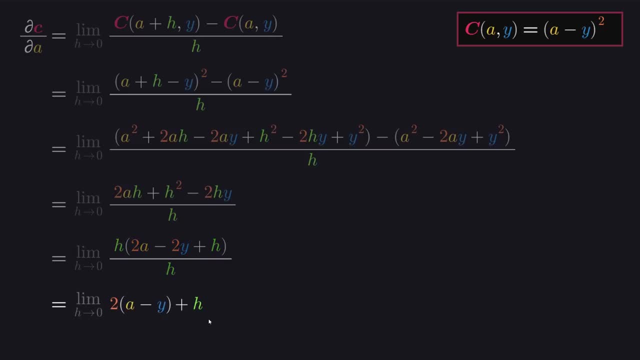 by h, which is crucial to the final step of then being able to say that as h approaches 0, this is going to approach simply 2 times the output activation minus the expected output. So there's our answer, and in code that would just look like this: 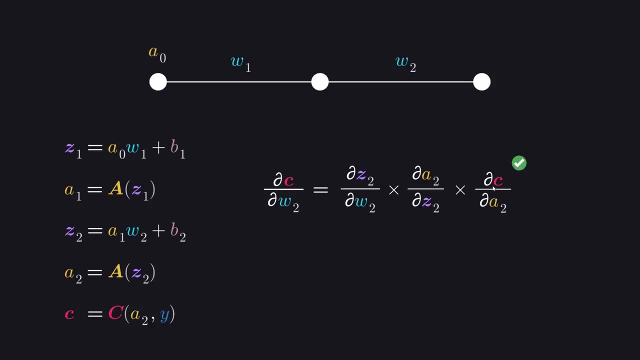 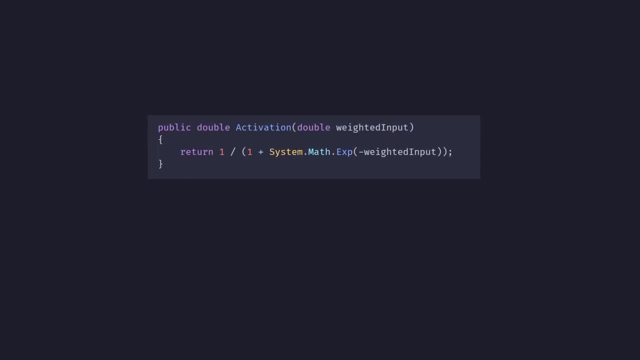 Okay, so we figured that one out. Next let's look at how the activation changes in response to the weighted input. So here's that sigmoid activation function we're currently using, and calculating its derivative is quite a bit more involved than the others, so I'm just going to skip right to the answer, which. 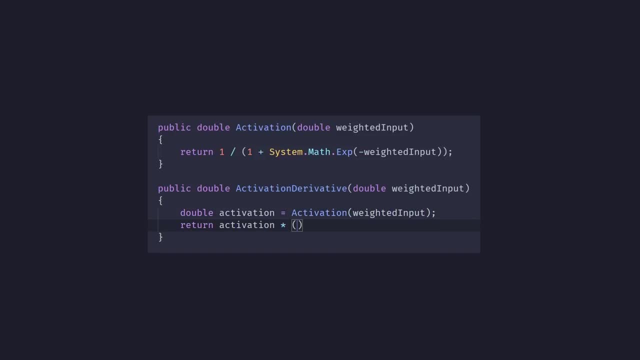 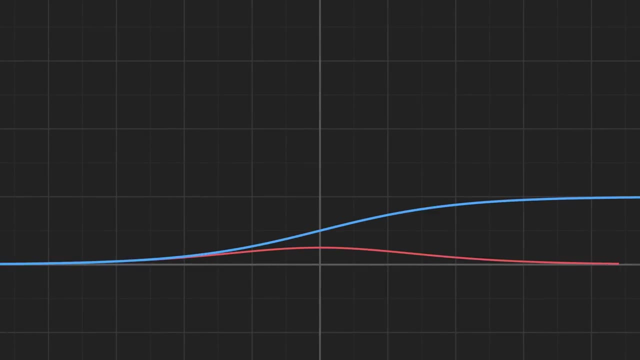 turns out to be simply the activation value multiplied by 1 minus the activation value. Let's quickly graph it, at least just for interest's sake, and here's what it looks like. Alright, for this last one. we want to know how the weighted input changes in response. 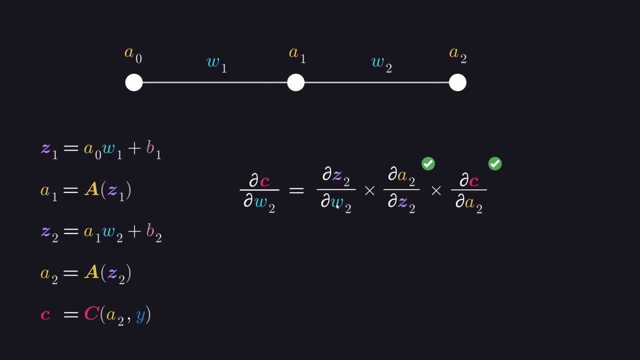 to the weight. This one's very easy, because if we just look at our equation here, we can see that the amount of effect that a change to the weight will have on the weighted input depends entirely on the input which is this a value here? For example, if a is 0, then changing the 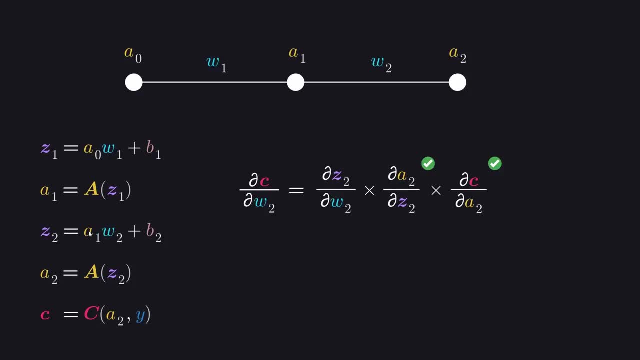 weight would have a 0 effect, whereas if a is 10,, then changing the weight would have a 10 to 1 effect. So if a is 10,, then changing the weight would have a 10 to 1 effect. So 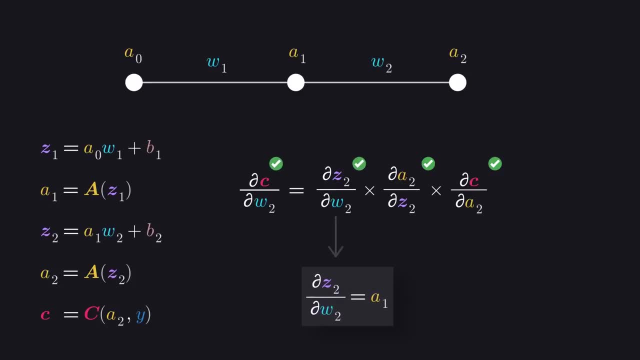 that's our answer. We now know how the cost is affected by the second weight. we just need to figure out the same thing for the first weight. So here's the partial derivative we want to calculate, and if we just look at how the 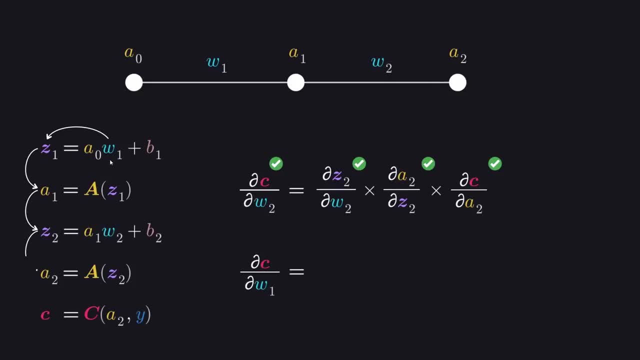 first weight ends up affecting the cost. we can again use the chain rule to figure this out. Taking a closer look, we can see that these two partial derivatives on the end are the exact same as these two, So we know those two. 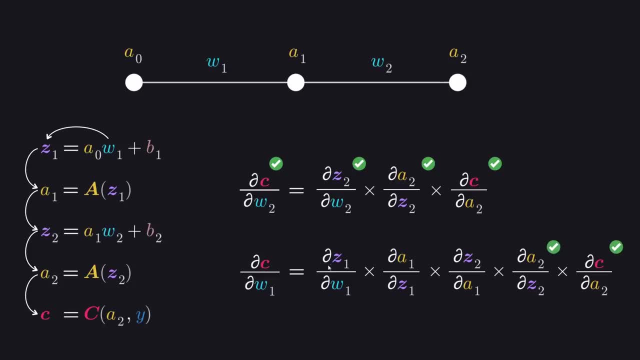 Then over here, this is the same thing as this, just taking place in a different layer, so we already know how to calculate it, And it's the same story, with this one being the same thing as this, just again in a different layer. 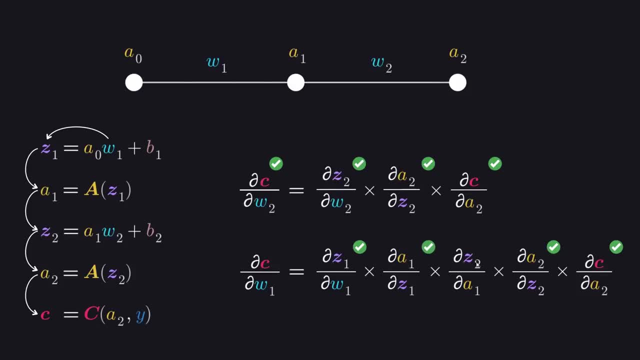 So all we need to worry about, then, is how the weighted input changes in response to the input. But again, if we just look at this equation here, we can see that the amount of effect that a change to the input will have on the weighted input is determined entirely. 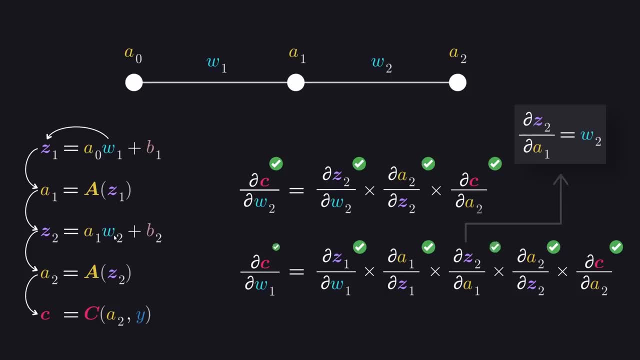 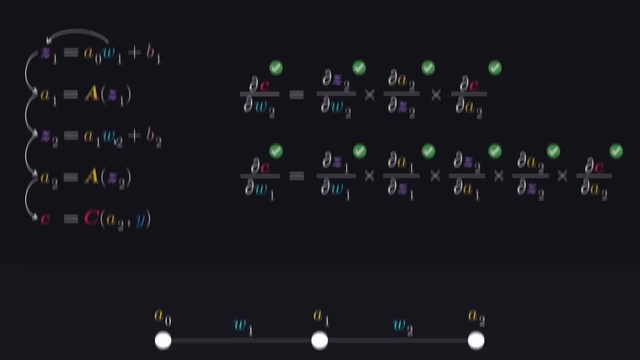 by the value of the weight. So there's our answer, And we now know how the cost is affected by both of the weights in our tiny network. Okay, I'm going to tidy these notes up a bit, because it's time for our little network to. 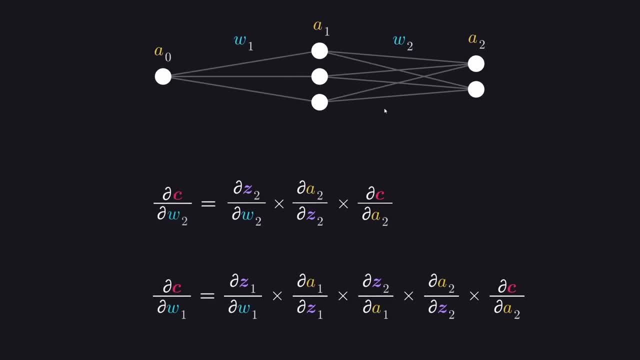 grow up. This does mean that our notes here don't make total sense anymore, but they do translate fairly intuitively, I think. so they're going to guide us as we work through this. Let's begin with this calculation over here, where we're taking the partial derivative. 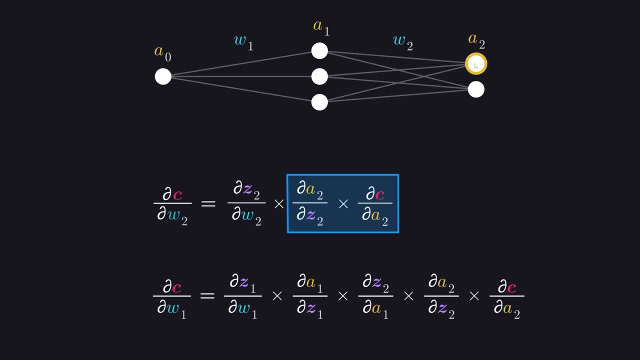 of our output node and multiplying it by the derivative of the activation with respect to the weighted input. Of course, we now have two output nodes and that just means we'll do the same calculation again, but using the activation of this other output node and its 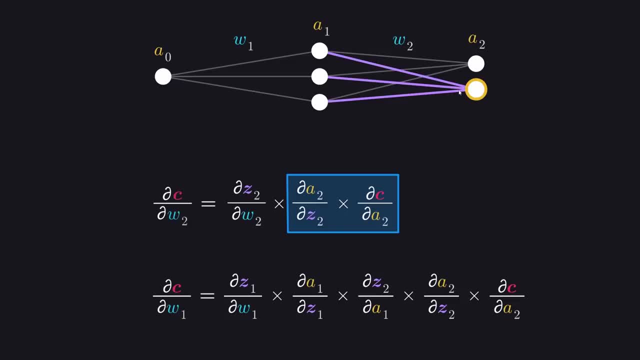 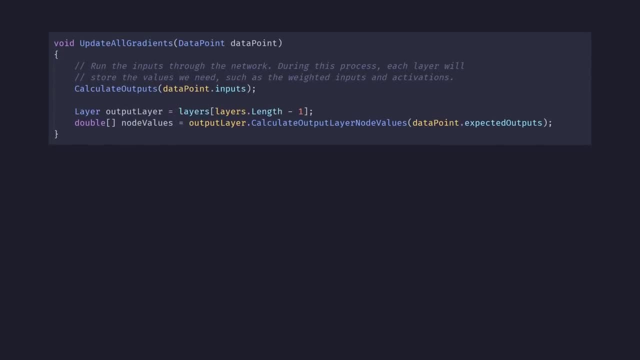 weighted input instead. So we end up calculating two separate values, which I'm just going to call our node values, because I'm bad at naming things. So over in the neural network script I have started working on this little function which takes in a single data point and runs it through the network. 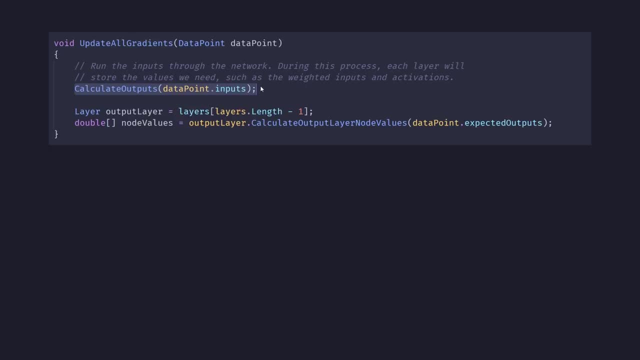 And I modified the layer code slightly so that, when that happens, each layer stores all the information we're going to need, like the weighted inputs and so on. After that, it asks the output layer to calculate the node values, which it does, just like we. 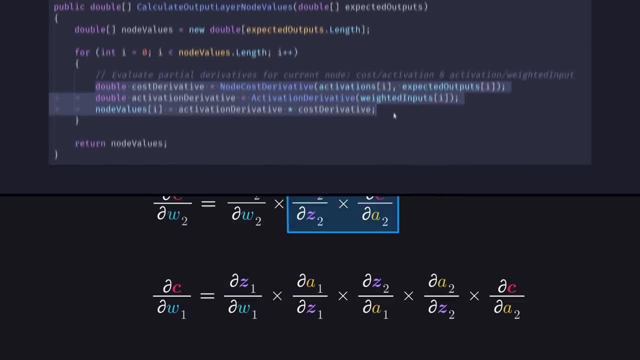 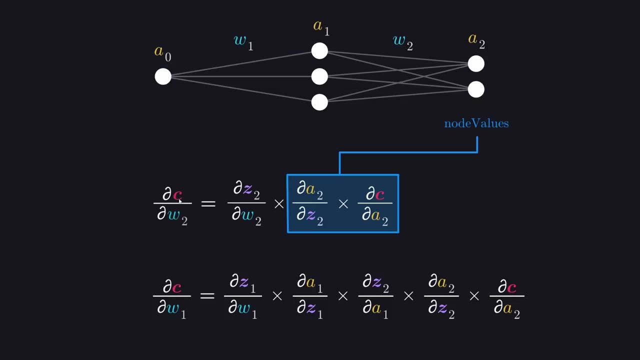 talked about. Alright, so we're now ready to figure out how each weight in the final layer is affecting the cost. So that means we'll actually be calculating six different values in this example, One for the weight of each of our connections here. 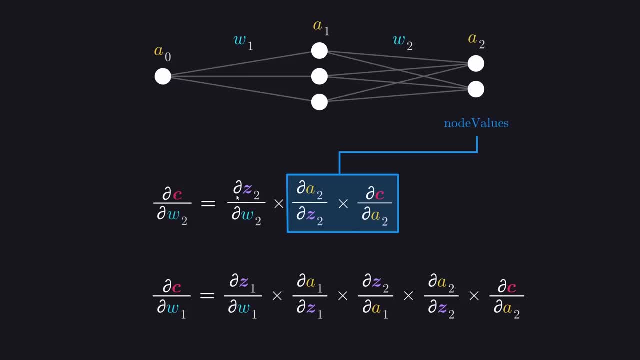 To do this, we need to multiply our node values by this partial derivative here, which we figured out earlier, was just the activations from the previous layer. How that'll work for this connection, for example, is we'll take the activation from the previous layer that's going to be input along the connection and multiply it by the node value that it. 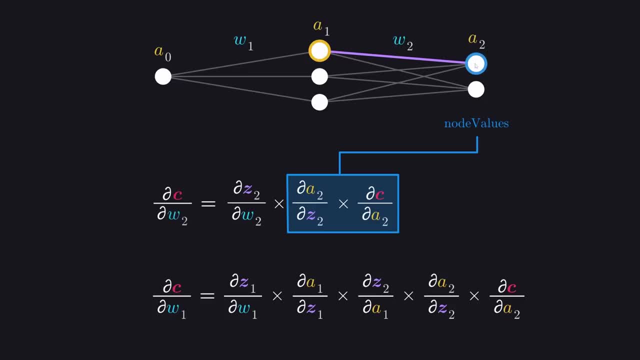 connects to on the other end, And we'll be doing that for all of them. So, just as another example for this connection, we'd be taking the activation coming out of this node And multiplying it by this node value on the other end. 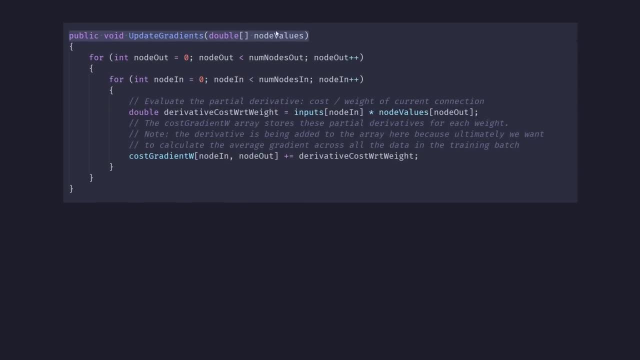 So over in the layer script I've made this updateGradients function which takes in the node values and then for each connection it calculates the partial derivative of the cost with respect to the weight of that connection and then uses that to update the gradient. 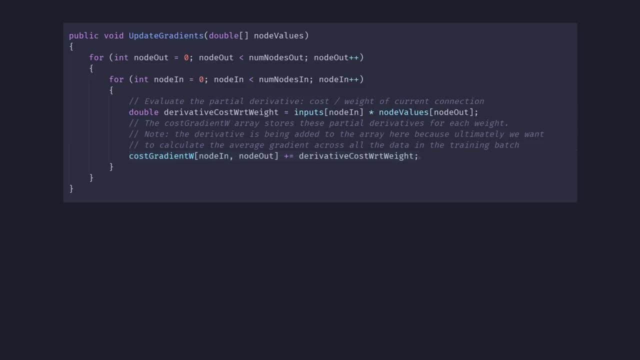 While we're here, we should actually also be updating the bias gradient. So to figure that out, let's quickly tweak our maths to be with respect to the bias instead, And we can see that we just need to multiply the value of the cost with respect to the. 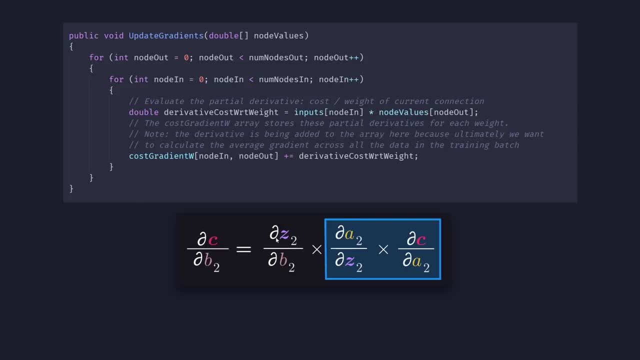 node values by whatever the partial derivative of the weighted input with respect to the bias is. So let's once again have a look at this equation, and here we can see that there's nothing affecting the bias value, which means that however much the bias changes, the weighted input will change by. 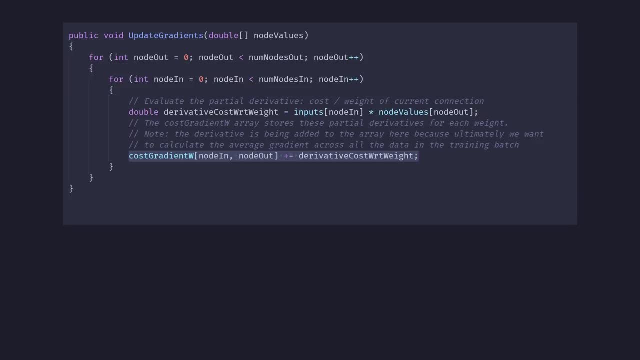 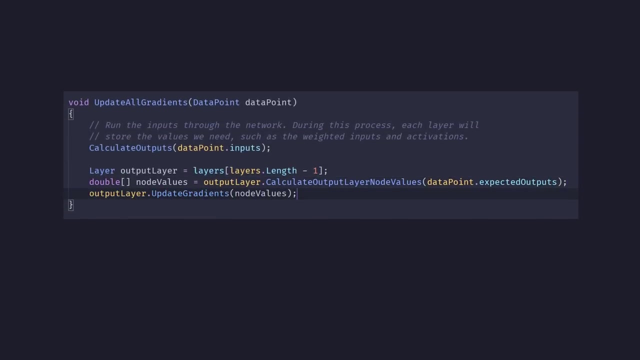 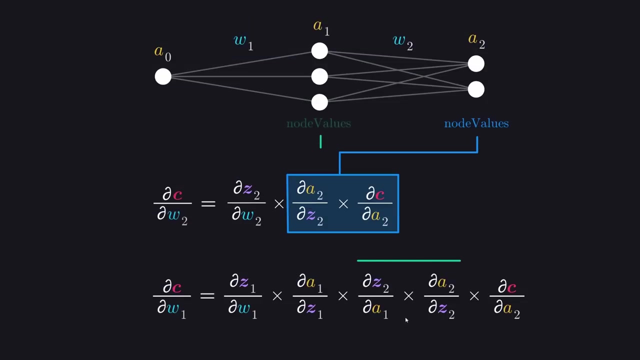 the same amount, So that partial derivative is just 1, and I'll go ahead and add that to the code quickly. Then, back in the neural network script, we'll of course tell the output layer that the output is 1.. So we can now move on to our second equation here, and let's focus on calculating this. 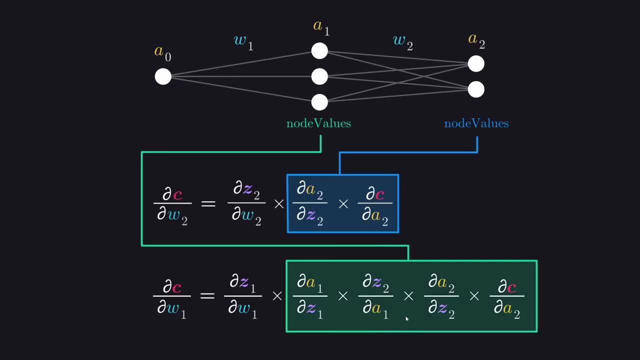 new set of node values for our hidden layer. As we noticed before, this uses the old node values in its calculation, so we first just need to take those and multiply them by. this partial derivative here, which we figured out earlier, is the weights between the two layers. 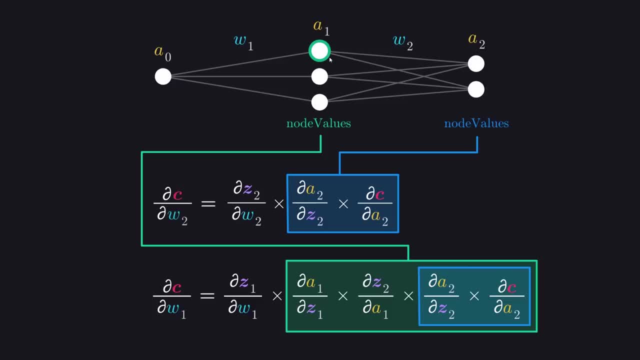 So how this works is that the first of the new node values here is 1.. So how this works is that the first of the new node values here will be equal to the weight of this connection multiplied by the old node value it connects to, plus the weight. 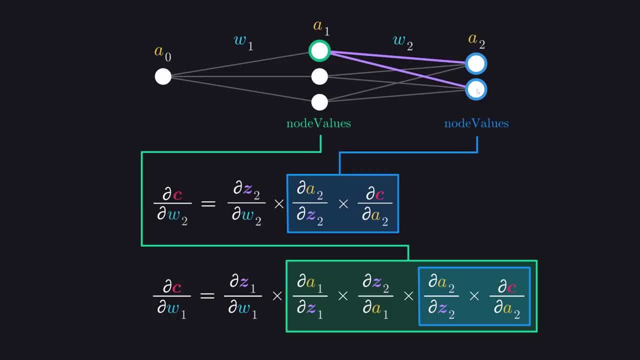 of this connection multiplied by the old node value that it connects to, And then, as you can probably guess, the second new node value will be equal to this weight multiplied by this old node value, plus this weight multiplied by this old node value. 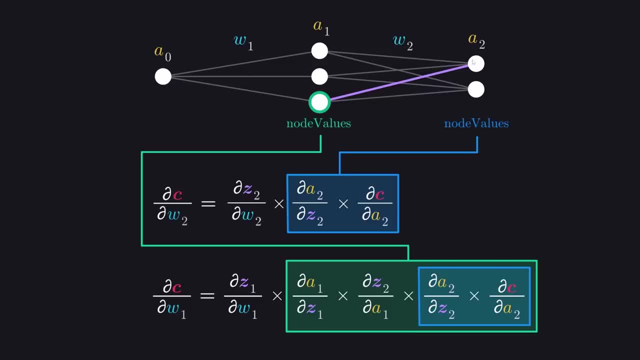 And same thing for our third new node value. But the calculation for these new node values is not quite done yet. we still need to do this bit, and so each of those new values will just be multiplied by the derivative of the activation function with respect to its weighted input. 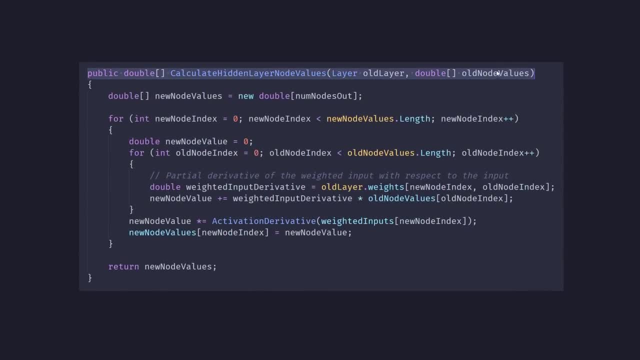 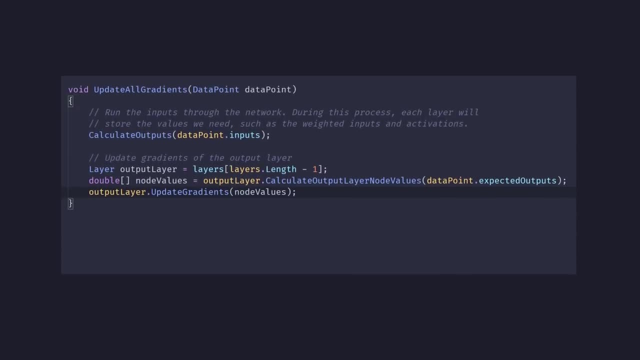 So here's our final addition to the layer script. this function takes in the old node values and uses them to calculate the new set of node values, like we just talked about. Back to the neural network script to finish things up over there as well. 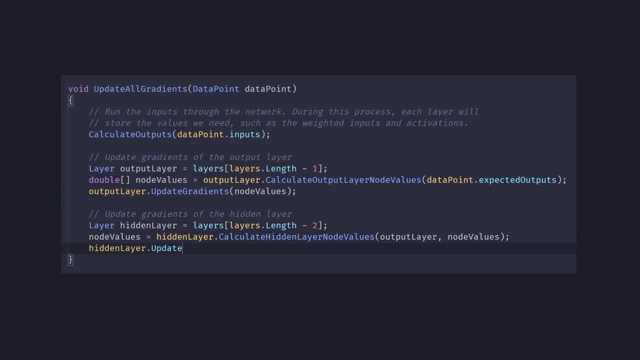 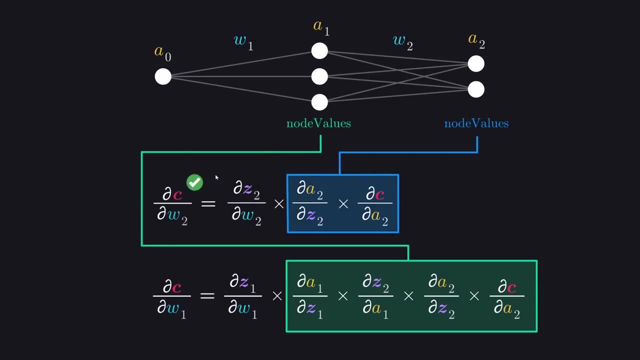 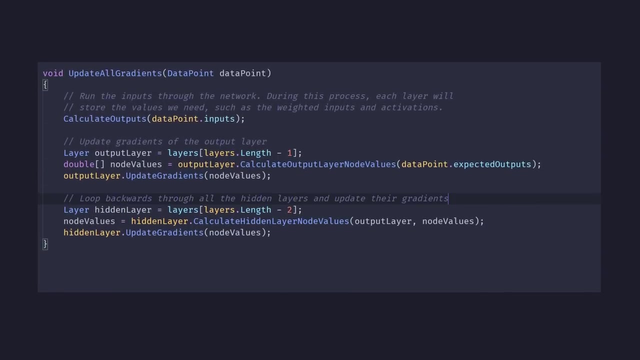 So we can create our new node values here and then just use those to update the gradients of the hidden layer And at long last we've now completely implemented our two equations. Of course, this implementation only works if we have just a single hidden layer, but 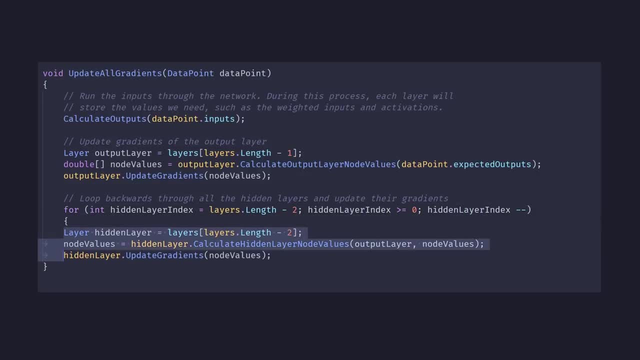 we can very easily modify it with a little loop so that it can handle any number of layers. So let's go back to the neural network script to finish things up over there as well, So we can create our new node values here and then just use those to update the gradients. 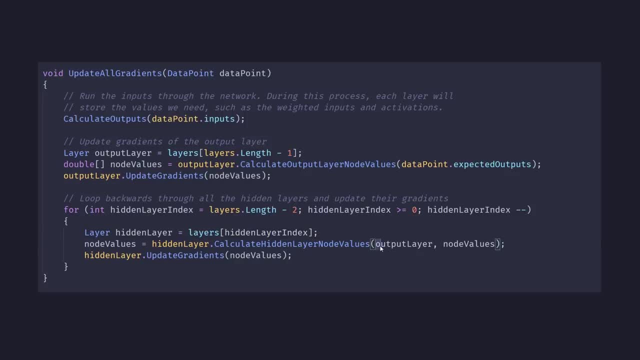 of the hidden layer. By the way, this approach of starting with the output layer and going backwards through the network so that we can keep reusing these node value calculations, is known as the back propagation algorithm And, as we can see, it's only running each data point through the network once, or I. 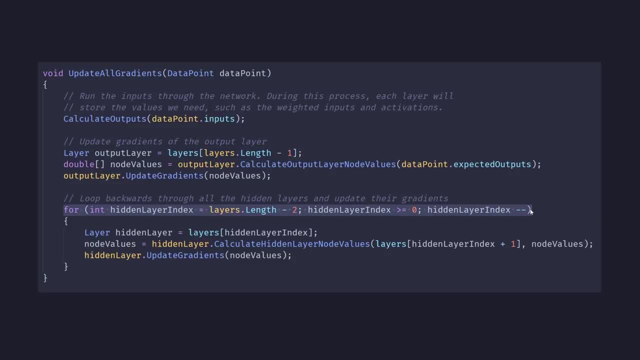 guess we could call it twice, since it does have to go backwards through the network as well. But that's a huge improvement over having to do it for every node. So let's go back to the neural network script to finish things up over there as well. 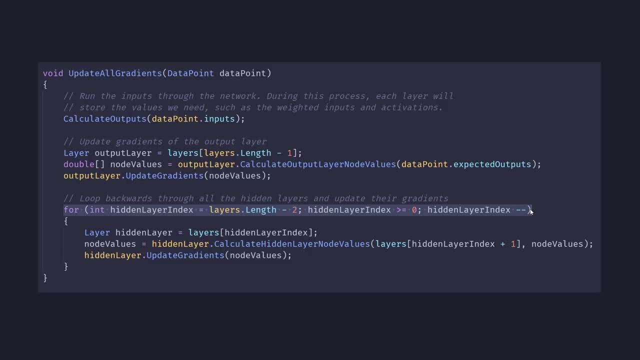 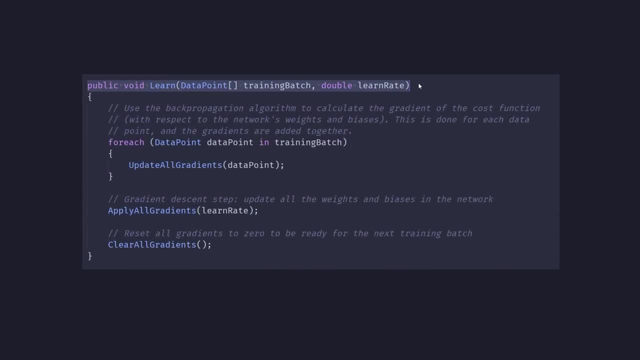 Anyway, now that we're able to update the gradients for a single data point, I've made a new learn function to replace the old slow one, and this takes in all the data points in the current training batch and adds up the gradients for each of them. 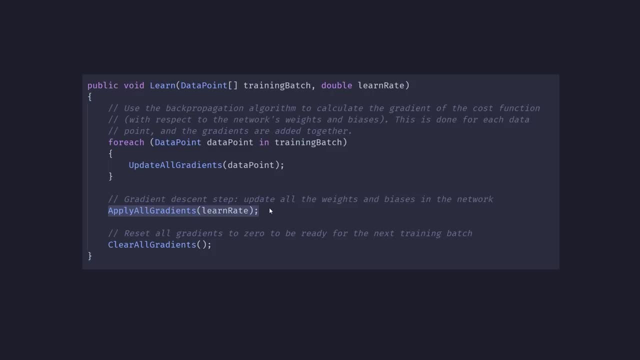 After that it just performs our gradient ascent step by telling all the layers to apply their gradients. And remember they multiply the gradient by the learn rate when doing that. so if we just divide the learn rate by the size of the training batch, then we get the gradient ascent. 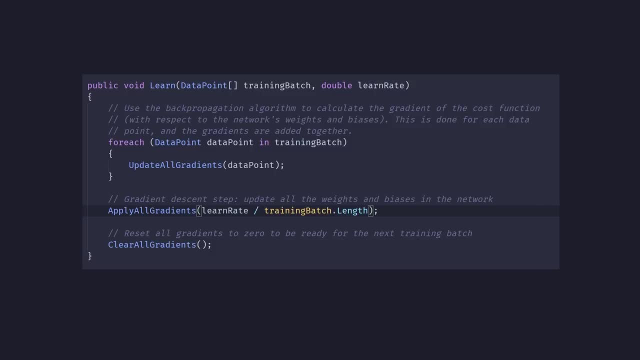 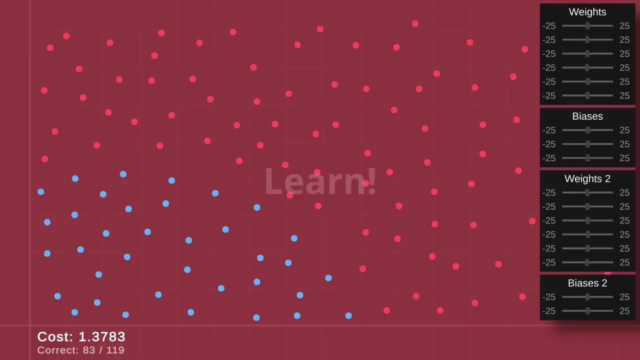 With that, our new learning code is complete, so let's go test it on some fruit, And it looks like it's working. Of course, there's many things we could still do to improve it. For example, one low-hanging fruit would be making it process all the data points in parallel. 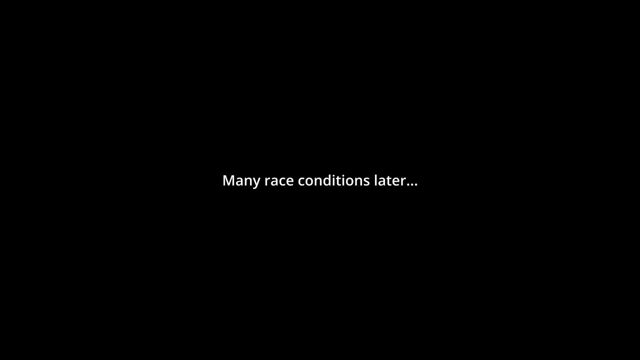 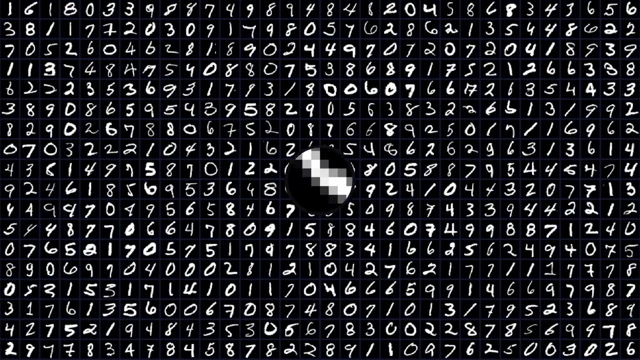 which I might actually quickly do behind the scenes. Okay, let's move on from the fruit at last and challenge our network to this class. Let's look at this classic handwritten digits dataset. We have 70,000 images on our hands here, all labeled with the correct answer, and each. 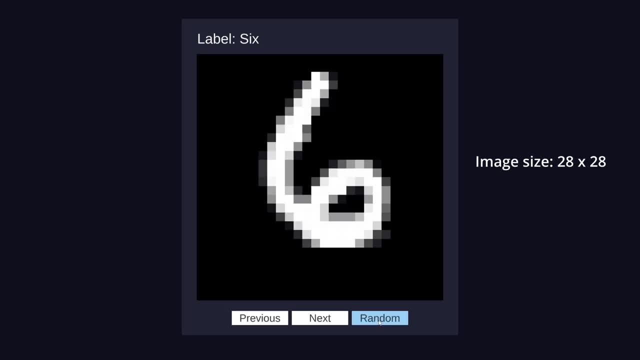 of these images is a miniscule: 28 by 28 pixels, so that's 784 values in total, each ranging from 0, meaning black, to 1,, meaning white. Now I've set up a simple interface for creating our neural network here, so I'll make one. 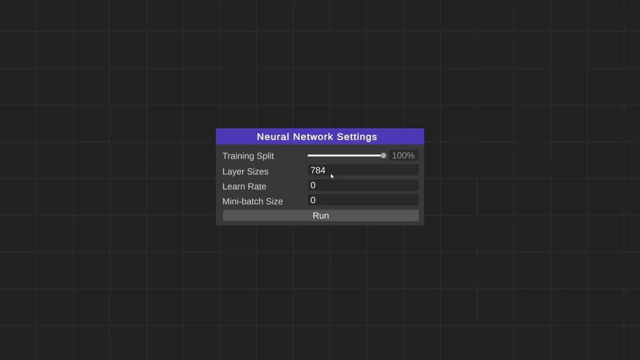 with 784 inputs to take in all those pixel values and 10 outputs for telling us which of the 10 digits it thinks it's looking at. Let's take a moment quickly to wrap our heads around this. So our fruit data had just two input values, meaning we could draw each data point in two. 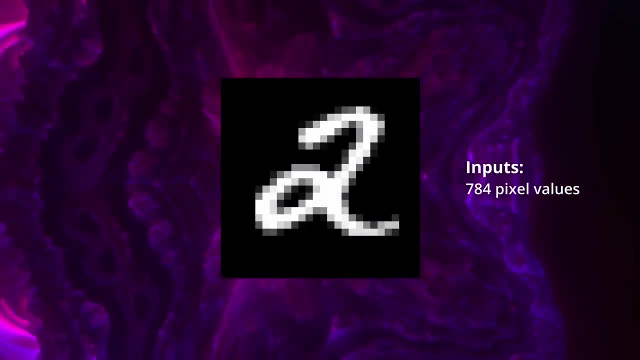 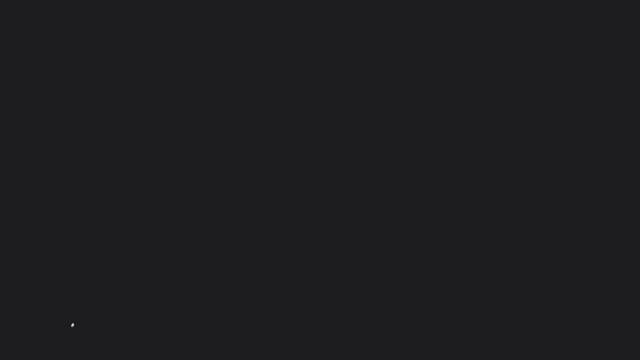 dimensional space. For the digits, though, we now have a 784-dimensional input space, which is a bit trickier to imagine, So let's just pretend it's in three dimensions instead, with each axis representing the brightness of a single pixel. Then perhaps images of a zero would tend to have values for those three. 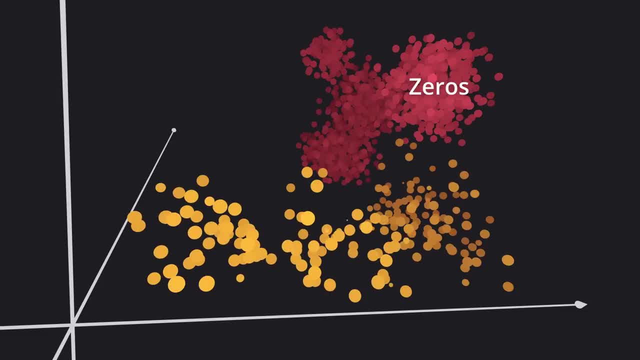 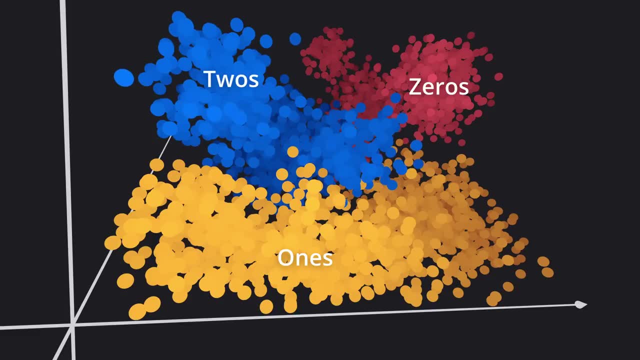 Values for those three pixels somewhere in this region, whereas for images of a one, maybe they'd be more in this region over here, And so on. I'm completely making this up, of course, but hopefully the idea makes sense that we can think of each of the images as points somewhere in 784-dimensional space. 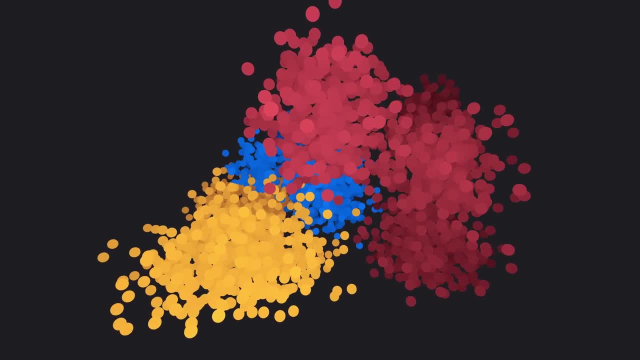 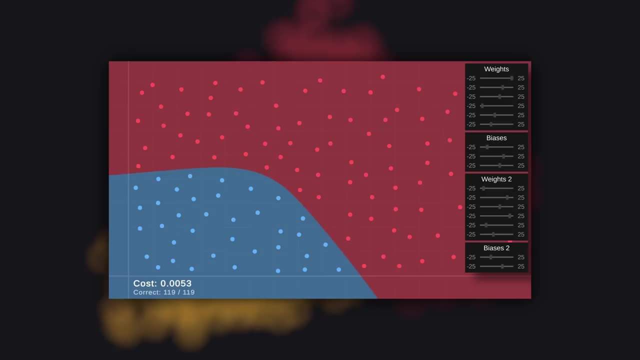 And our network just needs to figure out which regions of the space each digit tends to hang out in, just like it figured out which regions of two-dimensional space the safe and poisonous fruit tend to inhabit. Okay, let's get back to setting up our network, and I'll try giving this a learn. 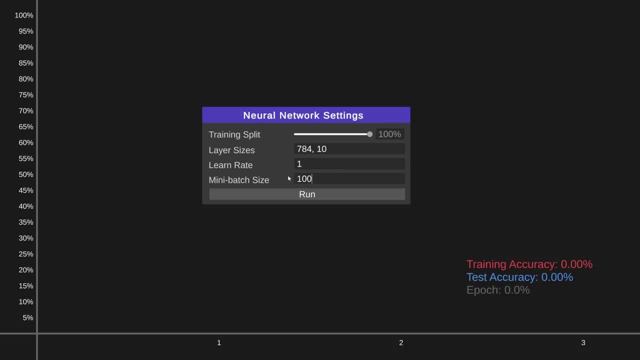 rate of 1, and a mini-batch size of maybe 100,, and that means it'll take us 700 batches to go through all the data we have, which is known as one epoch. We don't actually want to let the network train on all the data, though. instead we'll 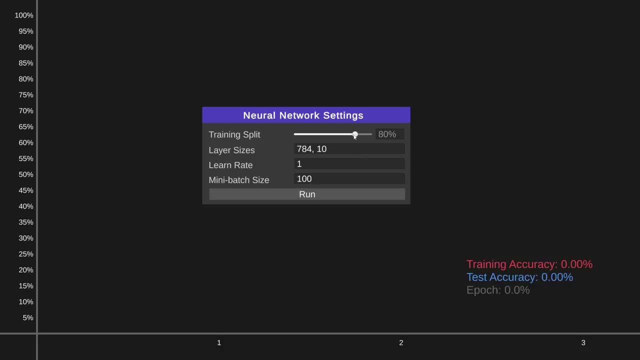 set some of it aside so that we can test how the network performs on data that it hasn't seen during its training, since that's what we really care about After training. for a few seconds it seems to have plateaued at around 90% accuracy. 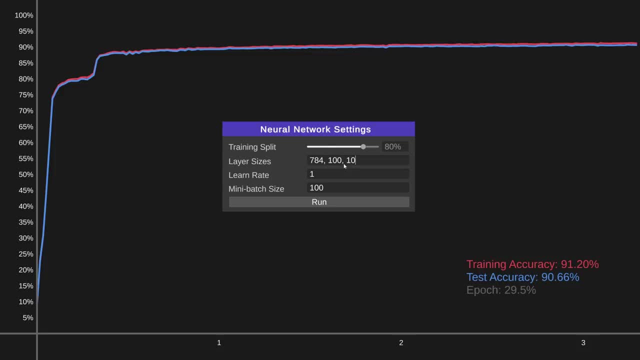 so let's try expanding the network with a hidden layer. I'll give it 100 nodes maybe, and we'll see if it can put all those extra connections to good use. It is taking a lot longer now to crunch the numbers, so I'll fast forward through the 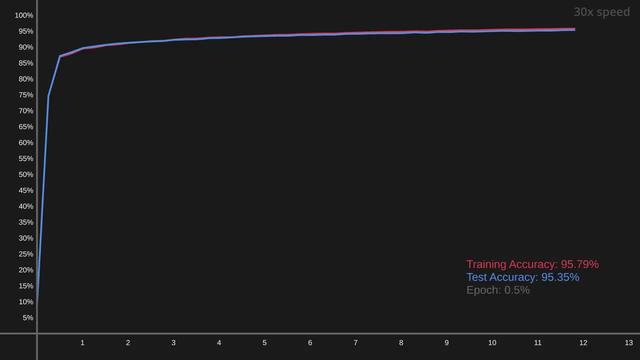 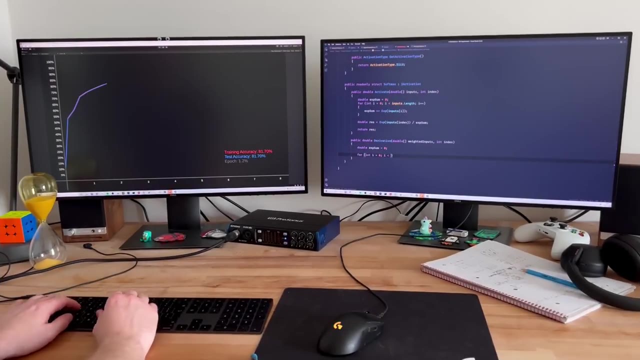 training, But in the end we've managed to get around 95% accuracy, which is not great, but not terrible either. To try and prove it a bit, I've been doing some research and implementing a few small things, like some different cost and activation functions, and also adding momentum to the 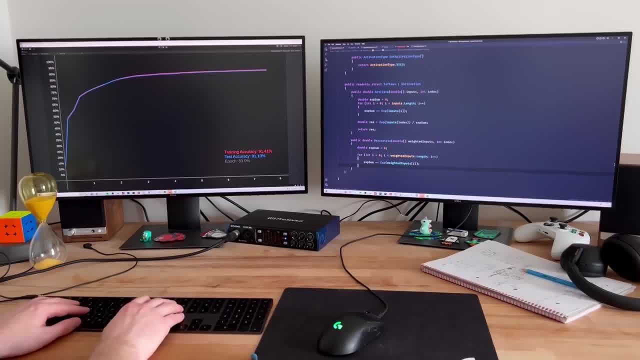 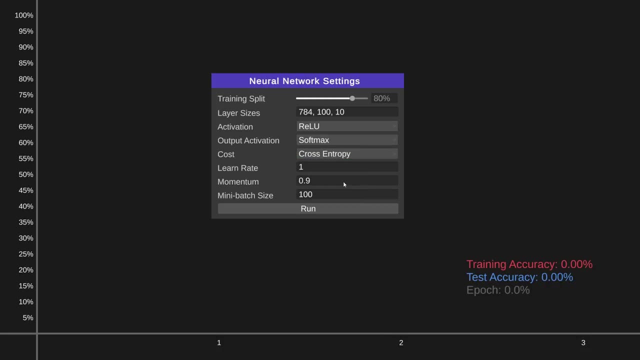 gradient descent algorithm which allows the weights and biases to essentially accelerate as they slide down those high dimensional slopes of the cost function. Hopefully all of this is going to help a little, so I'll set it up quickly and let's see how it goes. 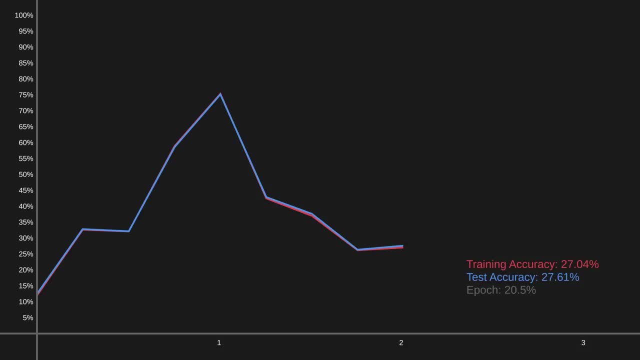 Well, that wasn't a resounding success, but before I go hunting for bugs, let's just try turning the learn rate down, because that could also be the issue. Okay, that's looking much better. We're getting around 97% of the test images correct, which I'm pretty happy with for now. 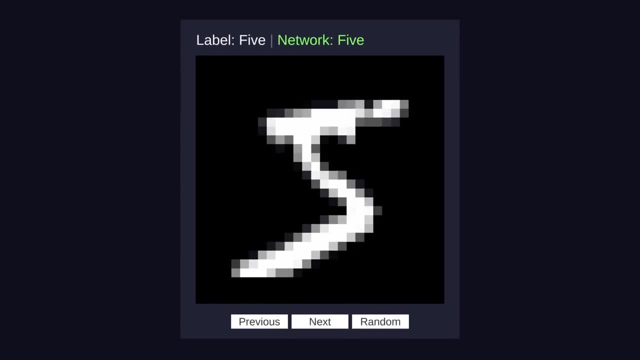 so let's take a closer look at some of these images. Here we have a 5, and up here, by the way, we can see what the network thinks it's looking at. So I'll flip through a few of these and we can see it's getting them all correct. so 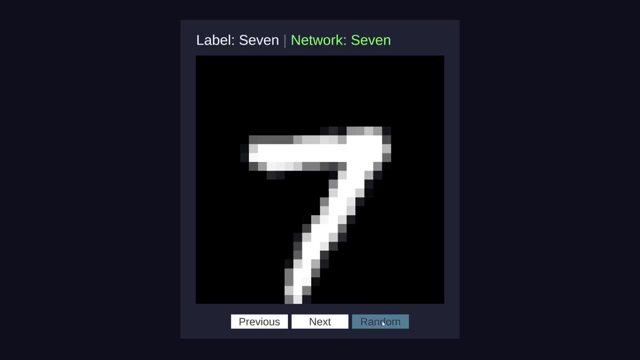 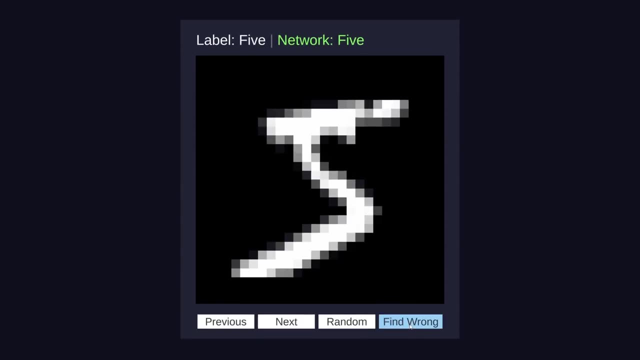 far. I'm more interested in seeing which ones. it's getting wrong, though, so I might need to add a way to find those. Okay, I've added a little button here, so let's try pressing it. Here's the first mistake. it thinks this is an 8,, but clearly it's a 0,, although I can. 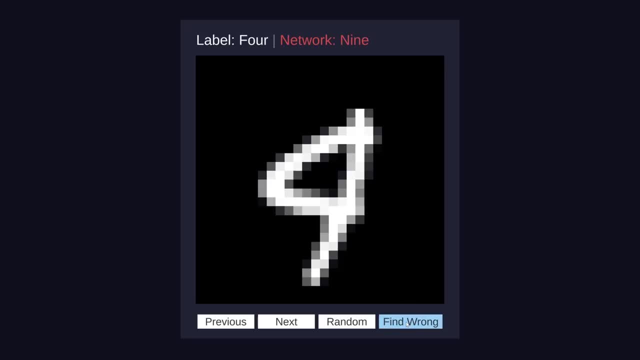 see where it's coming from. Next we have a 4,, apparently, And I think we can also see that it's a 4.. We can all forgive it for thinking that's a 9.. After that we have a 3,, which it thinks is a 7,, and I can half sympathise. it's maybe. 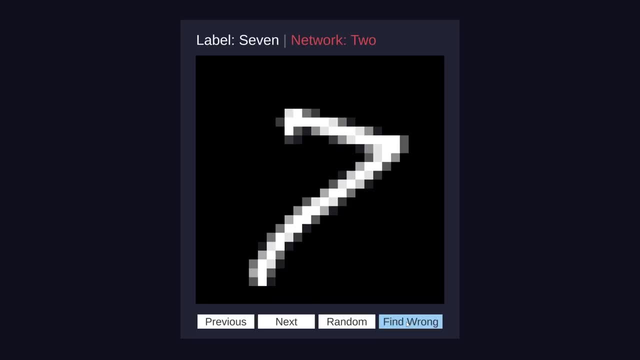 a bit unclear. Alright, let's look at one more. this time we have a 7, which it thinks is a 2 for some reason. So some of its mistakes are kind of understandable, but it's also clearly making some very blatant. 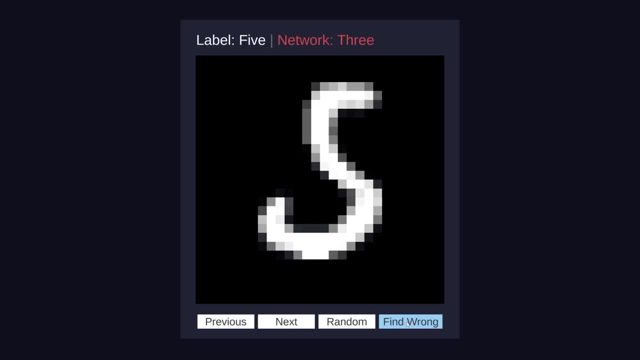 errors as well. We might be able to get a better idea of its shortcomings if we're able to draw our own digits. So I've been working on a super simple little drawing list. I'm not sure if you can see it or not, but it's a 9.. 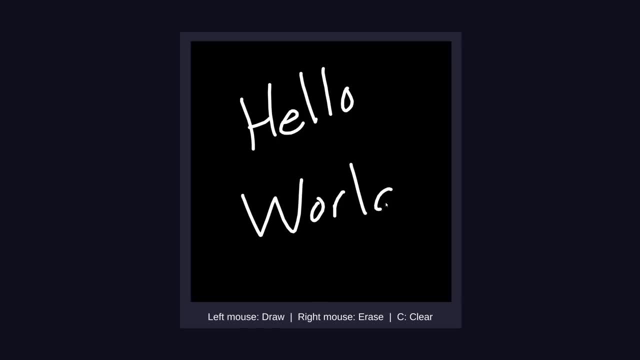 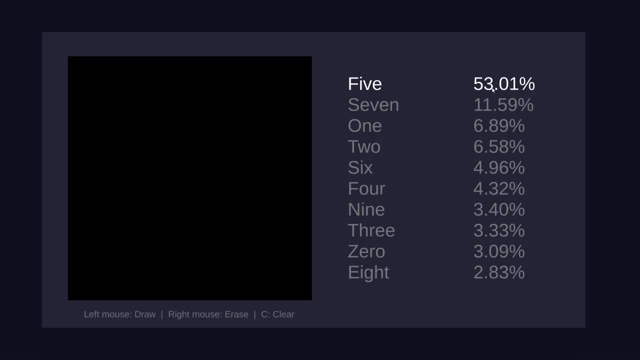 So let's try it out. I've got a drawing program over here which I'll hook up to the neural network and let's try it out. Starting off, it thinks this blank canvas is a 5, with a confidence of 53%, and we can. 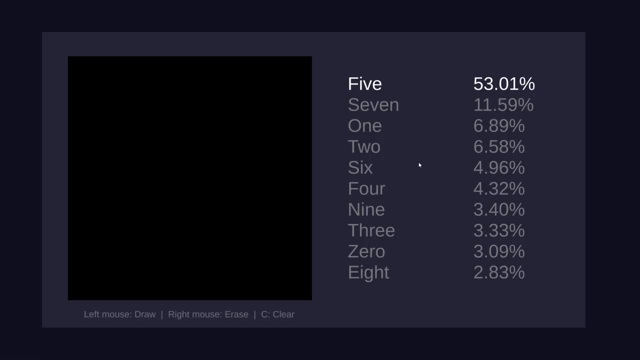 see the rankings of all the other digits below that. So let me start by drawing a 1, and it's managed to get that correct, so I'll try changing it a little bit. and all of a sudden it's saying that it's actually a 3.. 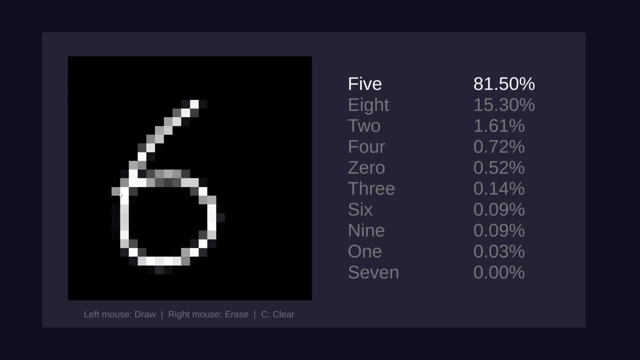 That's a bit concerning. Well, let me try drawing. maybe a 6.. No, it thinks that's a 5.. Okay, how about an 8?? That looks like a 3, apparently, So that's a bit strange. it's very good at recognising images from the dataset, but when 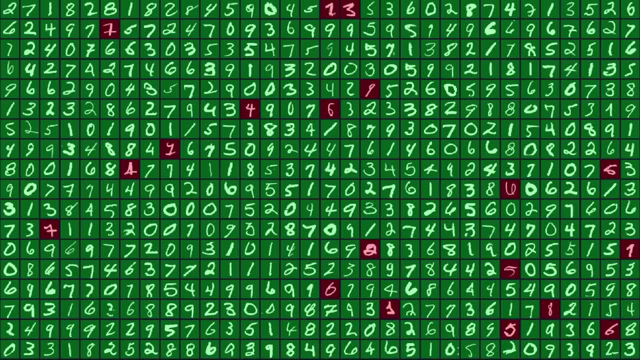 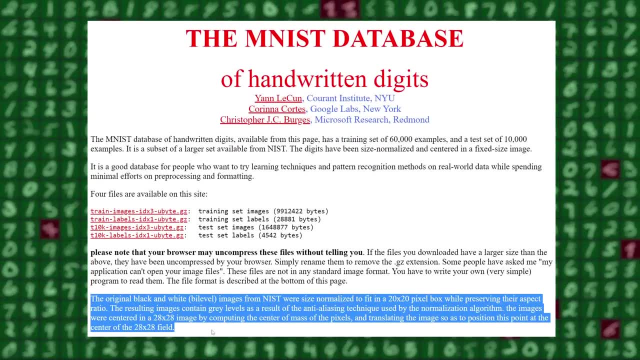 I draw my own digits. it's like it's never seen a number before. I think what's going on is that all the digits in the dataset have been sized and centred in a specific way, and I guess the network has come to rely on that being the case. 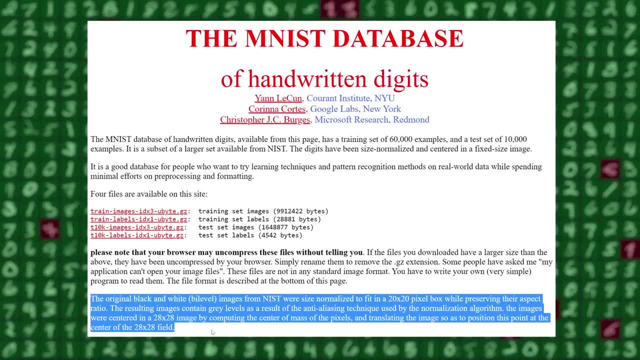 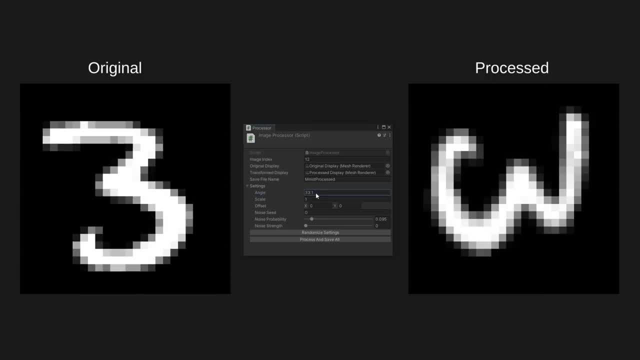 So we could obviously try processing our own images in the same way, but I'm actually more interested in trying sort of the opposite approach. I have written some code that can rotate. well, that was more sensitive than I was expecting. it can rotate the digits in the dataset as well as scale them, move them around, and 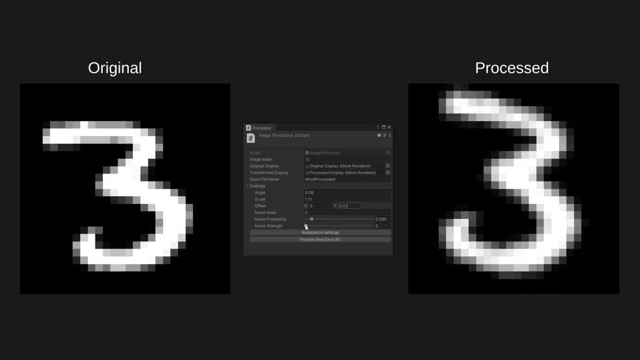 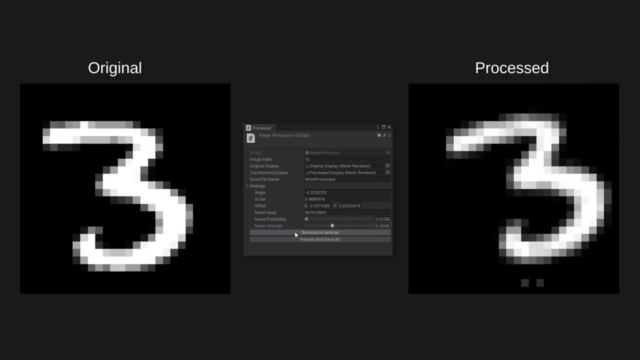 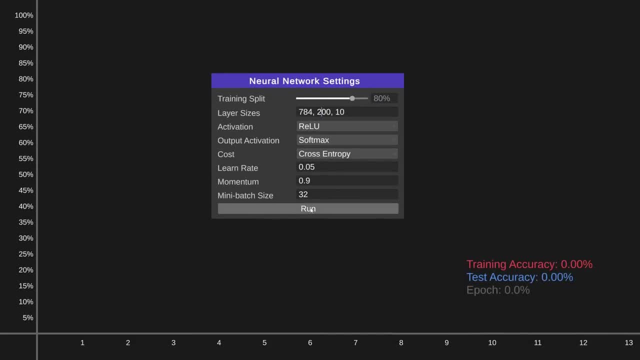 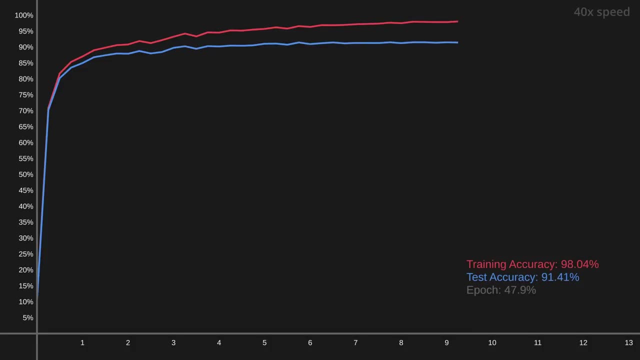 So let's do that, So let's do that, So let's do that, And it's definitely struggling a lot more. now we can see it's just scraping past 90% on the test accuracy. It is over 99% accuracy on the training data, though, which means that it's learning lots. 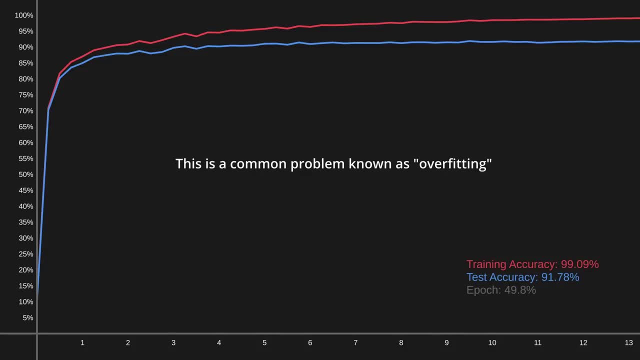 of overly specific patterns, essentially memorizing the answers, which is not very helpful. So I've been experimenting with various techniques for reducing this, and what I'm trying at the moment is simply adding some random noise to all the objects the network's inputs, with the hope that, if it can't rely on specific patterns, remaining 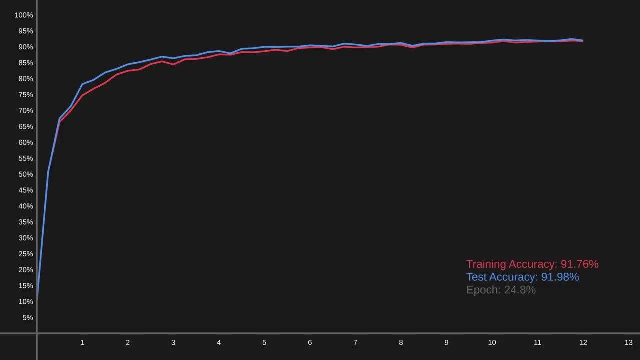 exactly the same. it will end up learning more general patterns instead. From the results we can see that it's somewhat worked. The test accuracy is up about 1.5%, which might not be wildly exciting, but it's nothing to sneeze at either. 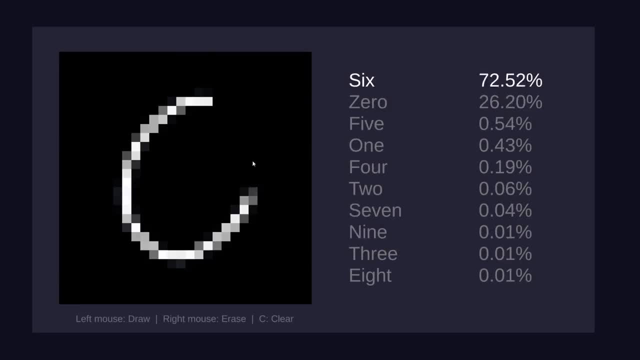 So let's go see if this new network can decipher my handwritten digits a bit better. So 0,, 1, and 2 all correct so far, so it's already looking a lot more encouraging than last time. 5 is correct as well, and 6, and 7, and 8,. this is exciting commentary, I know. 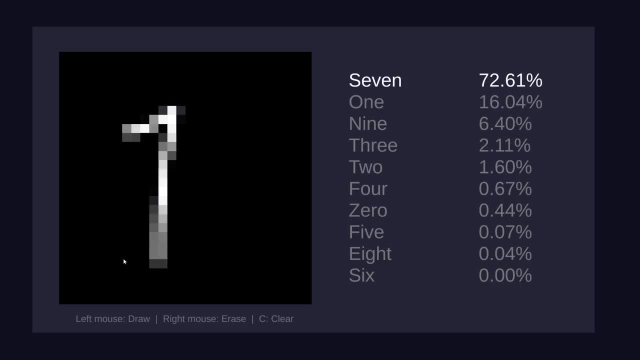 and there's all 10 digits correct on this first run through at least. I'll give it another try to make sure we didn't just get completely lucky the first time and it has managed to get all of them correct again. I'll keep testing it for a while though. 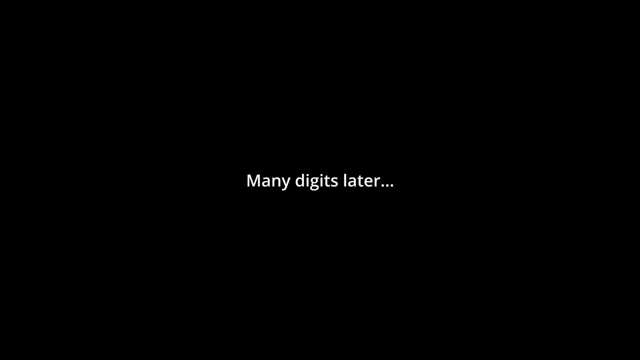 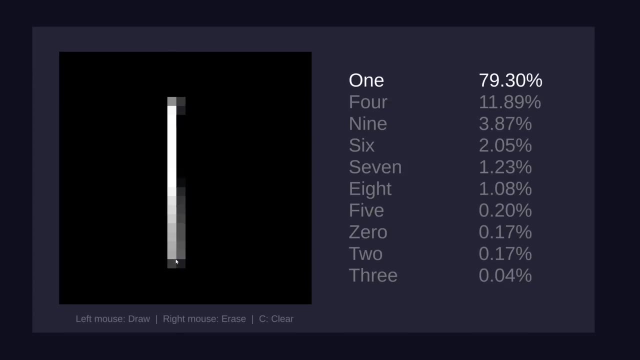 and let you know how it goes. Okay. so it definitely does have some big weaknesses. For example, if I draw a 1 as just a straight line, it's very happy, But if I add a little stroke at the top here, 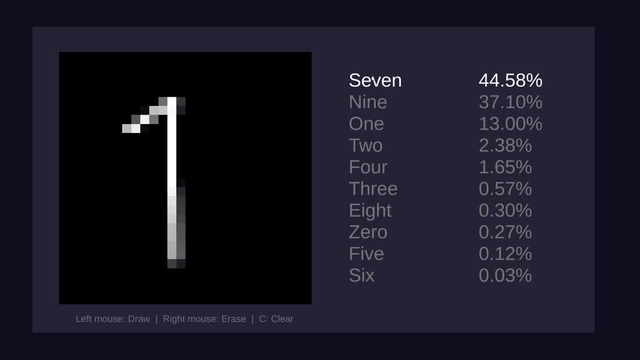 it can quite quickly start thinking it's a 7. instead. We can steer the network back on course by adding a little line to the base here. now it thinks it's a 1 again. But if that line extends just a tiny bit too far, the network will suddenly think it's looking. 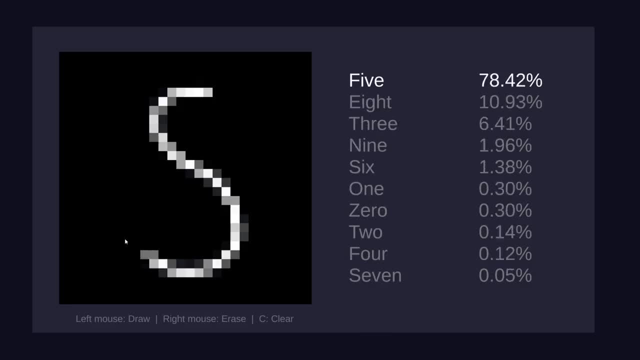 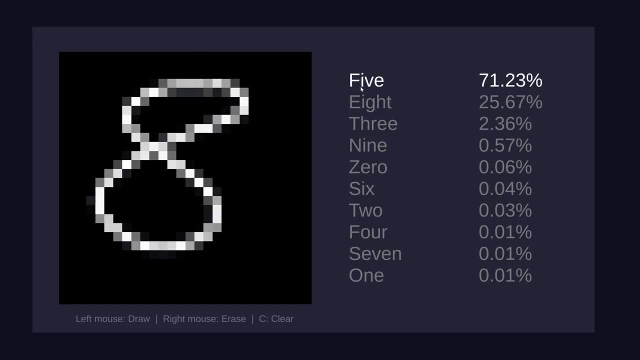 at a 2. instead, It seems to be a bit more reliable with other digits, like 8s, for example, But even there it doesn't take too many attempts to run into a case that bamboozles the network. Despite its flaws, though, I'm happy for now that it at least seems to work most of the time. 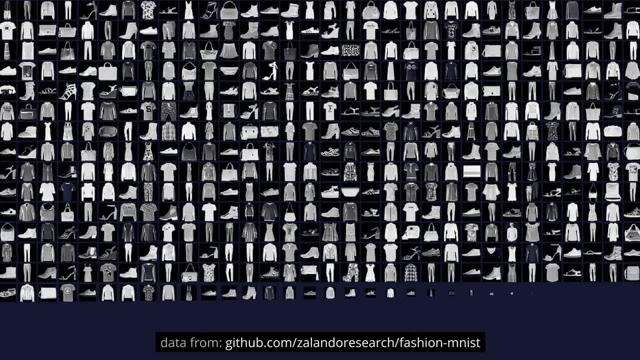 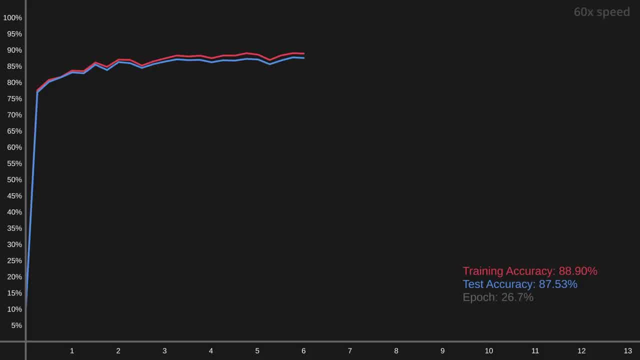 Just for fun, let's quickly try training our network on this fashion dataset, which was created as a more challenging drop-in replacement for the digits. So after a few minutes of training it's reached around 89% test accuracy. I'll give it another try, though, and it seems to be a bit more reliable with other digits. 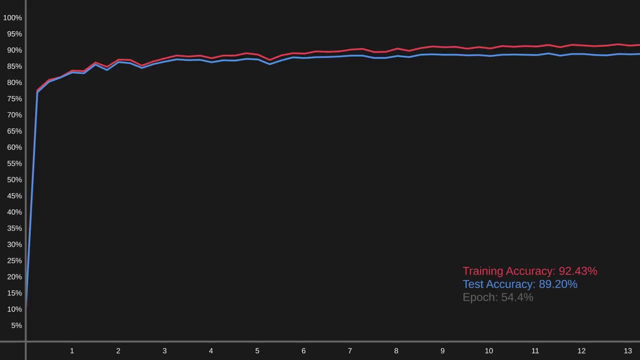 like 8s, for example, But even there it doesn't take too many attempts to run into a case that says 83%, which is not amazing, but it is apparently better than human performance at 83%, which I thought was interesting. 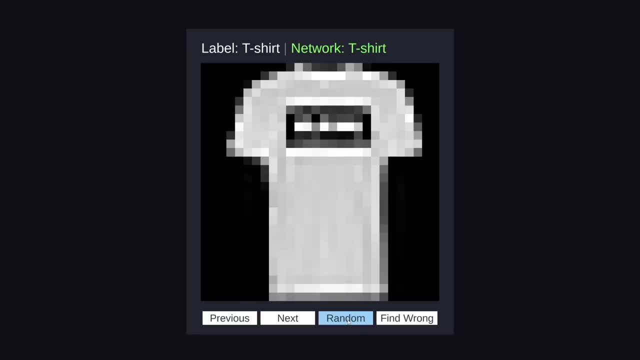 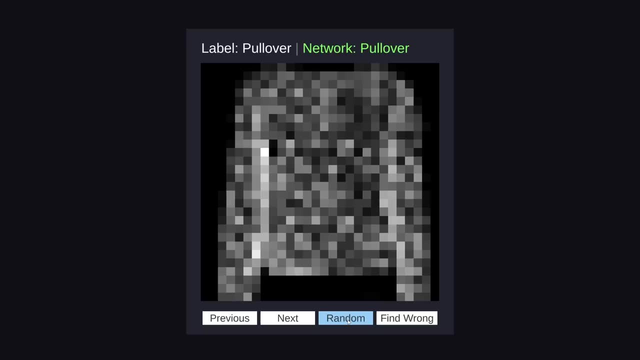 Anyway, let's take a brief look at some of these. So here's a shirt, excuse me, a t-shirt, which it's getting correct. Then here's a shirt and a pullover, also both correct. Let's see how long it can keep this streak going. So we then have a sneaker, a dress. 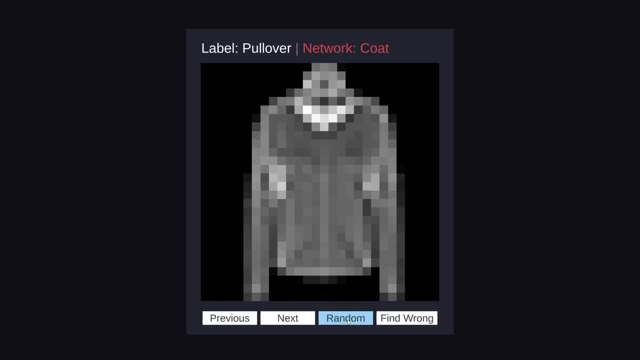 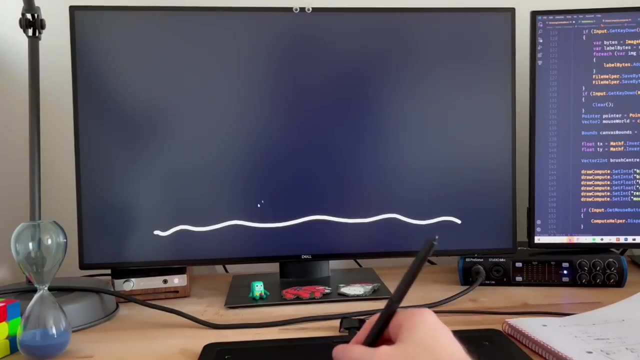 and another dress, Then a coat and finally it's been caught out by what it thought was another coat but is actually a pullover. Okay, I thought that was interesting to try quickly. But let's move on to our goal from the beginning of recognizing various doodles. 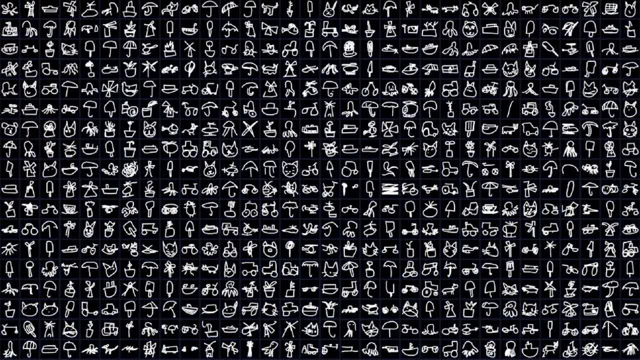 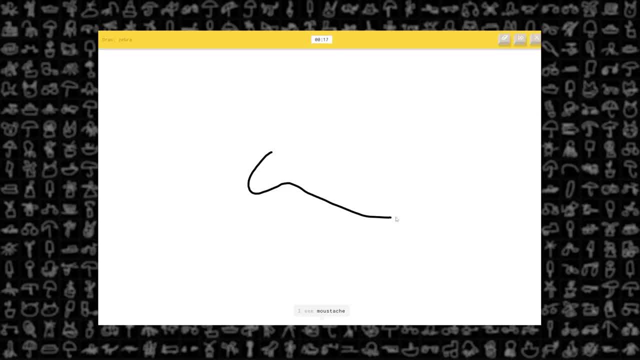 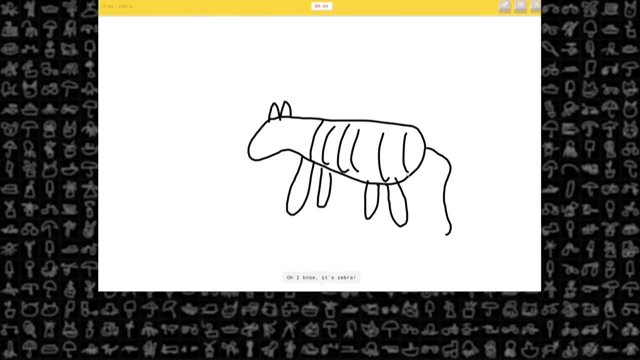 So I've downloaded a doodle data set drawn by people from all around the world, which comes from the very cool quick draw project. I see mustache or peanut or swimming pool or cannon. I see pillow or horse or tiger. Oh, I know, it's zebra. 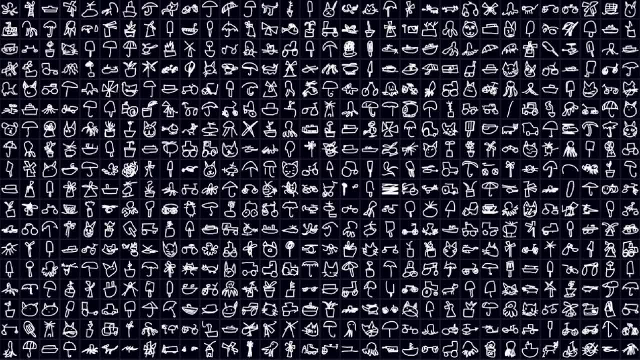 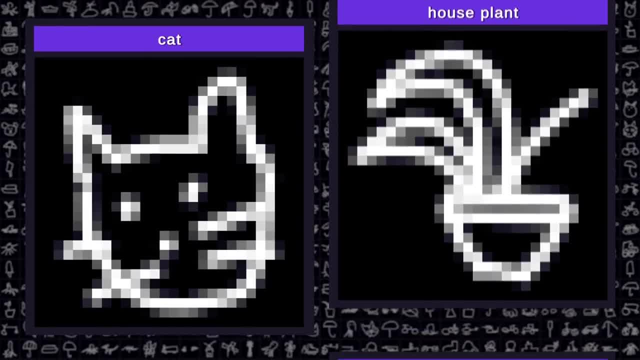 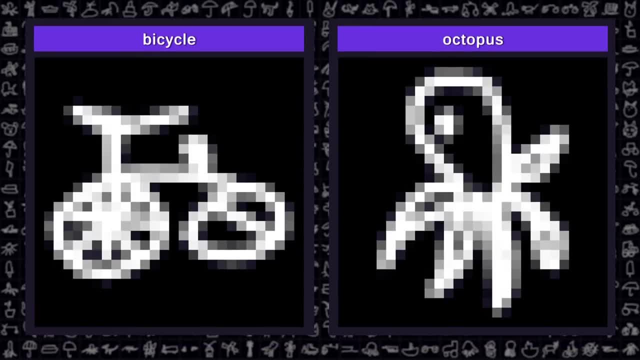 To keep things simple for us, today, I've picked just 10 categories from the 345 that exist in total, So our full lineup is helicopters, houseplants, cats, ships, cruise ships, windmills, popsicles, tractors, umbrellas, bicycles and octopuses. 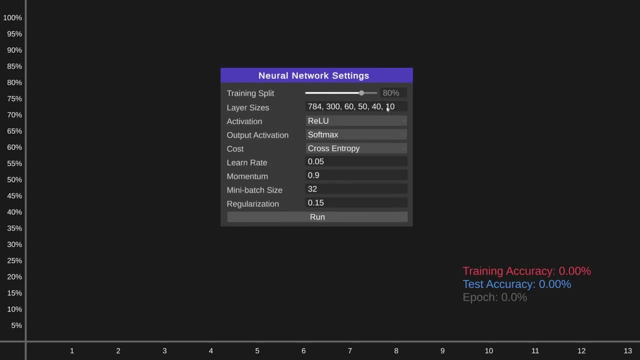 I've increased the size of the network again and also added some extra hidden layers, not for any deep reason. I've just been messing around with different settings out of curiosity, So I'll leave this to train for a few minutes. and, by the way, I did make the same random. 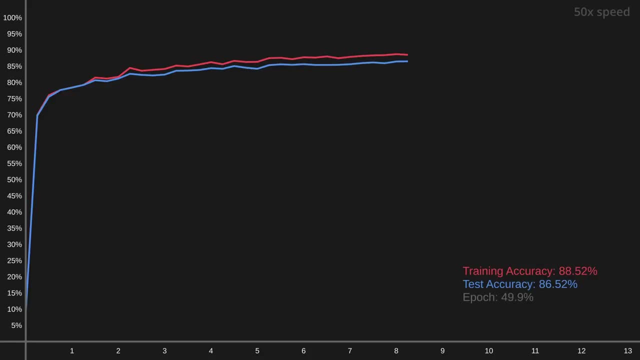 transformations to the doodles, as we did with the digits, since that seemed to be very helpful. Alright, we've ended up with about 87% accuracy here. but for the true test, let's see if it can recognise some doodles of our own. 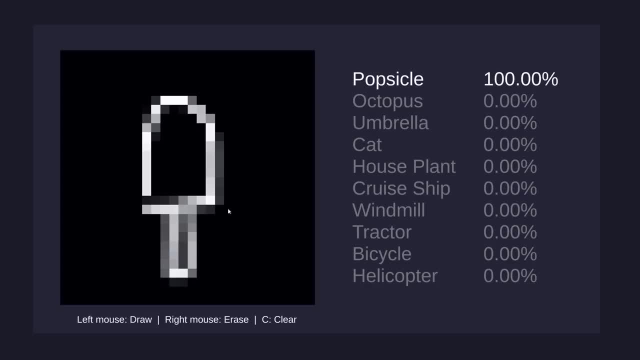 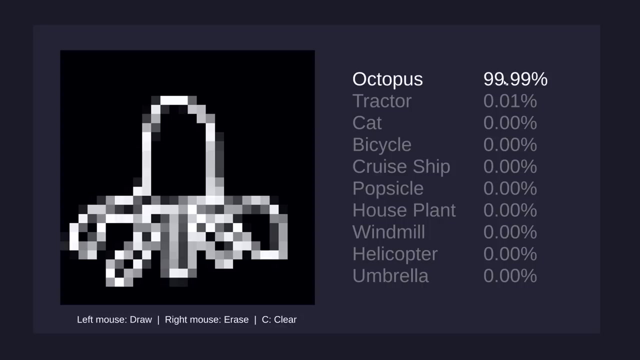 I'll begin with a popsicle- 100% popsicle. it says very nice. I wonder if I could give this some squiggly legs and turn it into an octopus. Okay, it's very confident about this being an octopus. now, with just a sliver of doubt. 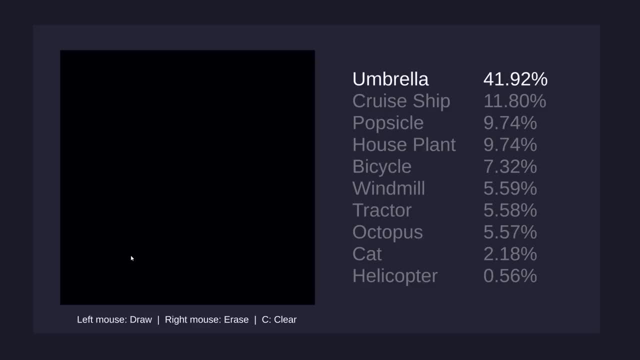 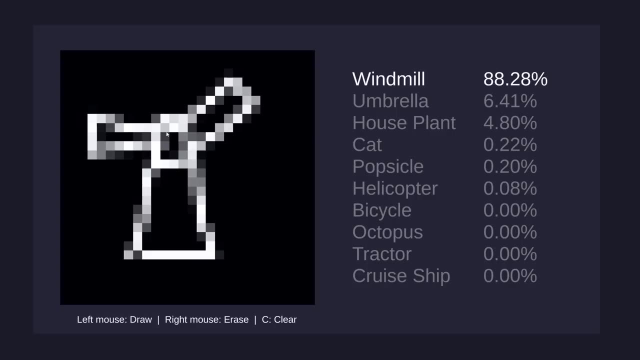 that it may in fact be a tractor. Let's try something else. So at the moment it thinks I'm drawing either another popsicle or an umbrella, although now it's just realised that I'm actually trying to draw a windmill. I see that houseplant is its second prediction. so let's try planting the windmill in a little. 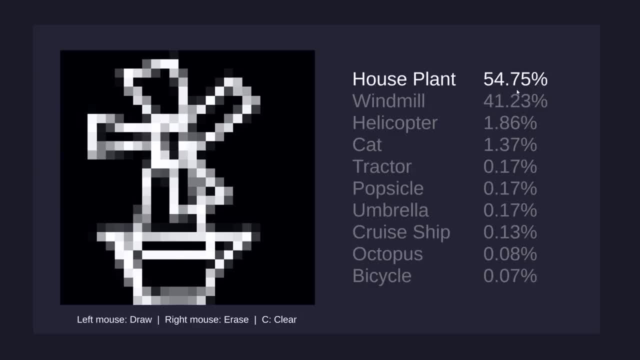 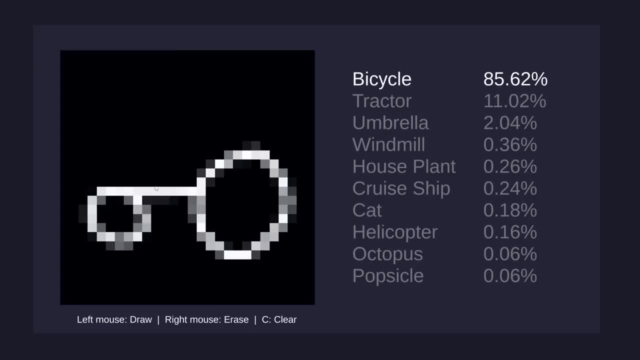 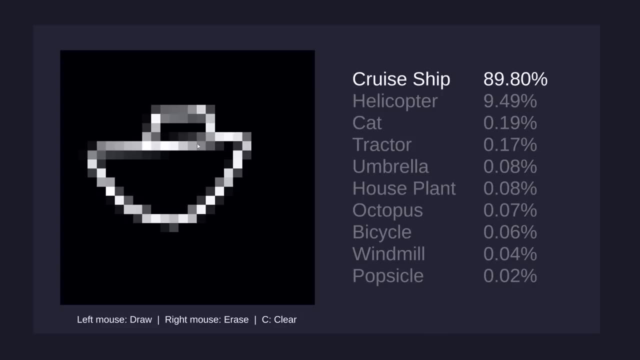 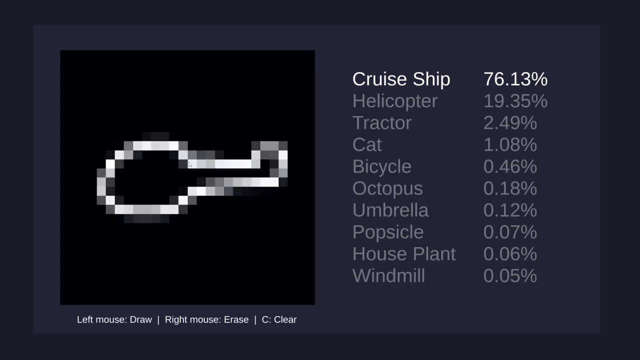 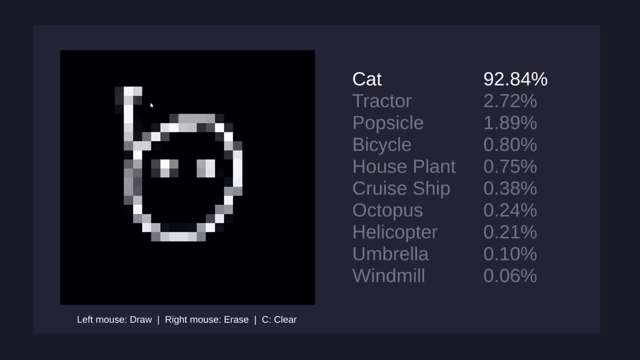 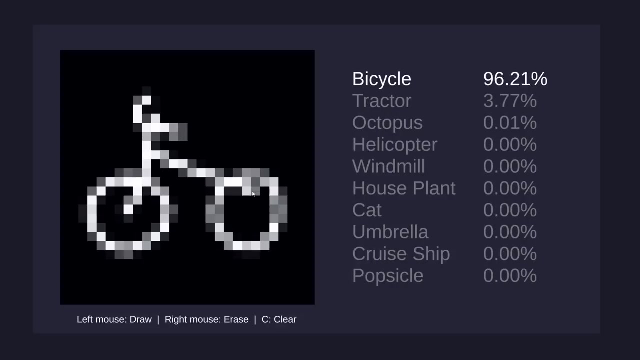 pot And it is saying that it's a houseplant now, although it's definitely a bit suspicious of it. Anyway, I'm just going to play around with this for a little while and see how it goes. Okay, so it's been working pretty well, I think, although, like with the digits earlier, it 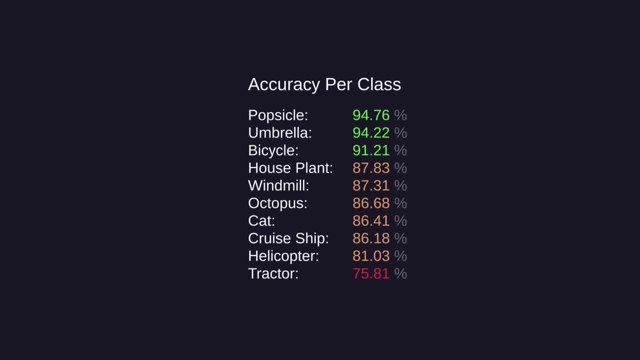 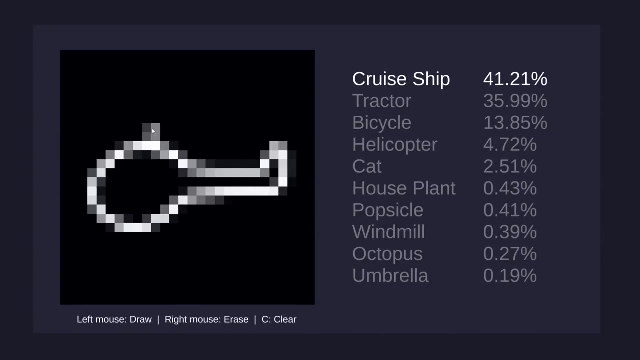 does still make some very obvious mistakes. I've printed out its accuracy on the individual categories here, and it looks like popsicles, umbrellas and bicycles are its specialty, whereas tractors are what really baffles it the most. For me, though, it seemed to struggle the most with helicopters. 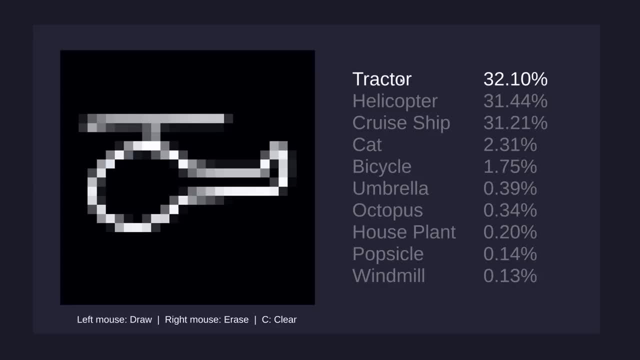 Here you can see. it's in a lot of doubt over whether this is a tractor, a helicopter or a cruise ship, And in cases like this it seems to be very sensitive to small changes. For example, if I add a random little line here now, it's an umbrella out of the blue. 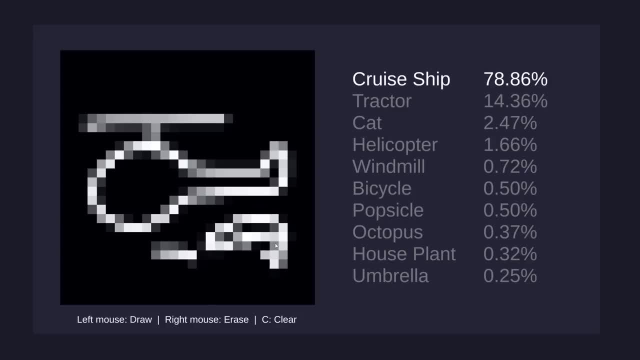 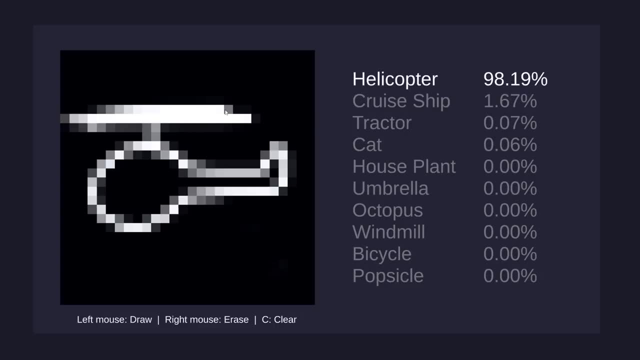 Now it's back to being a tractor and now it's a cruise ship. But if we can really convince the network that this is a helicopter- and it seems like just emphasizing the rotor here usually does the trick- then it's not nearly as indecisive. 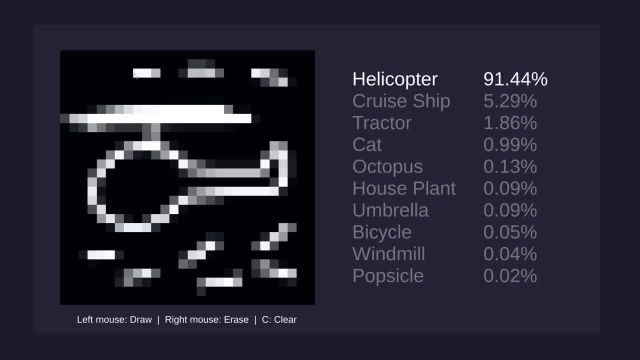 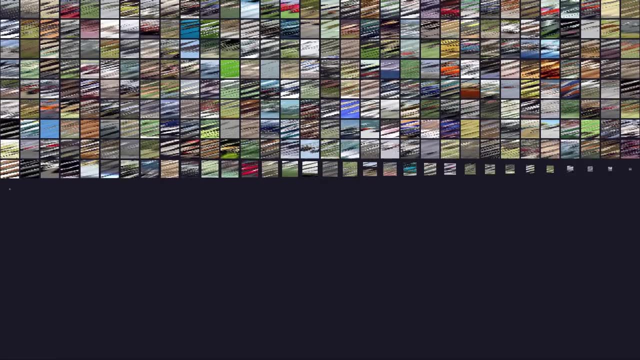 So clearly it's a very long way from perfect, but overall it does actually work reasonably well, I think, So I'm happy with it. for now, To end things off today, let's try giving our network by far its greatest challenge yet, Which is not supposed to look like this. 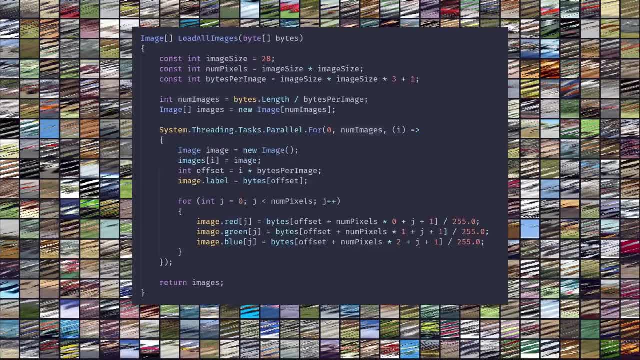 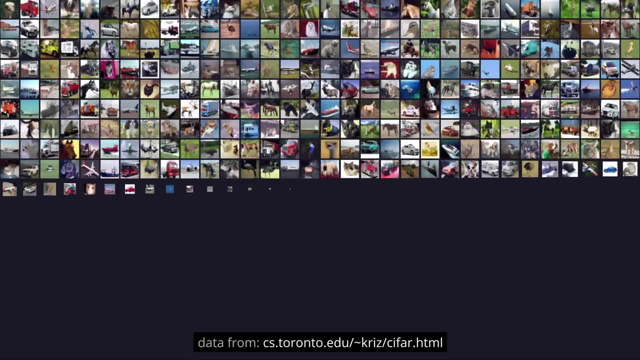 It's not supposed to look like this. What's going on? Okay, I forgot that these images are a whopping 32 pixels wide. now let's try that again. So these images are a bit bigger than before and in color, which means we have 3072 inputs. 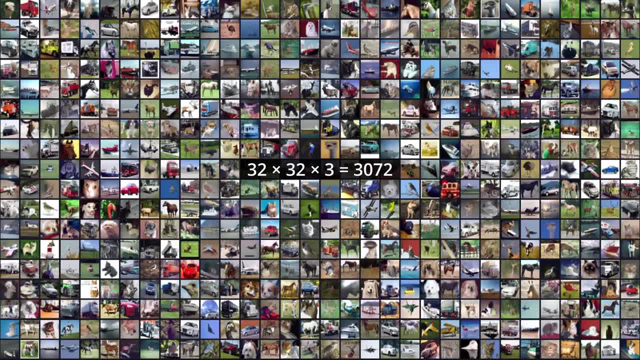 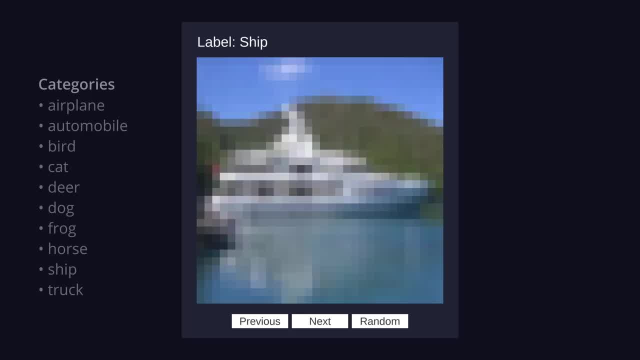 instead of just 784.. And let's take a closer look at some of them. Right away, we can see that this is going to be trickier for the network, because the object or creature it needs to recognize hasn't been nicely cut out for it, or anything there's. 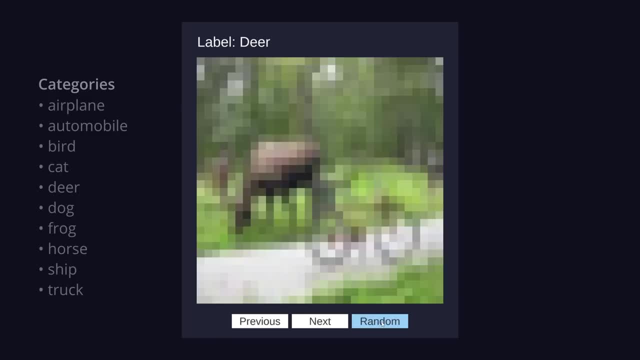 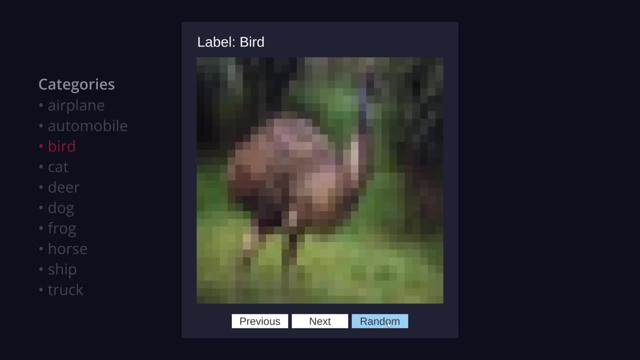 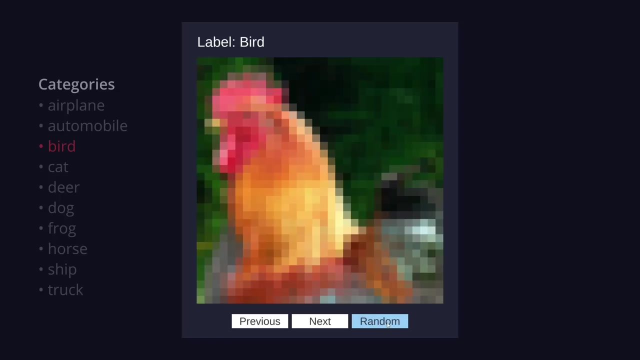 the whole environment around it, And we can also see how much variety there is even just among pictures of birds. for example, We've got little birds on branches, big birds jogging around, birds, swimming birds, flying birds staring straight into your soul. you name it. 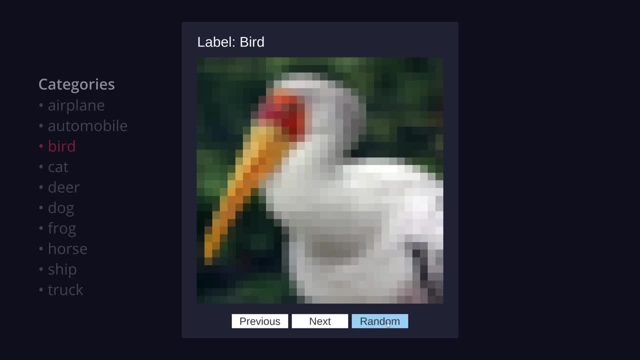 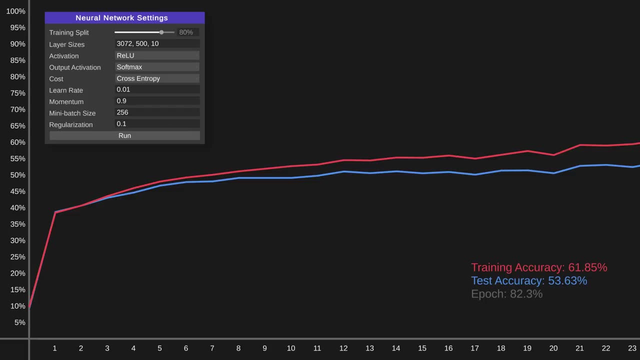 So, with all this complexity in mind, let's see how our simple network fares in its training. Not terribly well is, unfortunately, the answer. it ended up with an accuracy of about 53%. but let's take a look anyway. Let's see. 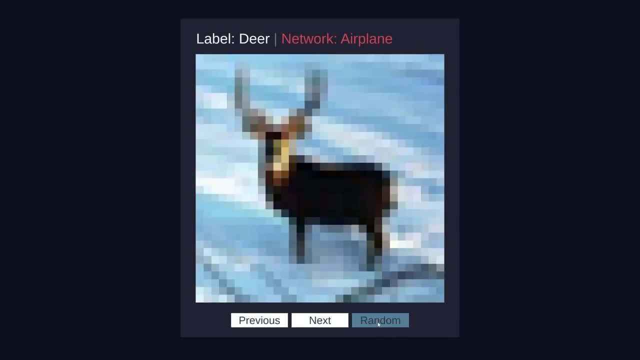 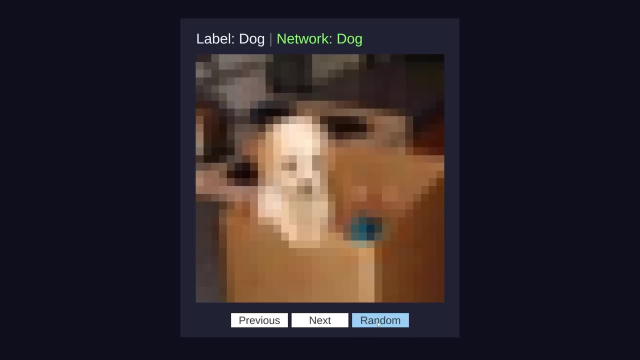 To begin with, we have a deer, which it thinks is an airplane, and a dog, which it thinks is a horse. so not off to a good start. It has recognized this bird, though, as well as this little dog in a box. but then this: 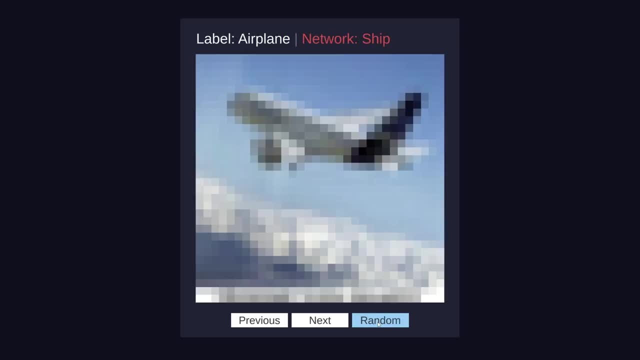 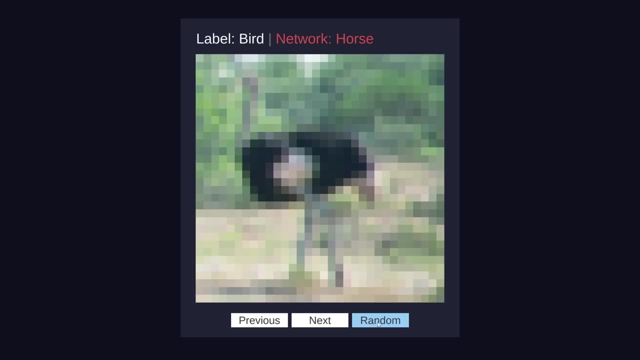 aeroplane. it's unfortunately misidentified as a ship. Let's see what's next. so this time ship was correct. and then we have an automobile and a truck, both correct, but that's certainly not a horse. So, as expected, it's getting around half of them, correct. 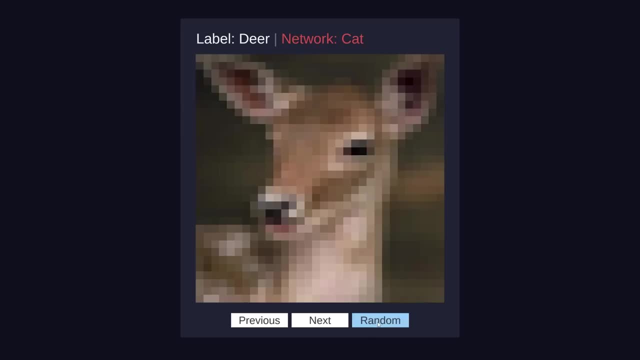 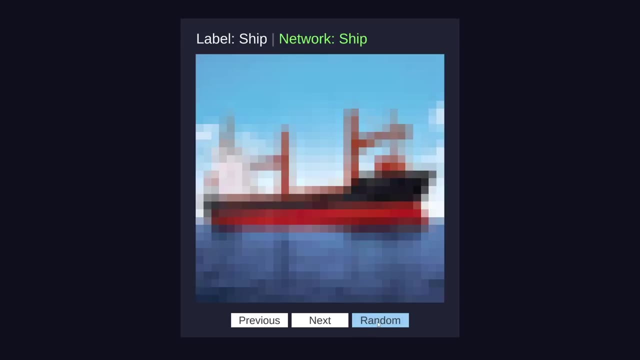 Which is of course a lot better than random, but still a pretty underwhelming result. I'm sure we could coax a bit more accuracy out of our simple network with some tweaks here and there, but if we wanted to really be able to take on this challenge, it's.